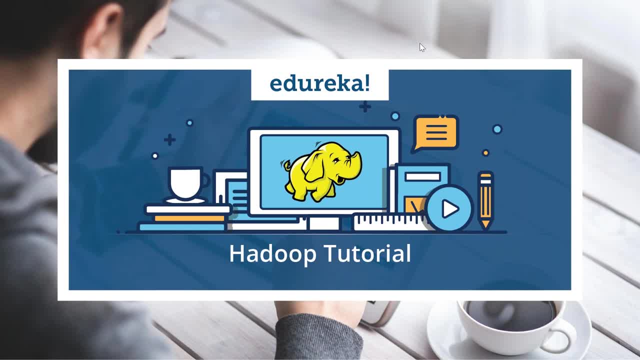 From this session. Okay, so, guys, can you quickly give me the acknowledgement in the chart window if you are already familiar with Hadoop or Spark? And also, guys, we'll try to make this session as interactive as possible, So it's like all of you would be on mute by default. So if you get any, 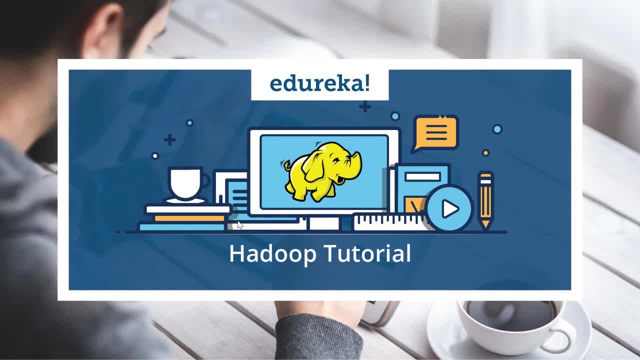 questions or any issues. you can always ping me in the chat window. Okay, many of you, says Kunal Shubham Kushal. all are saying that, yes, they have used Hadoop. Okay, Sudesh says very minimum experience on big data, but I've worked in data warehousing project. I'm familiar with Hadoop, but 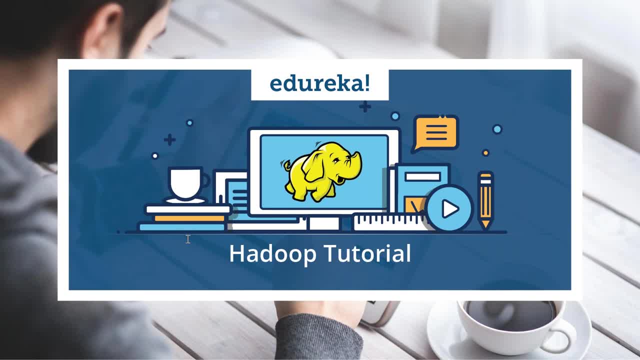 would like to know about the current trends and Spark. Okay Shubham says just basic understanding with Hadoop and Spark Java developer for four years. Okay Kumar says I'm not even in this field trying to get a big picture of how it works. So I'm not even in this field trying to get a big picture. 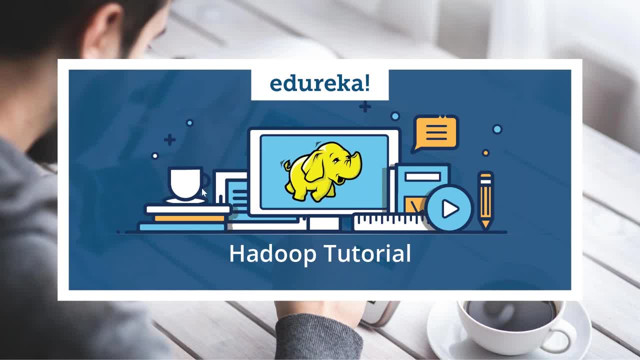 of how it works. Okay. Shubham says I'm not even in this field trying to get a big picture of how it works. Okay. Rakesh says: null experience in big data. Okay, how about others? Okay, just no experience. beginner: 12 years of total experience, six years machine learning: have a bit of familiarity with. 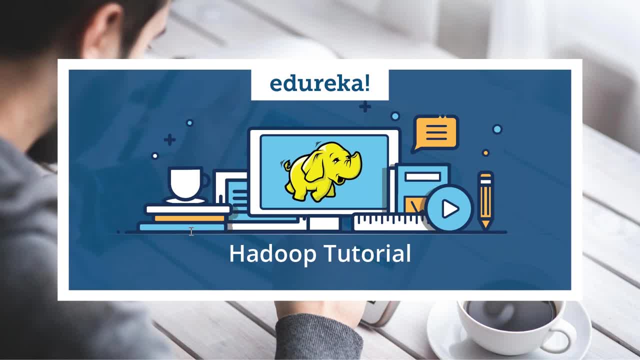 Hadoop and Spark Wrote some Spark jobs to clean clickstream data. Okay, no experience in Hadoop, Okay, perfect guys. So, guys, it's like now we have. I know the diversity of this class. It's like many of you are already familiar with the term big data and Hadoop and a few of you are completely. 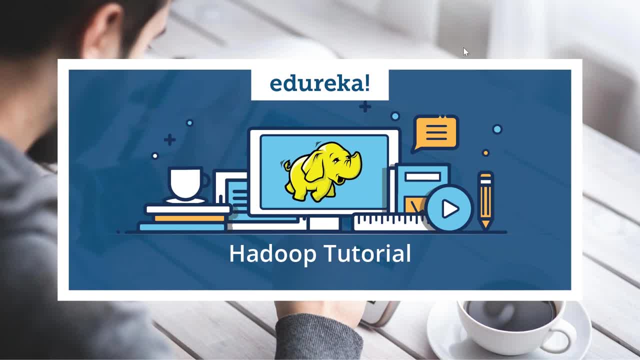 new to this domain. So, guys, not to worry, in today's session we will understand what is Hadoop, what is Spark, what is the difference and how Hadoop and Spark can work together. So we do have Kewal Kewal. 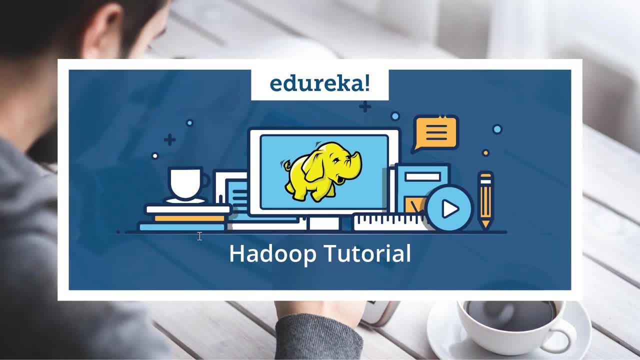 says: system admin, DevOps- 10 years of experience, real Hadoop, Spark, little experience with Kafka and Python. Okay, okay, perfect, guys. Okay so, guys, let's, let's get started. But yeah, before we get started, one thing: we'll try to make this session as interactive as possible. Whenever you get any questions or any. 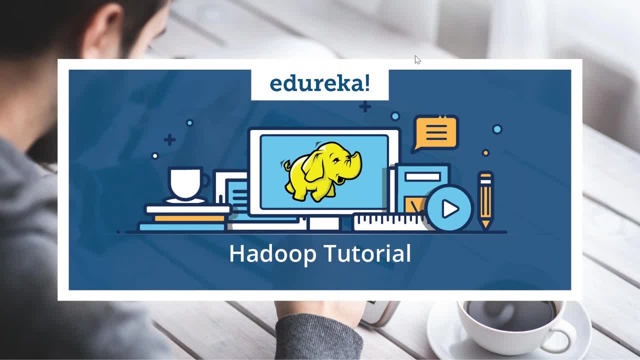 issues, you can ping me in the chat window. By default, all of you would be on mute. Okay, so, guys, we do have Rekha as well. So Rekha says Java developer, just started with big data and almost a pressure to Hadoop and Spark. Okay, so, those who are completely new to Hadoop and Spark, 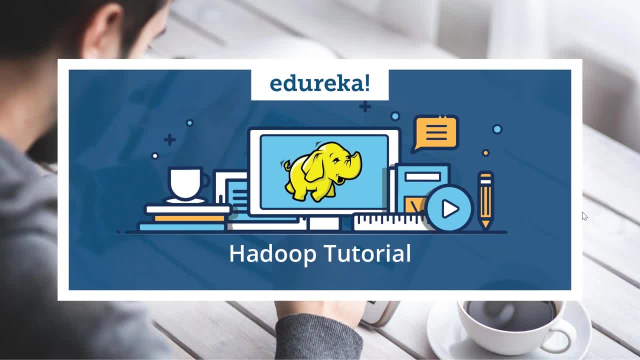 guys, not to worry, in today's session we will discuss what is big data, Hadoop and Spark. Okay, so one thing, guys: this session is just an introductory session. We will not be going into the details of Hadoop and Spark. This session is just to give you the overview of Hadoop and Spark. Okay, and also, if 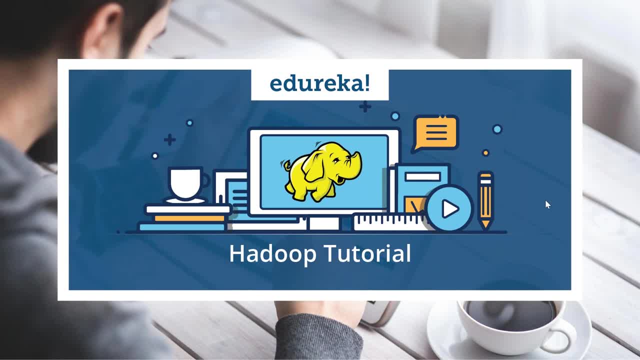 you want to get a, if you want to get expertise on Hadoop and Spark. So Edureka is providing courses on both Hadoop and Spark and this session- it's objective of this session is give you the overview of Hadoop and Spark and not to have a detailed discussion. Okay, so it's like when it comes to the detailed, 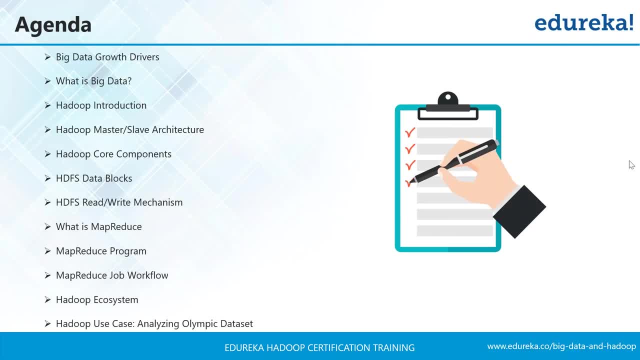 discussion of Hadoop. even if you give me 200 or 300 hours, then also I won't be able to complete it, and same is the case with Spark. Okay, but yeah, I'll try to all. I'll try to answer all the questions which you will have. Okay, guys. 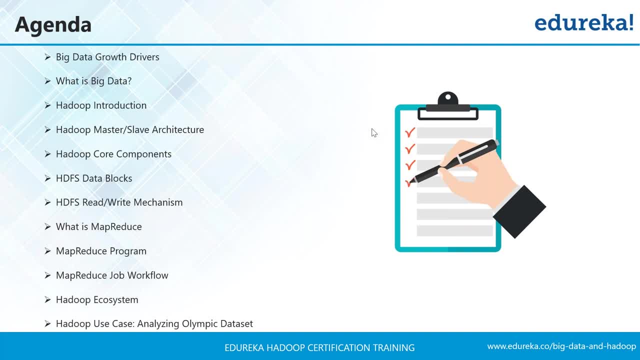 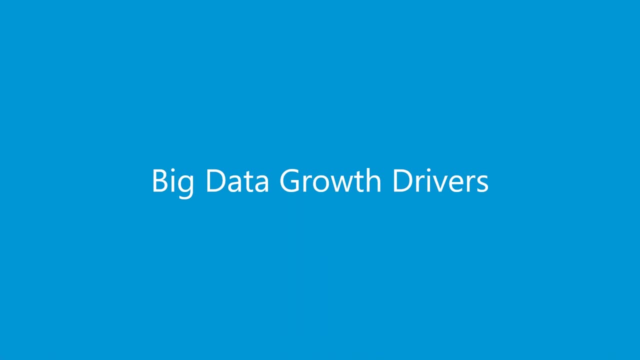 so let's get started. So this will be the agenda. So in this agenda you just see the topics related to Hadoop, but, not to worry, we will be discussing Spark as well. Okay, agenda of this session is to discuss both Hadoop and Spark so that you get the overview of both the components. Okay, so it's like: 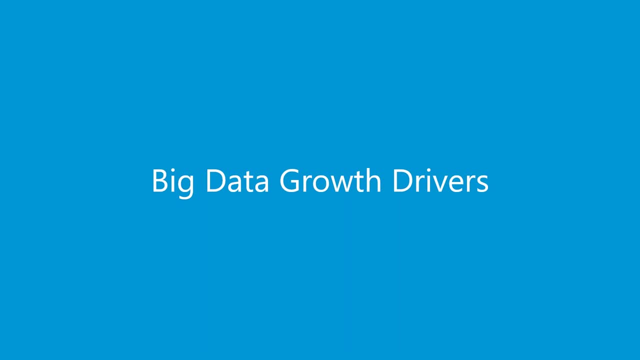 initially, in the beginning, we'll talk about what is like big data, What is Hadoop, What are the components of Hadoop, or Hadoop and Spark. So let's get started. So let's get started. So this will be about how it works, What is the architecture, and then we'll move on to the discussion of Spark. 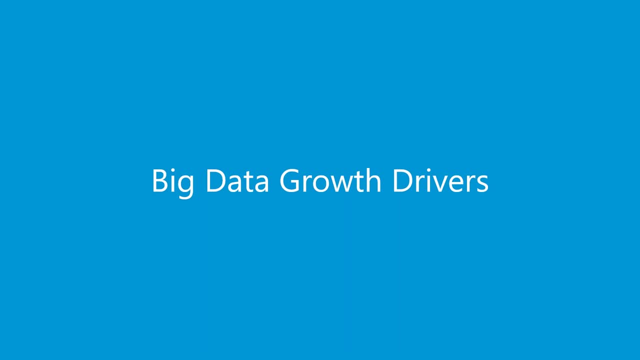 Okay. so, guys, big data, growth drivers. So, first of all, let's understand what is big data. So, guys, it's like it's a very any. if you ask me in general, like, what is big data, I would say that it's nothing, but it's a problem which industry is facing right now. So why am I making this statement where I'm 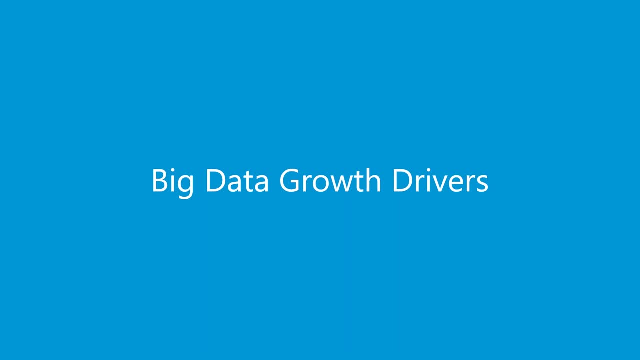 that it's nothing, but it's a problem which industry is facing right now. it's like if I talk about the scenario which was there in the, in the market or in the industry 20 to 25 years back, it's like we were not generating huge amount of. 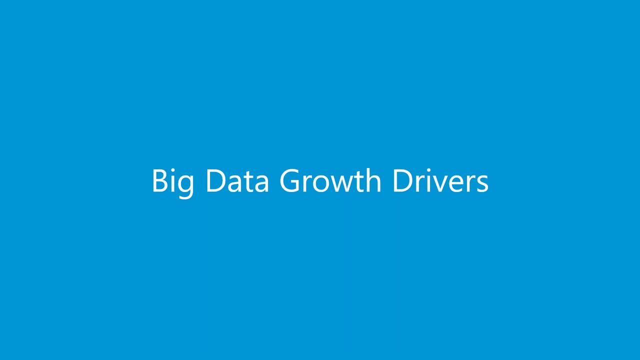 data, or we were not dealing with audio and video 20 to 25 years back as much as we are dealing today, right? so the tool or the technology or the framework which came into the market 20 to 25 years back is designed specifically to for small. 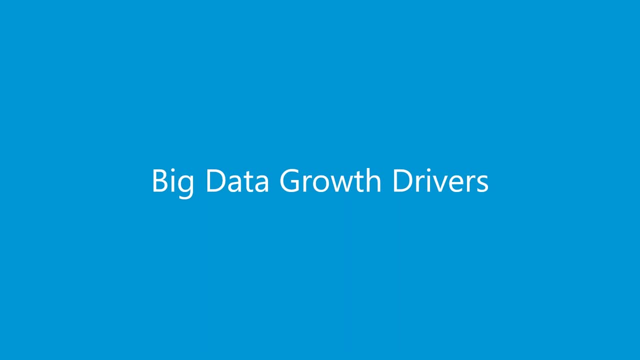 set of data or to process, structure data. but over the years, our requirement has changed. we are, we are dealing with different types of data, and data is getting generated at a very high speed, so the so the problem is we cannot use the tool or the technology which came into the market 25 years back, right. so 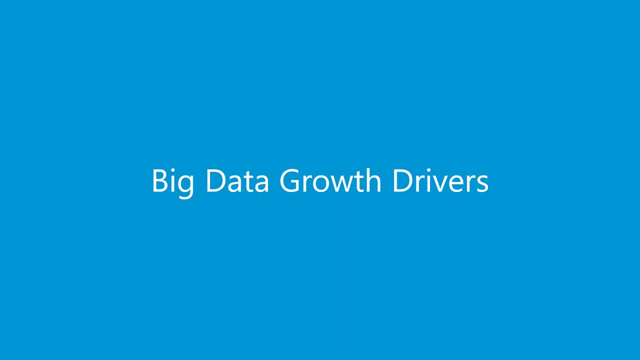 that's why what we are saying, we are saying that big data is nothing, but it's a problem which industry is facing right now. you know why? because we do. industry has got the experts on the tool or the technology which came into the market 25 years back, but that expertise is not. 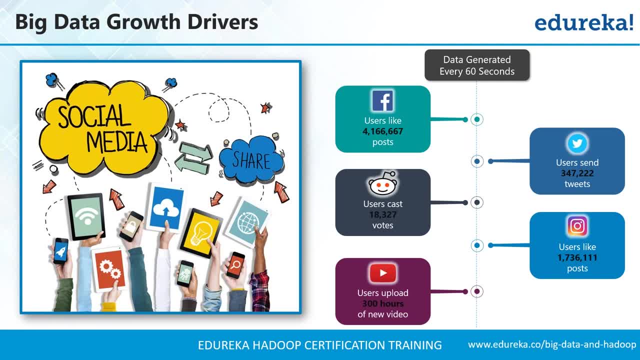 gonna help us now, right, that's why we are saying that, hey, we don't know how to process this data, how to store it, and that's why we are saying that it's nothing, but it's a problem in general. fine, so now if we talk about big data, 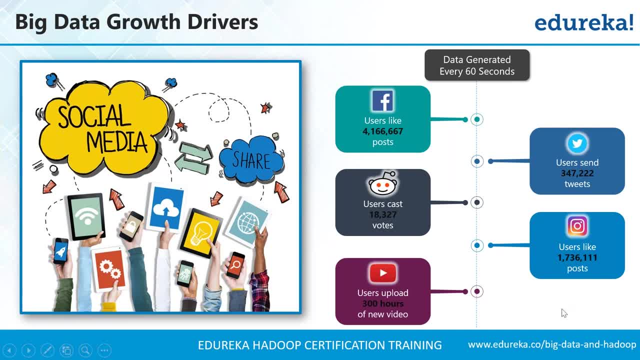 growth. drivers, as in you know why the scenario has changed, or why, suddenly, data is increasing at a very high speed, or why do we have variety of data? okay, draw drivers. I think you, you all are. it's like we all are responsible for generating this use amount of data. right, so we are are using social media. 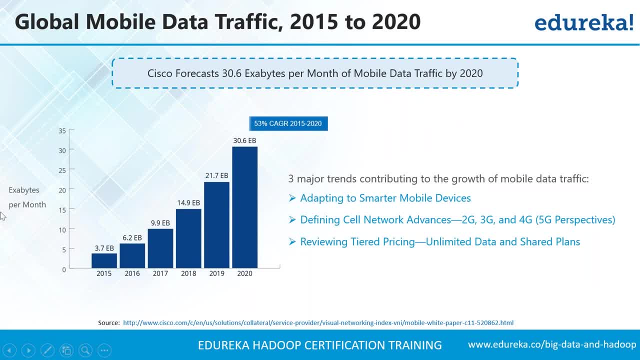 platforms like anything today, right. so what we are doing? we are generating the data. so, if you take example of Facebook, YouTube, Twitter and Instagram, right, for all of these social media platforms, data is increasing at a very high speed. okay, data velocity is very high. and also, if you talk about facebook or if you talk about insta, right. 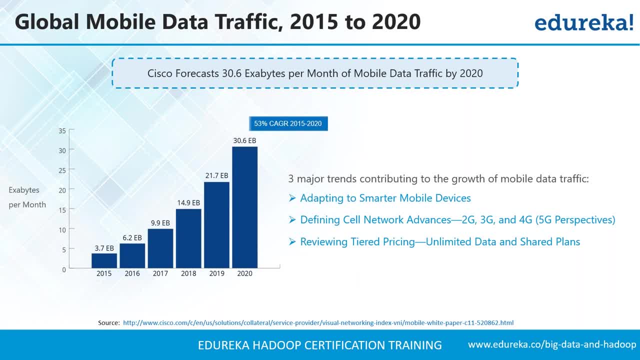 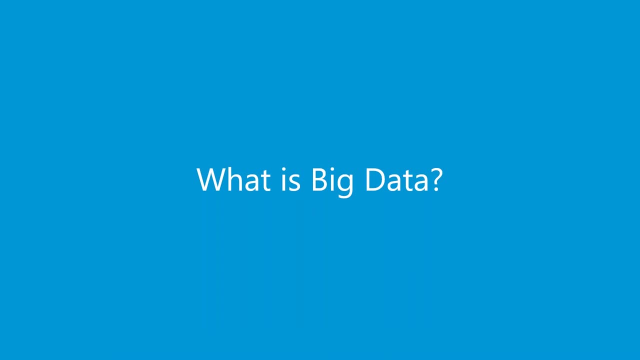 so we do have varieties of data as, and we do have text data, we do have audio data and we do have video data as well, right? so global mobile data traffic- it's like data- is increasing at a very high rate. so this is what the graph is depicting. it's saying that you know the data growth is very 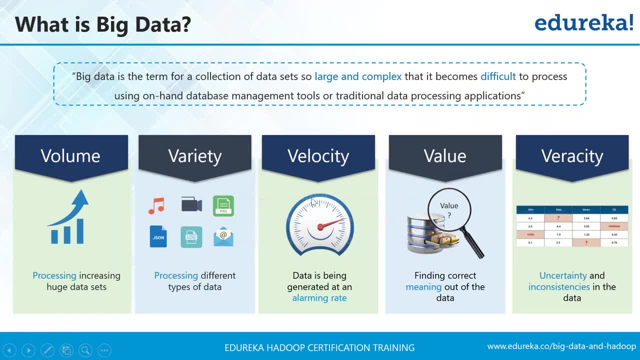 very high and if we talk about it's like nowadays we are, we are interested in using high speed network, right. so we moved to 4g from 2g and 3g and eventually we'll be moving to 5g, so higher internet speed as in like, we will be uploading or we will be downloading a huge amount of data, right. 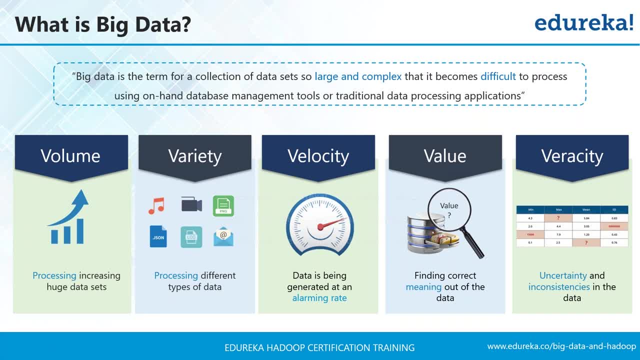 so, yeah, what is big data? we have talked about big data in general, like we said, that it's nothing but it's a problem. so now, when it comes to the technical definition of big data, what does it? it's a data which is getting generated at a very high speed. 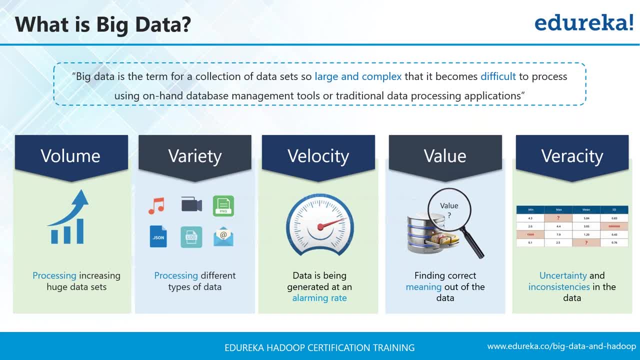 that's why it will have a very huge size and it has got varieties as well. right as in, the data is getting generated at a very high speed. it is used in size and, of course, the data is generated at a very high speed. also, it has got varieties, as in it it has got text data, audio data and video data. 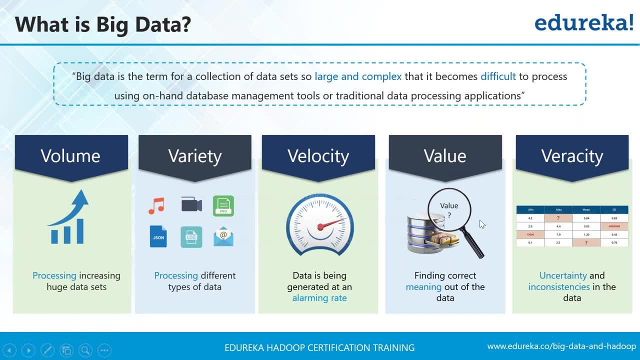 okay, so technical definition says that big data is nothing, but it's a term for a collection of data set which is so large and complex that it becomes difficult to process using existing tools or the technologies that is what we had already discussed. so, guys, when, uh, when- we started talking about big data- initially- right, we used to talk about three v's, where we used 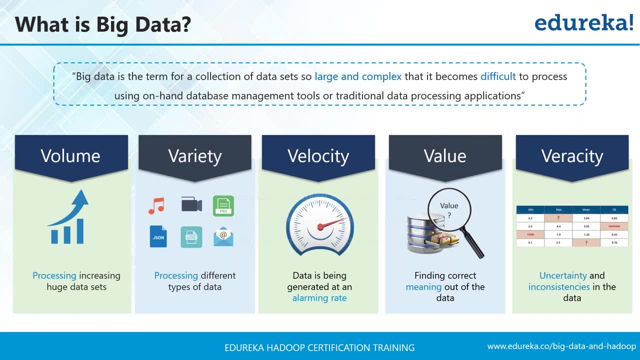 to say that, you know, it's related to velocity, it's related to variety as well as with volume, so that's why we used to say that these are nothing but the three v's. right, but nowadays we are concerned with value as well as with veracity. okay, so what is value? as in guys. 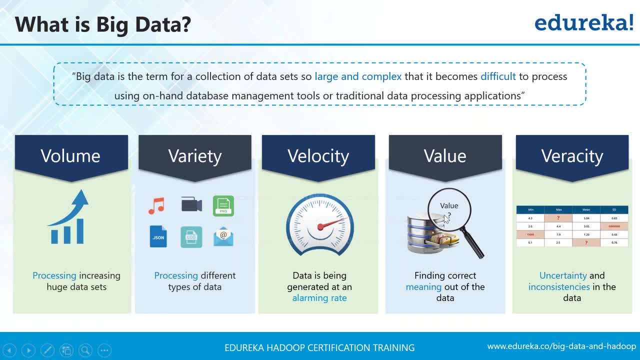 it's like every day, you are generating huge amount of data. let's say, every day you are consuming huge amount of data. that's what you're doing, but the point is if, at the end of the day, if at the end of the day, you are not able to find the quality of the data which is what we would say in the case of big data, 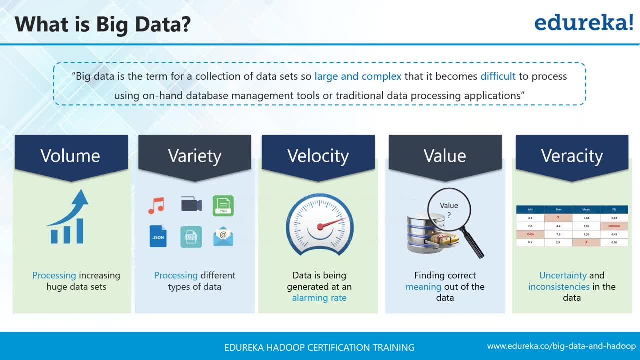 correct meaning out of the data, there is no point. why do you think that you will spend so much for the storage and for the processing of the data if you don't know what, what the story is right or it's like, if you are not able to find the correct meaning out of the data? you would not want to? 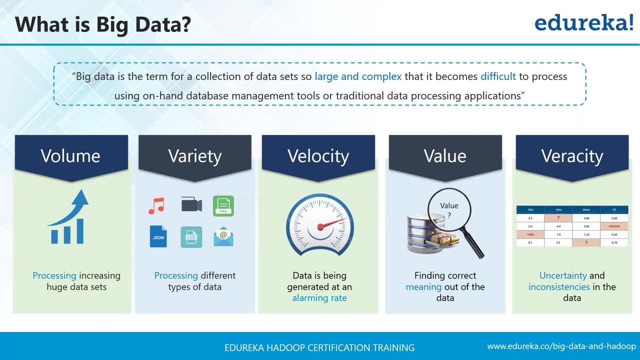 spend much, right, so that's what it is right. so it's like, objective is to find the correct meaning out of the data, right? and what is this veracity? this veracity is nothing, but it is uncertainty and inconsistency in the data. right, uncertainty as in. okay, sometimes we will look at the pattern. 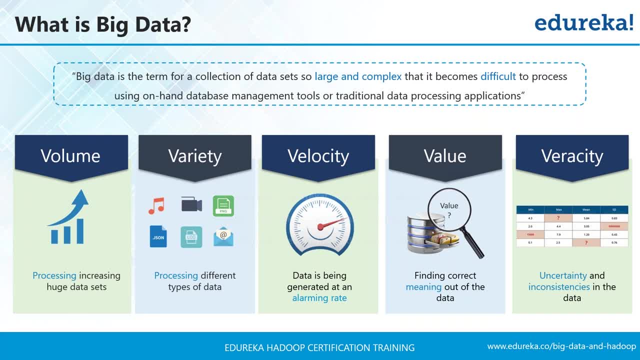 and we will say that, okay, we have missed some data or we do have some junk data. so, basically, all of all of us are- all of us are interested in doing the analysis on valid data. we are not interested in doing the analysis on junk data. so the point is, if we are doing the analysis on junk, 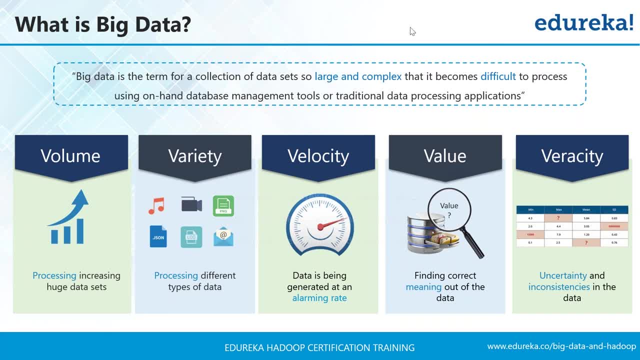 data, we will not be generating accurate reports, right, we will not be generating accurate reports. so that's the point. that's what veracity is. so when we talk about big data, we talk about these five B's, right, which is volume, variety, velocity, value and velocity. okay, so guys. 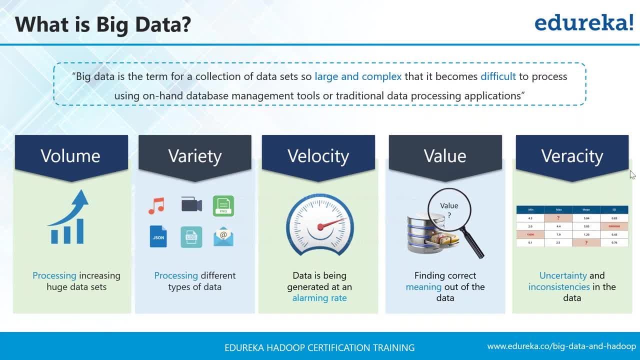 are you following? is the definition of big data clear? so those who are completely new to big data, guys, are you following? is the definition clear? is it clear? like, what is big data? and why do we say that it's nothing but it's a problem? can I get yes or no from all? please, guys, please don't hesitate if you. 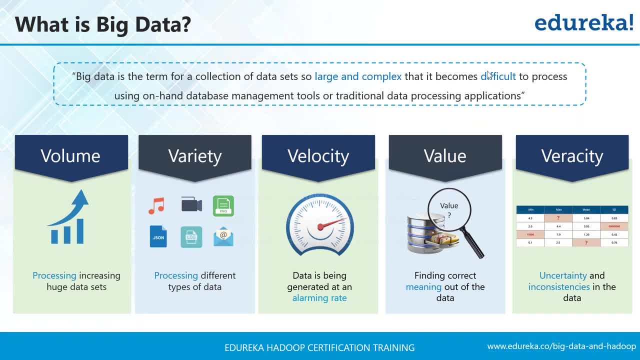 have any questions or any issues, you can always bring me in the chat window. okay, perfect, so let's move on, okay, yeah, okay, the one veracity is nothing, but it's the unconsistency or the uncertainty in the data, as in whatever messages you receive on whatsapp or on facebook, not all are genuine or valid. right by looking at some of 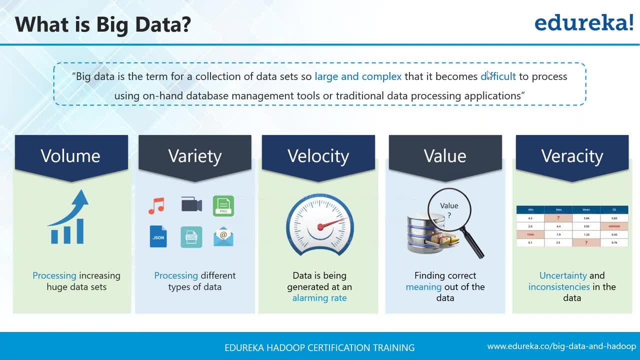 the messages, you will say that, hey, this is a fake message, right? or this is a fake video, right? so the point is, we are not interested in generating the reports on the data which is not valid or which is fake, right, we don't want to do that. so the point is, we need to find this kind of 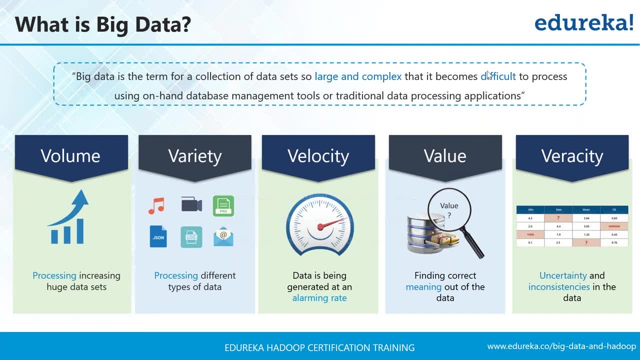 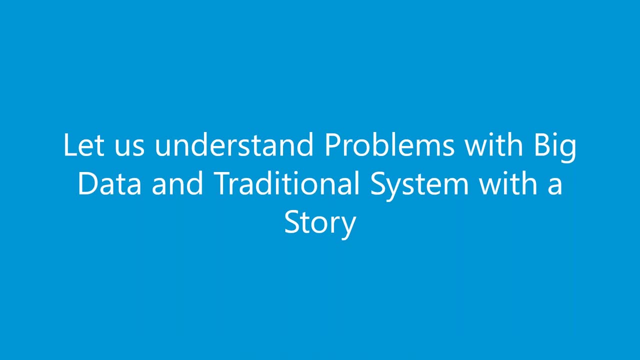 uncertainty or inconsistency in the data where we are able to make a call and where we are able to say that, okay, hey, this data is not of any use. so not every data which you are receiving over the network is genuine and valid. so that's why what we say- we say that it has got some uncertainty and 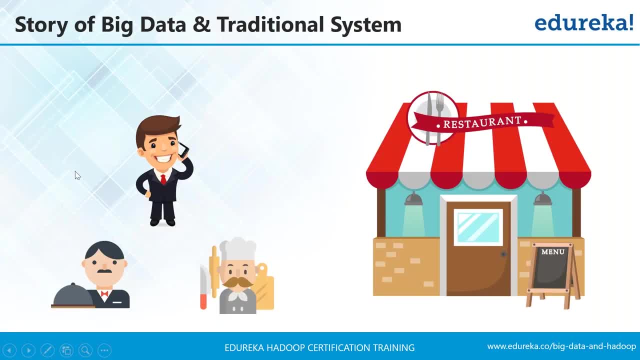 inconsistency. you okay the one says: from data, how would you segregate? yes, the one. that's what data scientists are doing, right. so this is a, this is a job of data scientists. where they make a call, they do have algorithms running. they are doing n number of things to to say that, hey, this is the valid data. 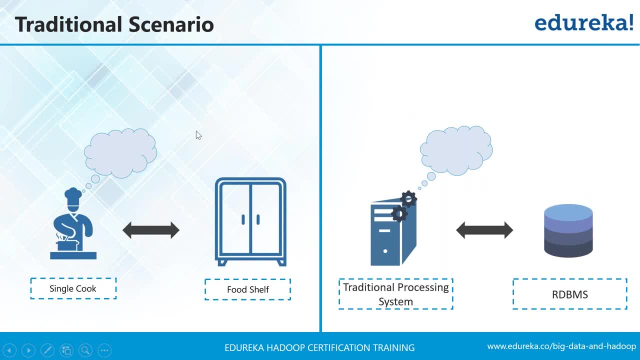 and this is the junk data. okay, can i know how it is different from database? yes, money going forward. you will understand that. okay, this is just the data. so now the problem with big data and traditional system. okay, so, guys, this this is a very you know, uh, initially, uh, what do you see? this is the traditional system. 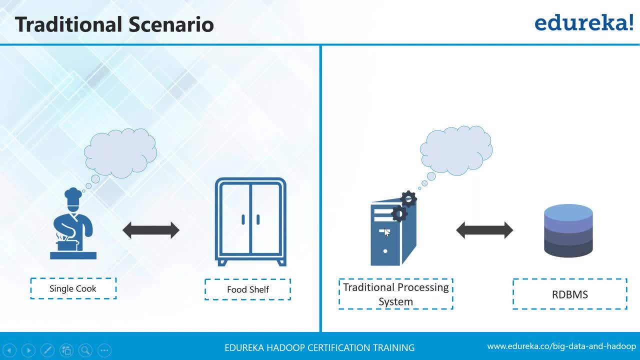 okay, so it's like there is this restaurant and there is this manager. uh, then there is this, uh i mean the one who, who will be serving the food, and then we do have chef, right. so it's like this was a small restaurant, so it's like whenever, uh, some order was coming, so there was a restaurant. 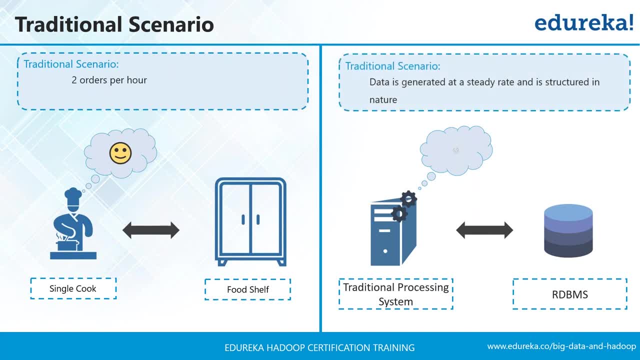 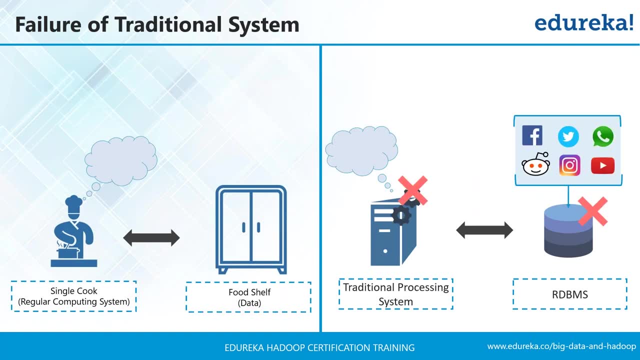 was single cook who was preparing the food, who was keeping it in the food shelf and then it was being served to the customer, right? so if we discuss it technically- sorry, if we discuss it technically right, so there was one single machine. here is your database. okay. so whatever data this database was, 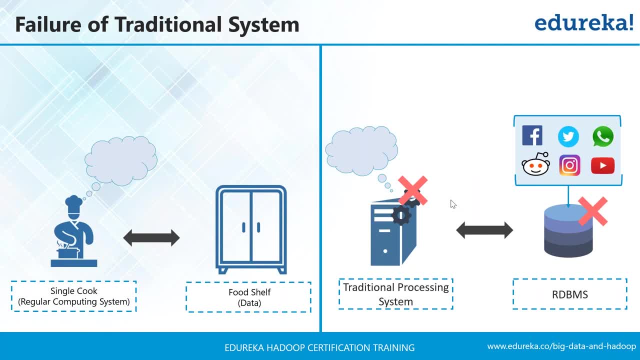 having who was processing it. there was this server, or this single machine, or a single server, which was, which was processing the data, fine. so now it's like initially, because the load was less, so single cook was able to handle that, fine. so now what has happened? so now, what has happened? it's like the 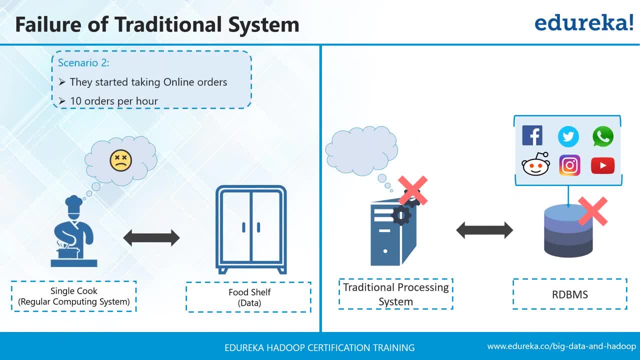 load has increased. right load has increased, so failure of traditional system. it's like if you talk about rdbms, right? rdbms is designed specifically for structured data, right? so now these days, we are dealing with facebook, instagrams, like we do have unstructured data in the form of audio and video as well, so do you think that you can store that kind? 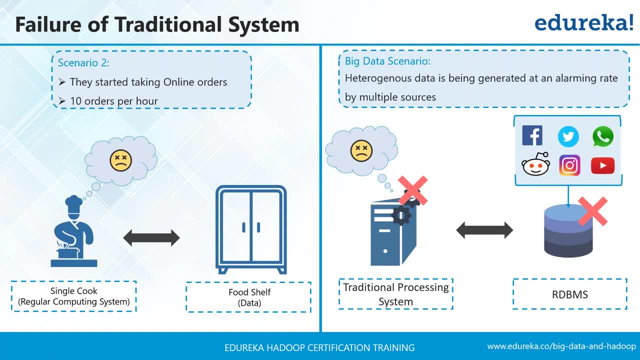 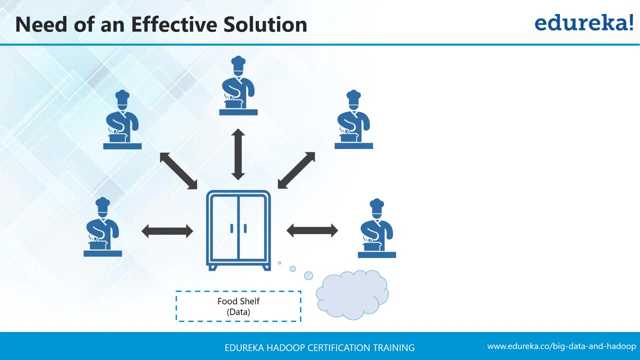 of data in rdbms. no, so traditional system failure, right. so now, if we, if we talk about this chef, right, the chef is saying that, hey, i'm getting too many orders down and it is becoming quite difficult to serve the customer on time. right, so this was the problem with the traditional system, okay, so 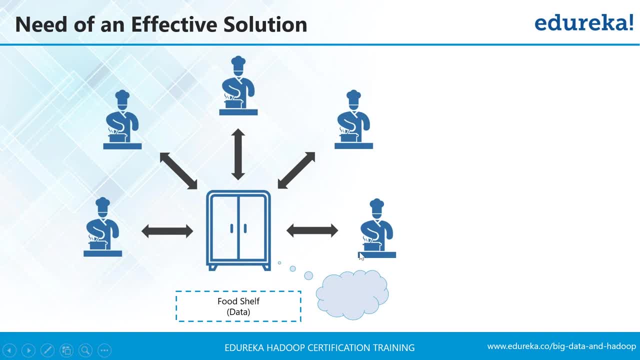 initially what was happening? a single server, server was processing the whole data set. right, because data was small and it was structured. but now a day scenario has changed completely. okay there. that's why we say: failure with the traditional system, okay. so now if we talk about the solution? okay, if we 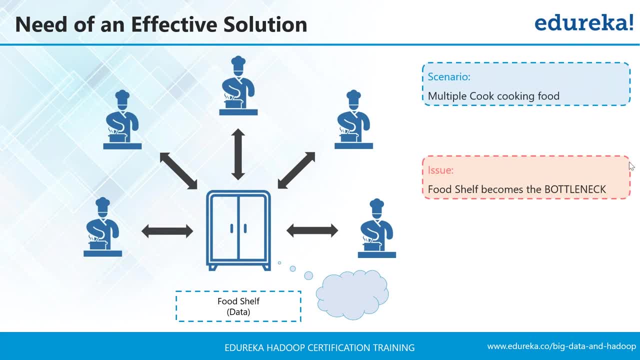 if we think from this chef's perspective. so what we can have is, instead of having only one cook, we can have multiple cooks, or we can have multiple chefs who will be preparing the data and would be keeping it in the shelf, right? so, guys, this shelf is nothing, but it's a. 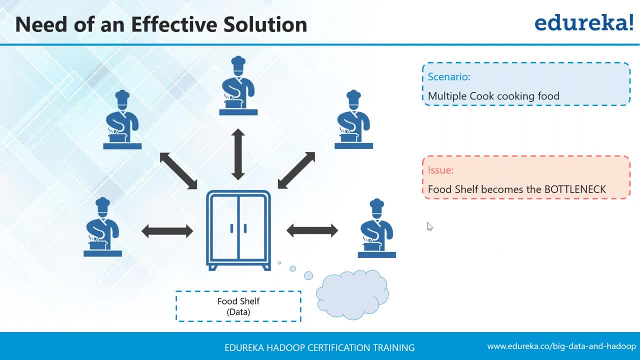 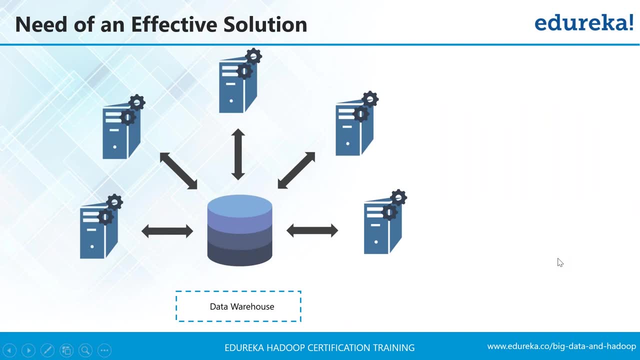 storage. this shelf is nothing, but it's a storage where we will be storing the data. okay, but now what can be the problem? problem can be with the storage. okay, problem can be with the storage. right, so it's like because multiple cooks are, uh, preparing the food and they are storing the 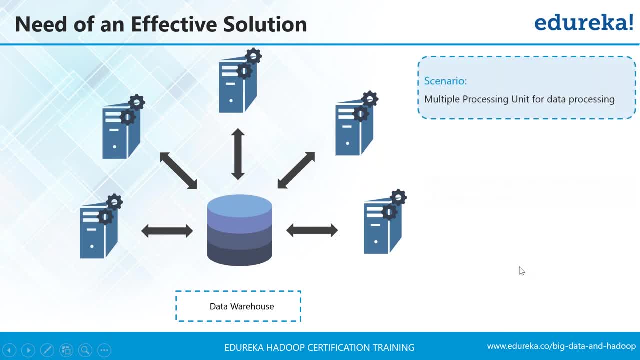 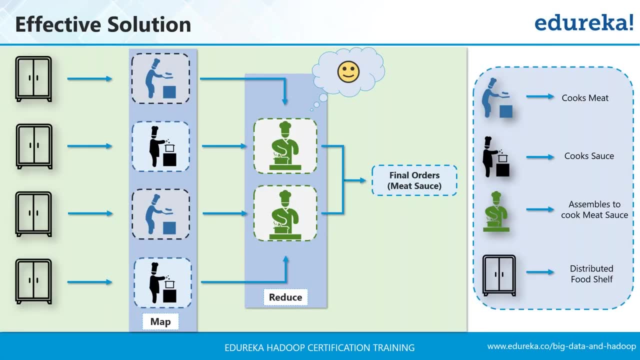 data in the same shell. so we can say that: okay, you know, we do have less storage space now. so now what we can do is to each of the cook we can give one shell or one storage a space, right? so here what you see: multiple machines, but all are writing the data to the same data warehouse again. 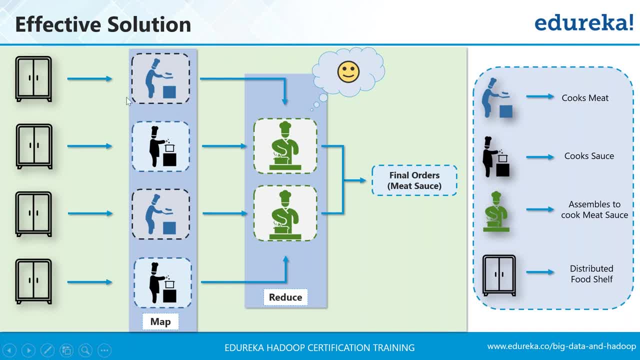 it can be a bottleneck. so what do we have? we do have this scenario right. so it's like: each of the cook, right, they are having their own shelf. and when it comes to the serving the customer, right. so let's say that, for a customer a, this chef is preparing item a and this is preparing item b. 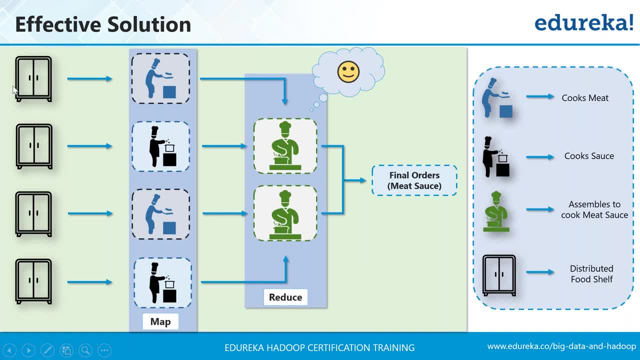 so the one who will go to serve the customer, they will aggregate or they will get the food from all the shelf right and then they will serve it. so this is what hadoop is okay. so basically, first of all, your data with data will get distributed to the different different machines. 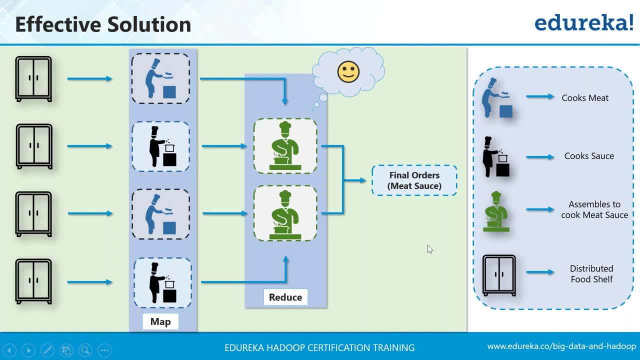 machines processing the data in parallel and, when it comes to the serving of customer, aggregation will happen. that is nothing but the reduce and then final order would be served. okay, so this is this is what effective solution is. okay. i have a question here, guys, and the question: 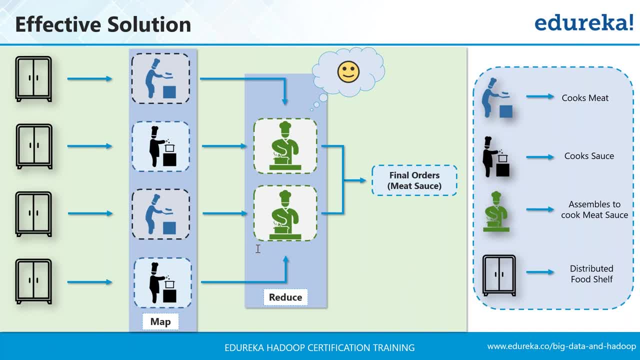 is from. uh, yes, and the question is from Sudesh. this is but system like Oracle did allow to operate in real application cluster mode. why is it still a failure? real application customer. so, Sudesh, who was it doing the parallel processing? was multiple servers running in parallel? I don't think so. no, 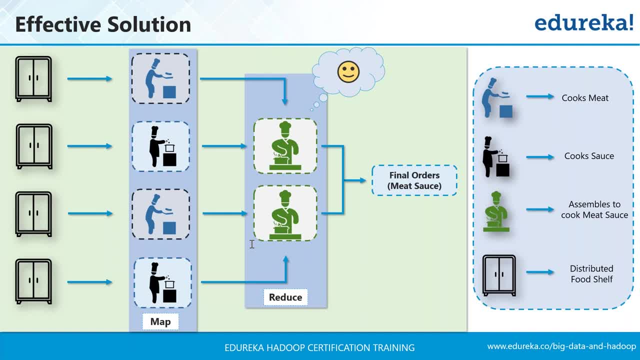 it was doing the parallel processing, where you know one machine who was acting as if multiple machines are running in parallel. right, yes, right, so that that that was. that was the main problem. problem here: I'm not saying that one is acting as of multiple. you know, cooks are preparing. 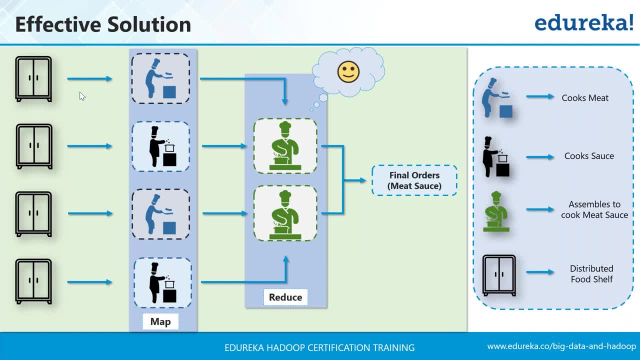 here. What do we have? We do have in actual multiple servers, but if you talk about the parallel processing in Oracle, it's like only one server, but it was behaving as if multiple threads are running or multiple servers are running in parallel. That's where the difference. 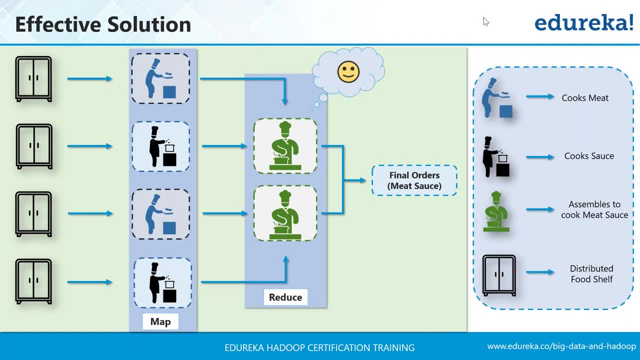 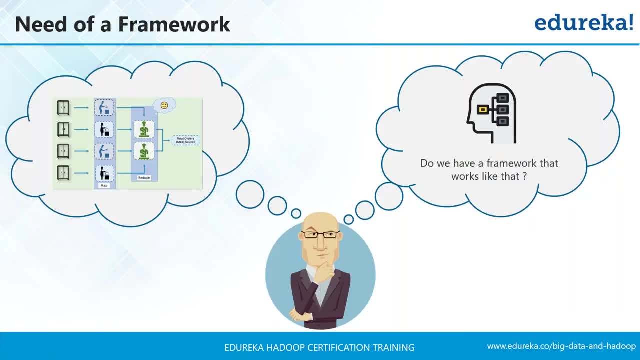 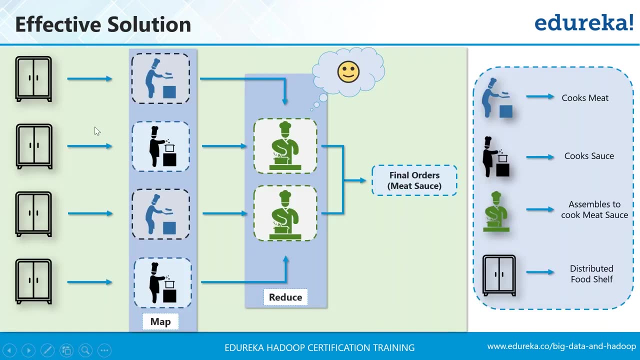 is Yes, Yes, Yes, Correct. Oracle DB: it still has one engine, but when it comes to Hadoop, it has got multiple engines. That's the difference, Okay, So yeah. now it's like: what do we need In order to do this kind of thing? right? It's like: whatever order. 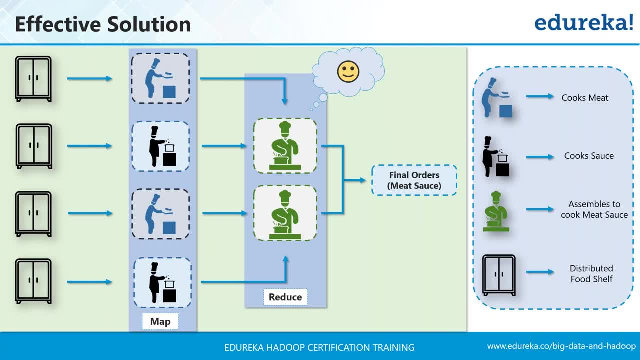 is coming from the customer, it should get distributed to the different different chefs or the cooks, and then cooks would be storing the prepared food on the different different shelves, And then we need someone who will aggregate it and then it is then serving to. 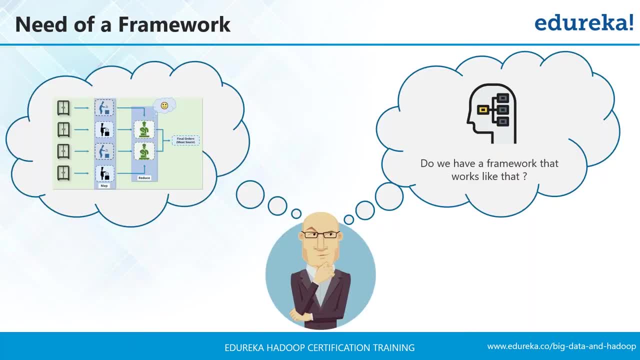 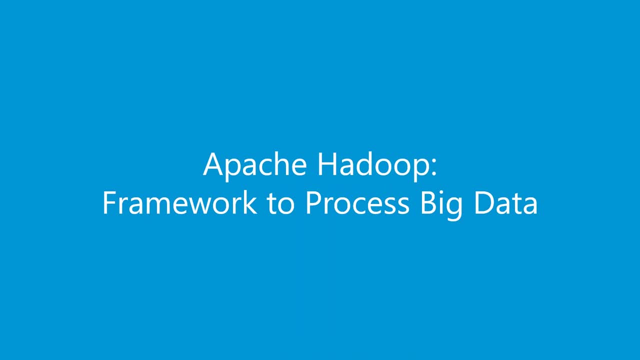 a customer, right. so the point is now: in order to do all these things, objective is to find a framework. okay, so we need to understand like: is there a framework using which we can do all those things? answer is yes, okay. so what do we have, guys, we do have hadoop here. okay, hadoop is nothing, but 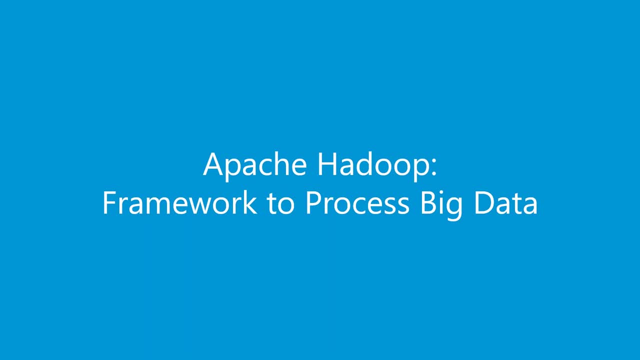 it is a framework, so, which is designed specifically for big data. hadoop is nothing, but it's a framework which is designed specifically for big data, so why are we saying that it's a framework? so, guys, as an framework. so what is our basic understanding on the framework? as in, it will have n number of 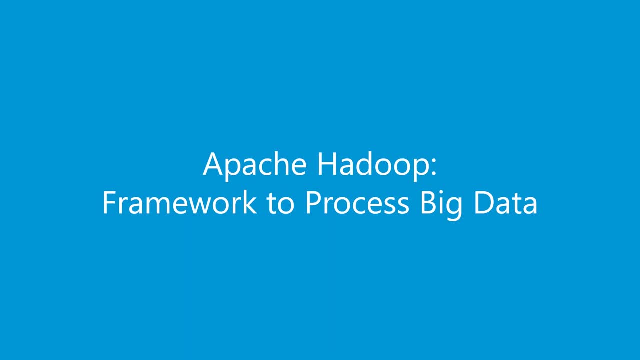 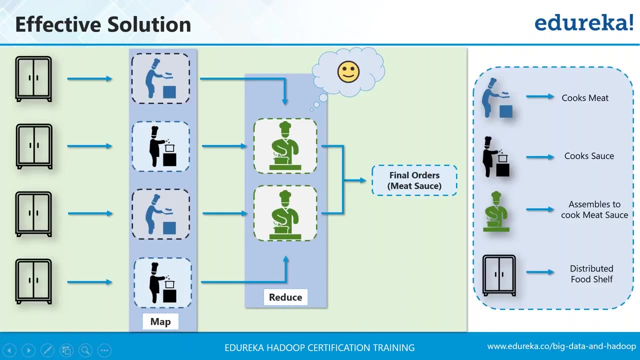 inbuilt functionalities. right, it's like: basically, it will have n number of inbuilt functionalities. so it's like you, you just need to write code for you. you don't need to write code for n number of things, you will just be using the inbuilt functions and your work will be done. so now, when we talk, 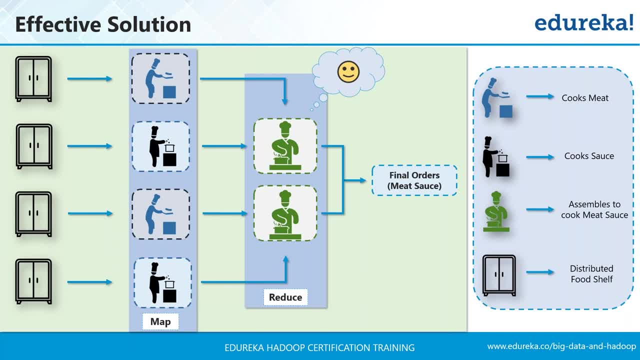 about this whole process right, where we are saying that first the order should get distributed to multiple cooks and then multiple cooks will be keeping that data in different, different shelves and then the aggregation will happen and then it will be served. right, so you don't need to write a logic for this. 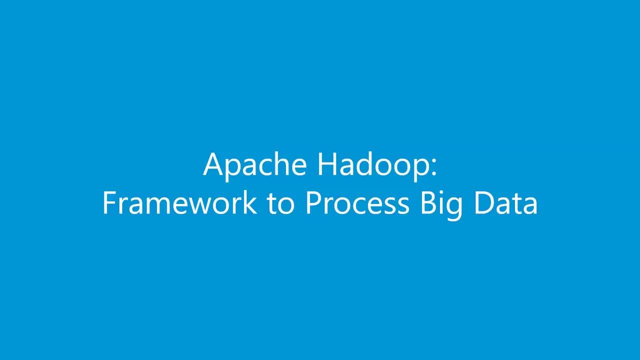 because this is something which is being handled by the framework. as a developer, you will just be focusing on the implementation of the business logic. so that's why what we are saying? we are saying that hadoop is nothing, but it is a framework which is designed to be used for. 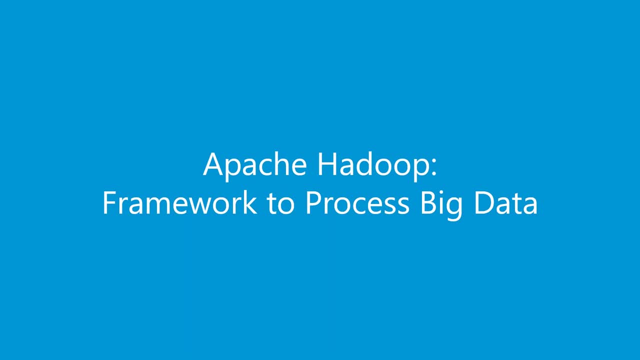 design specifically, which is designed specifically to store and to process big data. okay, so this is, this is what hadoop is. so big data is nothing, but it's a problem, and when it comes to hadoop, it is nothing but it's a solution. okay, so, guys, are you all following any questions so far? 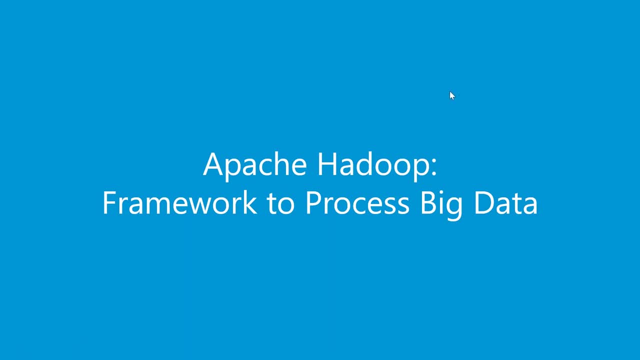 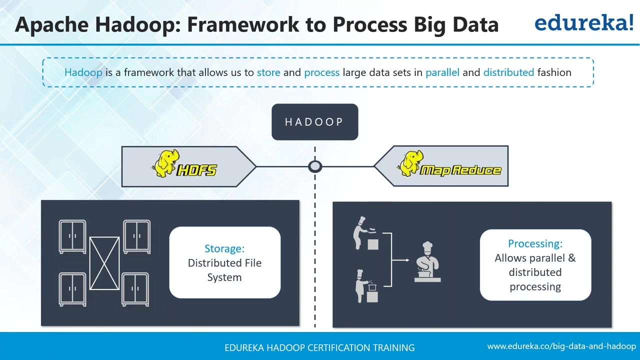 any questions, guys? okay, i don't see any questions coming, so i hope you all are good so far, let's move on. okay, okay, okay, okay, okay, okay, okay, uh, yes, okay, so now we'll talk about map reduce, okay, so, guys, now, when it comes to hadoop as a framework, what i said? i said that the code is: 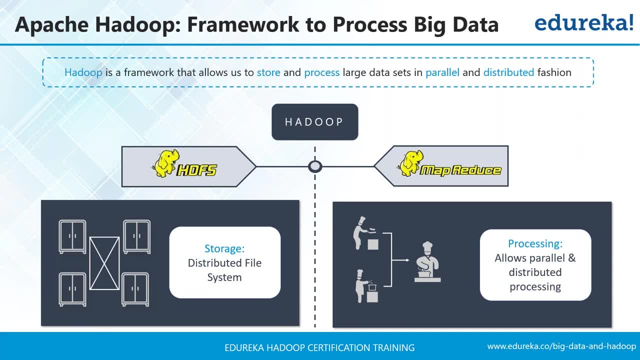 already written. give me a second. i said the code is already written, right, it's like it has got n number of inbuilt functions. uh, it has got n number of inbuilt functions which you can use. you know you will. you will not be focusing on the distribution of the 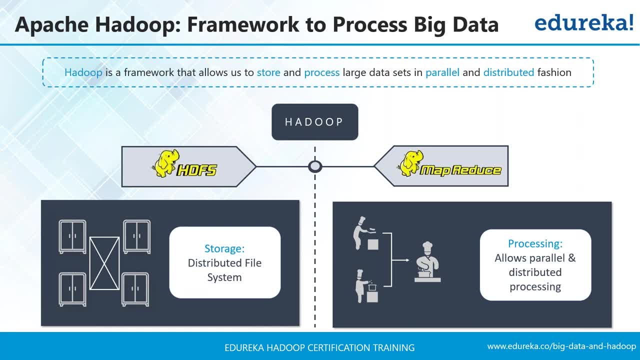 data, or you will not be focusing on the parallel processing. it's like, what is your job as a developer when it comes to uh, the users of hadoop? so, guys, it's like let's say that your objective is to find the uh maximum number. uh, objective is to find the maximum number out of some n numbers. 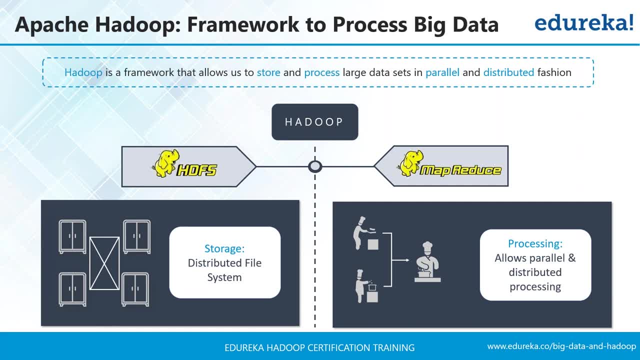 right. so now what? what you will be doing as a developer? you will be focusing on writing the logic where you will say that, okay, hey, this is how maximum, uh sorry, the largest number. you will be finding it out, okay. or you will be, uh, finding the maximum temperature, or something. 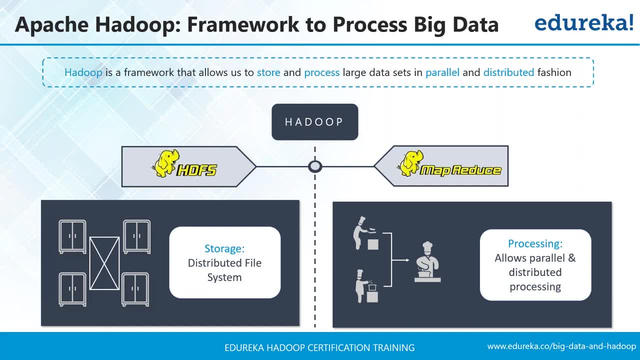 like that. okay, largest number objective is to find the largest number out of n numbers. so what you will be doing as a developer, you will just be focusing on writing the logic using which you will be able to find the largest number. fine, so you will not be writing the code for the distribution. 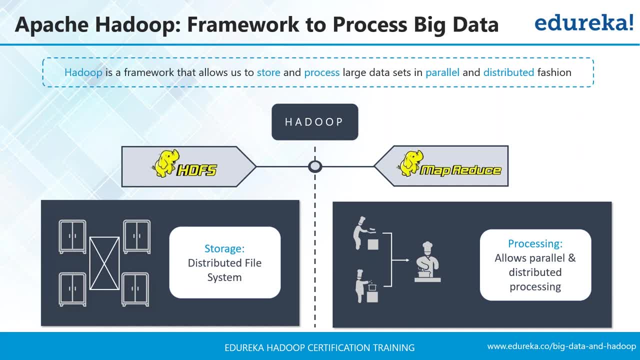 or you will not be writing the code for the parallel processing. you will not be telling hadoop that, hey, this is how the data should get distributed or this is how the parallel processing should happen. you will not be doing that. so who will do those kind of things this framework will be doing. okay, hadoop, as a 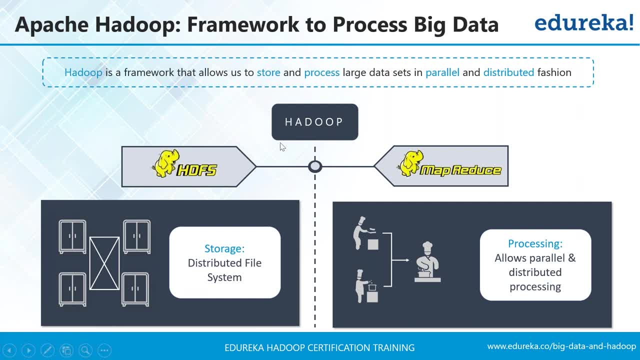 framework will be will be taking care of the distribution as well as of the parallel processing. so, when it comes to hadoop as a framework, what do we have? we do have two core components: one is for storage and one is for processing. so the component, the core component, which is there for storage, that's nothing but hdfs. okay. 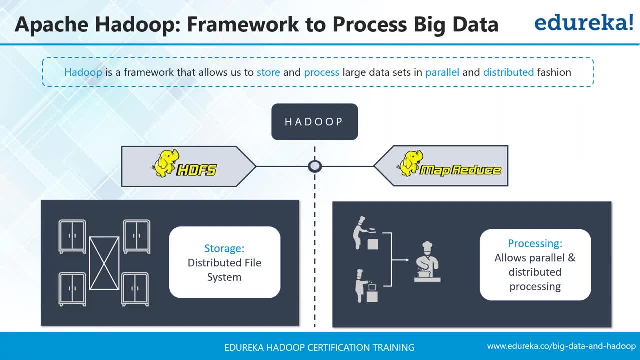 so this is the component which says that, hey, i will take care of the distribution. it says that, hey, you don't need to write a code for the distribution as a developer, because this is my job. okay, so it's like: in order to- in order to work on hadoop, you need to get the understanding. 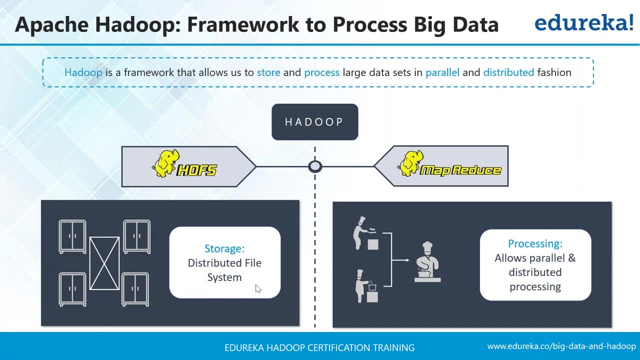 of these two core frameworks, like how they are working internally. even though you will not be dealing with these components directly, you need to get the understanding of these two core frameworks correctly, but you need to understand the architecture, like how these components are working. okay, so hdfs stands for hadoop, distributed file system, dfs as a distributed file system. so if i 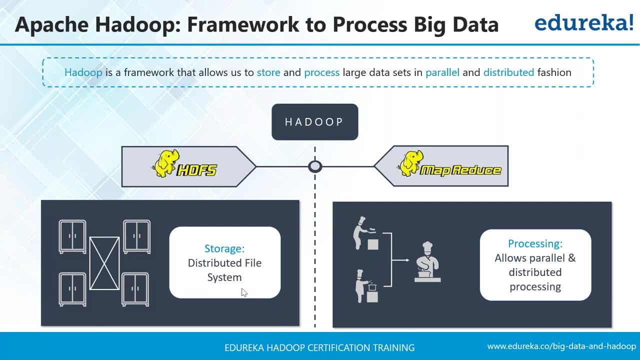 talk about traditional system, right? so what do we have? we do have a file system, like we have ext3, ext4 or 532, right? so these file systems are. these file system are operating on a single machine, but when it comes to hdfs, you need to understand the architecture, like how these components 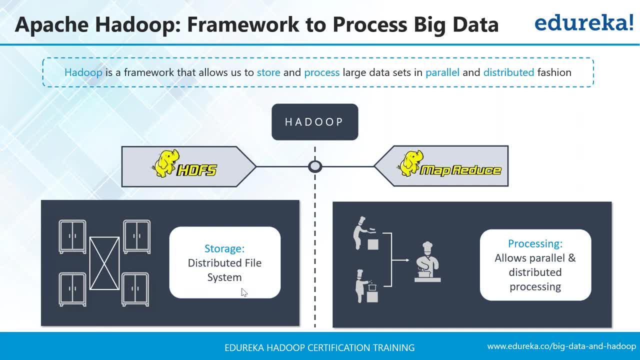 are operating on a single machine, but when it comes to hdfs or when it comes to the parallel processing or the distributed computing, it's like multiple machines would be running in parallel, like we took the example where we said that multiple chefs or multiple cooks would be. 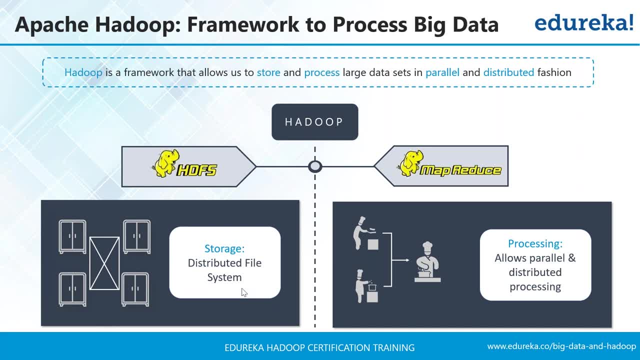 preparing the food in parallel, right, so what is that? it's like now? there is now and and. when it comes to uh, when it comes to uh serving the final order to the customer, what we do? we do the aggregation. but internally, what is happening? multiple chefs are working on preparing the food. 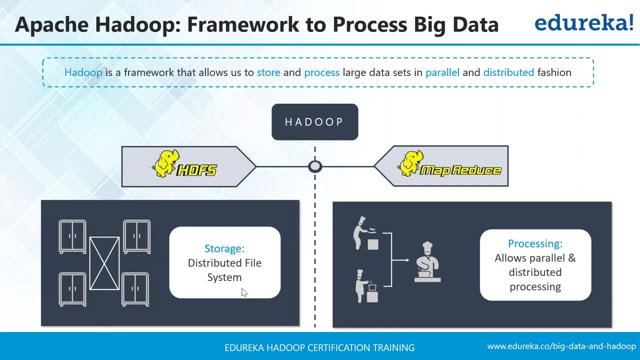 right. so this is what distributed file system is, as in your data is there on multiple machines. it is distributed. so this file system it's not working on one machine, it's working on n number of machines in parallel. so that's why we are saying that it's a distributed file system. okay. 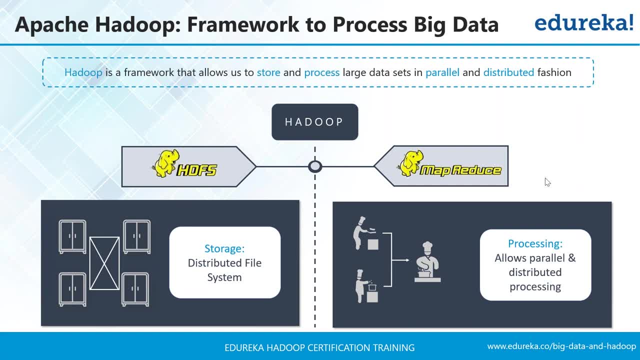 okay. so, guys, are you following? it's the concept of distributed file system, clear, okay, here we have multiple storage and multiple processing for one output. yes, reika, perfect, right, so all these things are working towards generating the single output. okay, it's the concept of distributed file system. okay, so, guys, are you following? is the concept of? 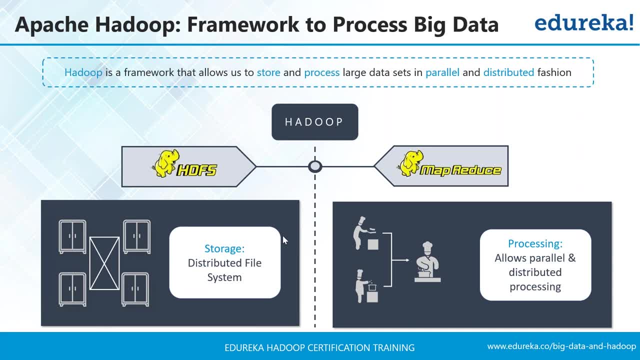 distributed file system. okay, it's the concept of distributed file system. okay, it's like you say that, hey, you, it's like you say that, hey, you are interested in finding the largest, are interested in finding the largest, are interested in finding the largest number. but internally it's like not only. 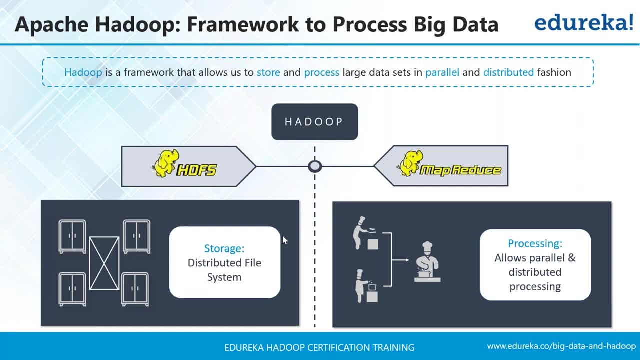 number, but internally it's like not only number, but internally it's like not only one machine. one machine, one machine. n number of machines would be running in n number of machines would be running in n. number of machines would be running in parallel, as in parallel, as in. 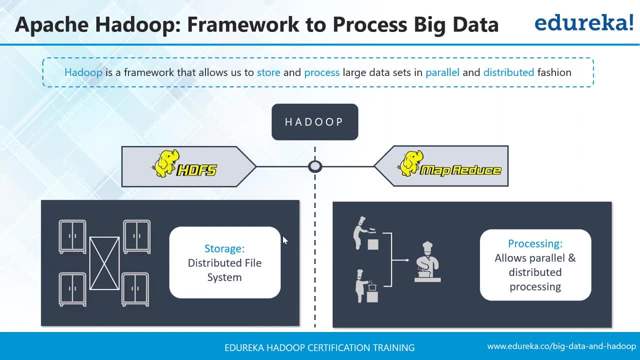 parallel, as in: i do have a file okay in the file, i do. i do have a file okay in the file, i do. i do have a file okay in the file. i do have numbers from 1 to 100- okay, what am i? have numbers from 1 to 100- okay, what am i? 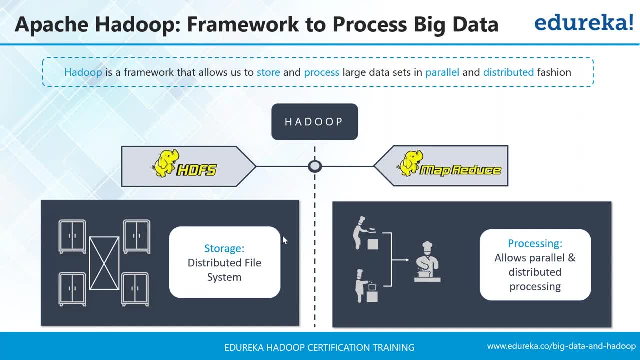 have numbers from 1 to 100. okay, what am i doing? i'm giving that file to one resource and i'm asking that resource to find the number 99. so what that resource will do? that resource will read each and every number and after five minutes, the resource will say that i found the. 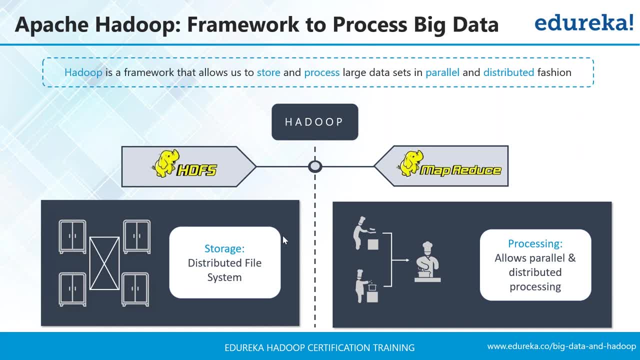 number 99. okay, and i'll be like: hey, no, five minutes too much time, so can you please reduce the time? resource will say that, no, i did my best and i don't think so that i can do it in lesser time, right. so now, as a manager, i'll say that, okay, let's do one thing instead of giving all the 100. 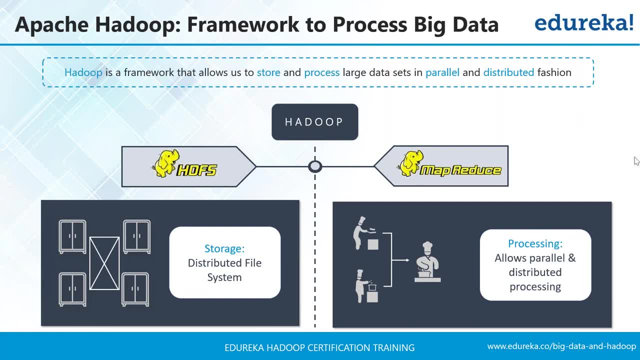 numbers to one resource. let's do one thing: let's distribute this file to other resources as well. so now, first 20 numbers, i'll be giving to one the source, next 20 numbers to another resource, and like that i'll do the distribution. then i will be asking all the resources to work in parallel. 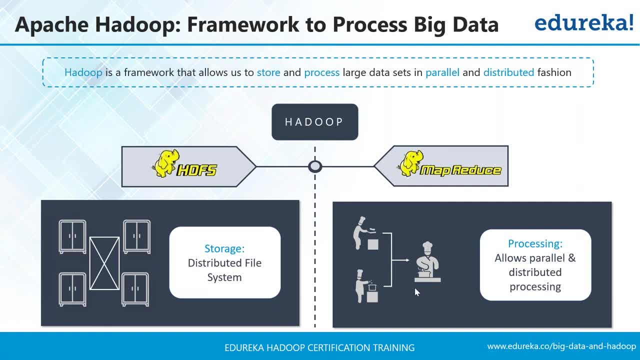 for finding the number 99, for finding the number 99. okay, that is something. that is something which we call as distributing file system or parallel processing. okay, yes, it has a set of servers. yes, cluster, it is a cluster. okay, so now, when it comes to the hdfs is like first distribution, and then i told you right that, when it comes to observing, 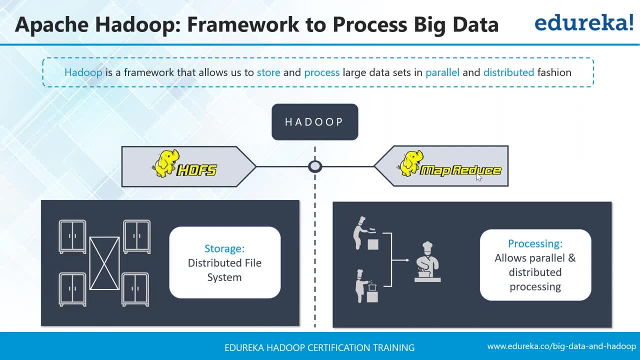 the uh final order to the customer. or let's say that we, we are interested in adding the sauces to uh, all the food which is being prepared by a different, different chefs, right? so here, what this cook is doing or this head chef is doing, this is just adding the sauces, right? 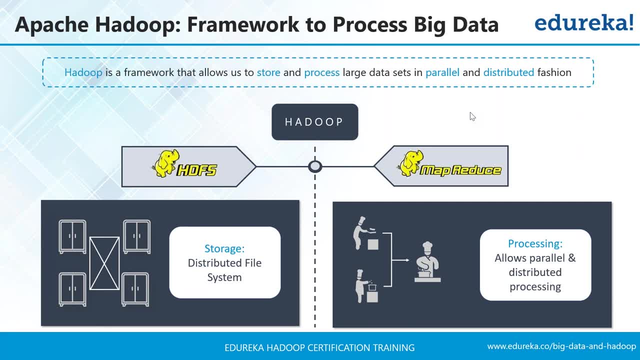 so that it can be served to the final customer. so this is what this is, nothing but the concept of parallel processing. no, no, no, srikumar, it's not the same file. that's why i said that it's a distribution right. that's why i said that i do have a file of numbers with one, two hundred. what i'll be doing, i will be. 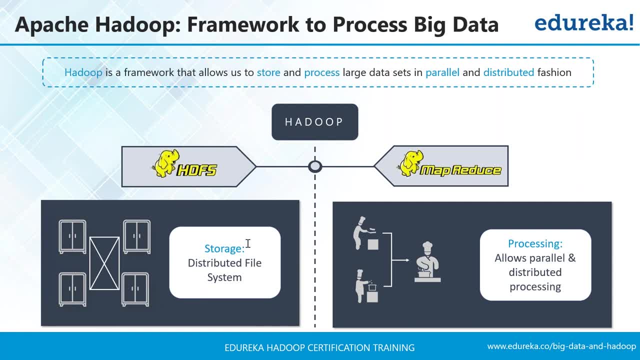 distributing it to andrew sources. right, it's not the same file i'm giving. there is no point in that case. it's like all the resources are working on the same dataset. that's not. parallel processing is okay. we don't talk of multi-task, no, it's about multi-processing. is hdfs like landing of data and map reduce like etl? 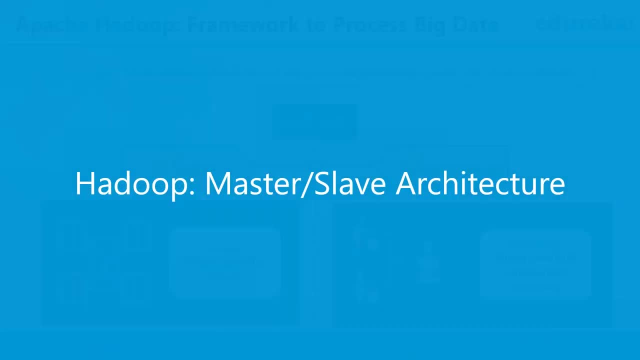 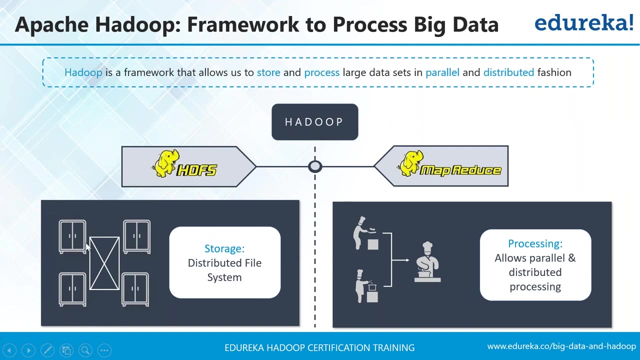 yes, map reduces, like processing the data cable says hdfs splits the file and the distribute them on different machines and each node would be processing it locally. Yes, Yes, cable. completely agree to that. So, guys, just to summarize, HDFS stands for Hadoop: distributed file system. 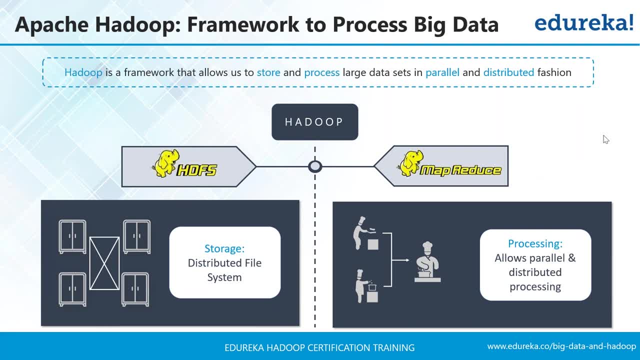 HDFS stands for Hadoop, distributed file system, And what is the role of this core component? The role of this core component is to distribute the data. distribute, guys- I'm not saying the same file will be given to all the resources It's like. to distribute the data to n number of machines. 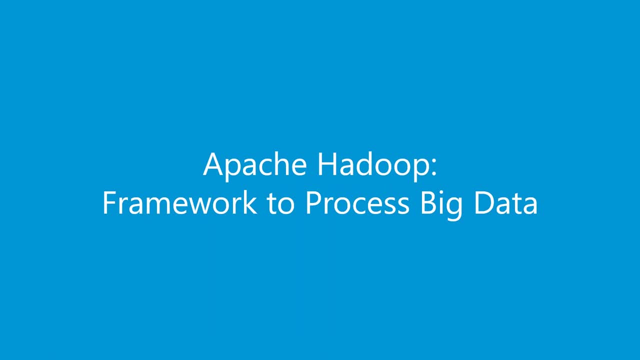 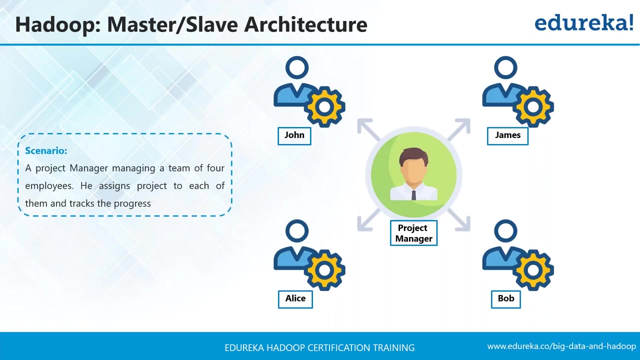 And what is this MapReduce? basically, it is a framework. for what is this MapReduce? This is nothing, but it is a framework which will be processing the data in parallel. Okay, it is a framework which will be processing the data in parallel. Okay, 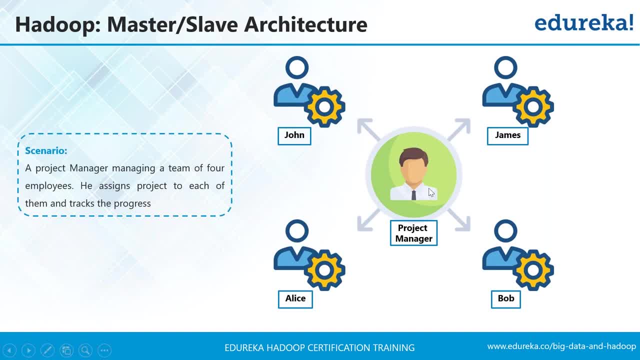 Okay, Okay. so let's move on. Okay So, guys, when it, when it comes to Hadoop Right, when it comes to Hadoop framework, Let's understand the architecture. We will not be going into the details, but we are. we will discuss it overall. 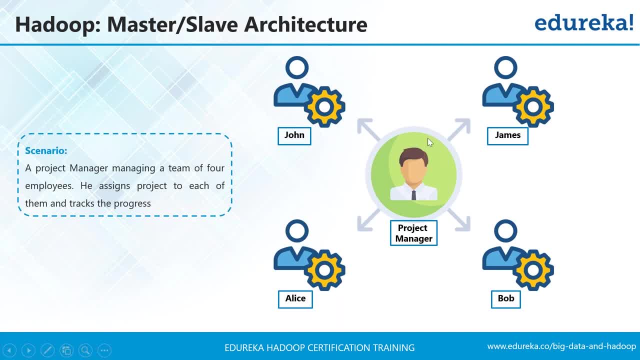 So what do we have here? It's like we do have a project manager and then we do have these resources, Right? so this project manager is having a team of four employees. so this project manager, what it will be doing, it will be assigning- sorry, it will be assigning- the project to each of the resource and then 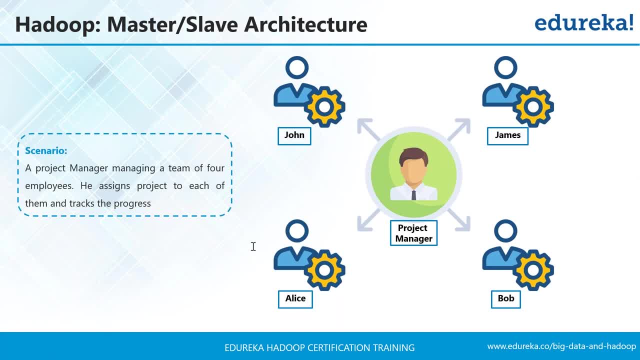 it would be, uh, like manager would be tracking the progress. this is how hadoop works, and these resources are not the virtual resources, guys. okay, these are the technically. they are the physical servers, okay, or they are the physical machines, okay, i have a question here. user file will be distributed and it will do parallel. 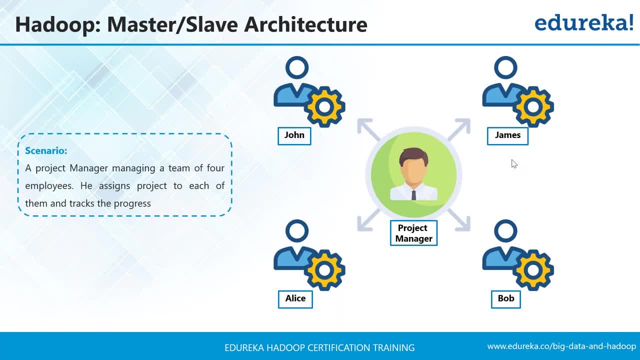 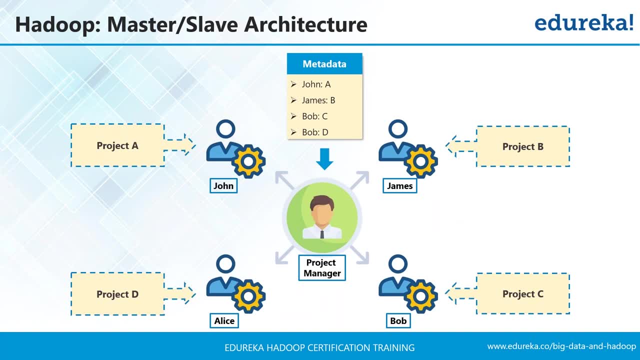 processing. what if one server go down? yes, vani, very good question. so, guys, it's like now. the point is, this project manager is has assigned the task right. so what if one of the resource goes on vacation or leaves the organization? this project manager is saying that, hey, not to worry, i don't. 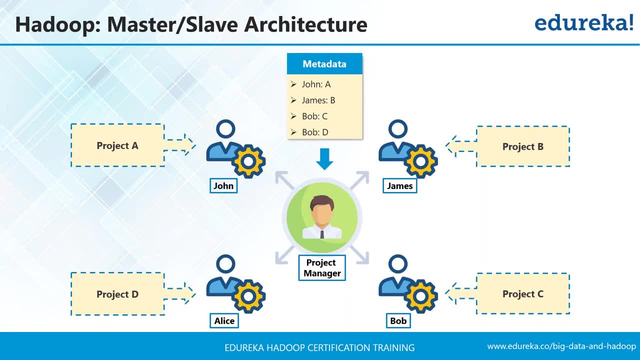 have the backup ready, right, because the data is getting distributed and we cannot tolerate the loss of a data, right? so what? what will happen? so, basically, the application will take place. replica is nothing but the backup. so whenever you write the data or whatever you are doing in the hadoop, 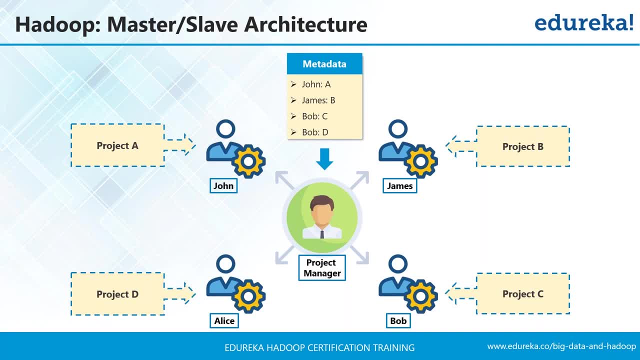 cluster. that will be replicated. so when it comes to storing a file to hadoop, right, so it's like internally, it will be storing that file three times at three different places. as in, you went for a test up and you would have. you have very good photographs and and, and you don't want to lose. 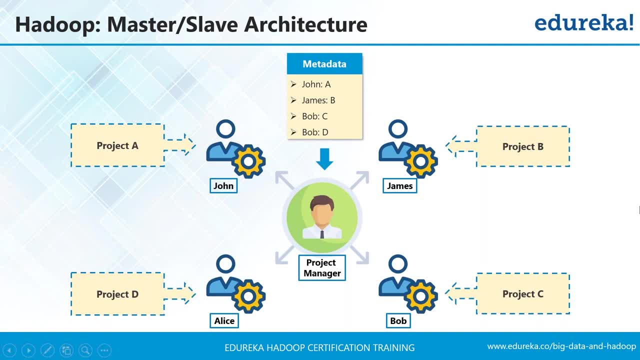 the photographs ever, and you don't want to lose the photographs ever. so what is the the main thing? so, basically, it's like what you'll do: you will upload the photos to the dropbox, right, you will? you will have it in your laptop and you can put it to the hard disk as well, right? so basically, you, 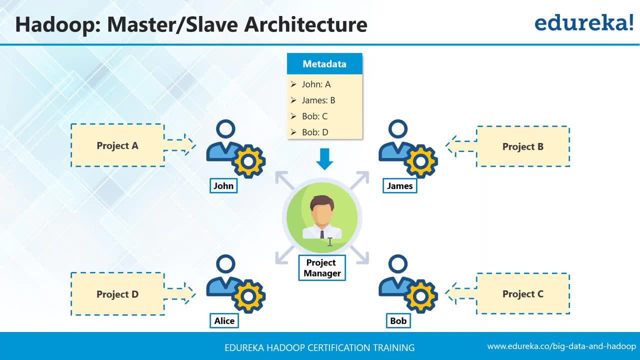 have taken the backup at three different places. you have taken the backup at three different places, so this is this is what you're doing, right same way. similarly, hadoop is intelligent enough to understand that that, because i'm distributing the data, i cannot tolerate the loss. so what i will do is: 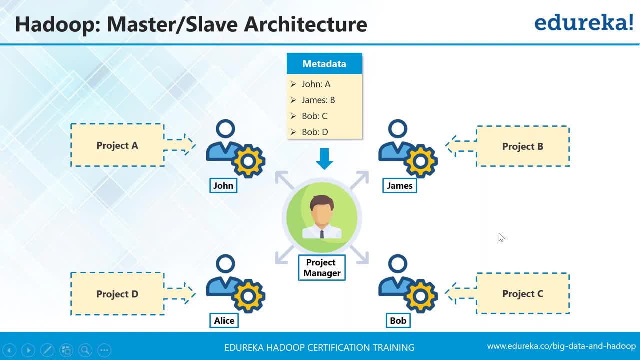 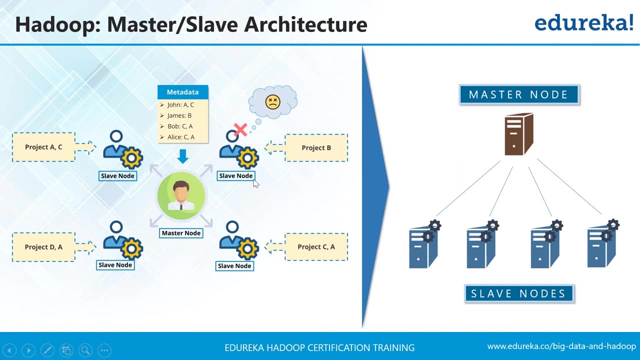 i will keep this data to the different different machines as well. okay, i have a question here. is there application happening using storage driver or hdfs? hdfs is the one who is taking care of the application, sadesh, okay, okay, so let's uh move on now. you see, this is gone, right, so what will happen? right? so what if one machine goes down? 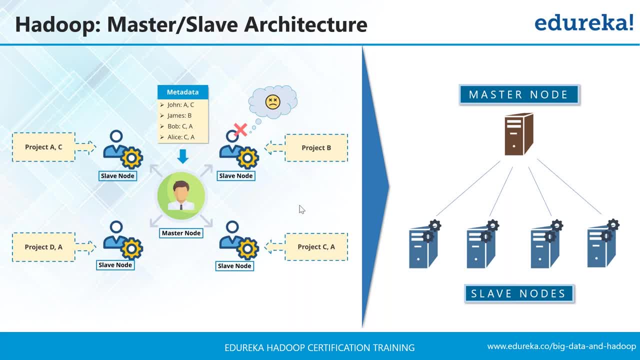 see the same scenario, right? is it only file system? only file system as in box? is it its user? rather, you remove from the account? is it only file system data? so yes, it does. it's like hadoop understand everything in terms of file. it's just a file system. it's not a database. it's not a database. guys. if you say that you want to have the concept of primary key, foreign key or things like that, that is not going to work. 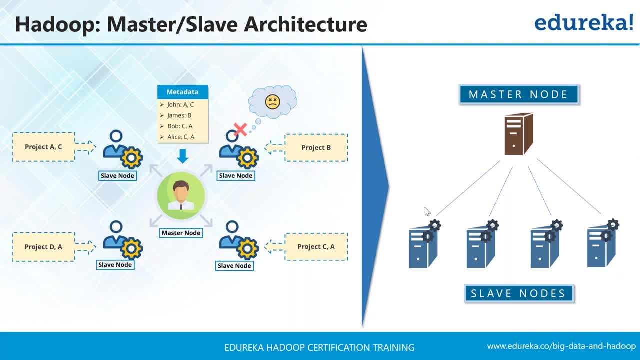 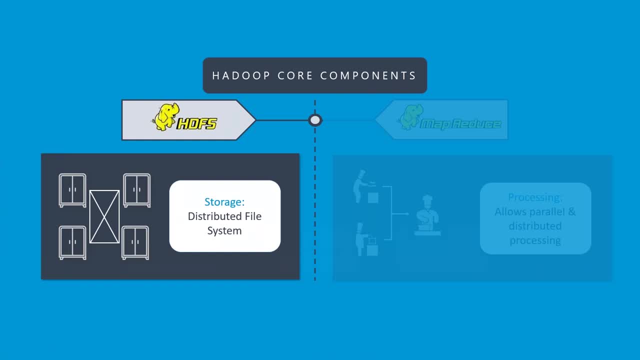 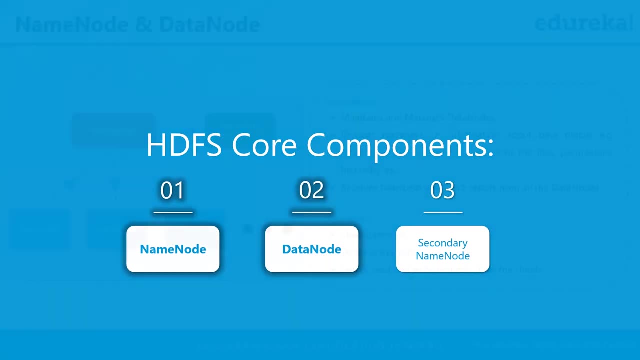 a file system. that's why we do not say that hadoop is a database, and i think this question was asked by vani as well. right, funny? if i'm not wrong, you had asked right. so how is it different from a database? so this is a difference. here we will be feeding the data in in form of a file. here we will. 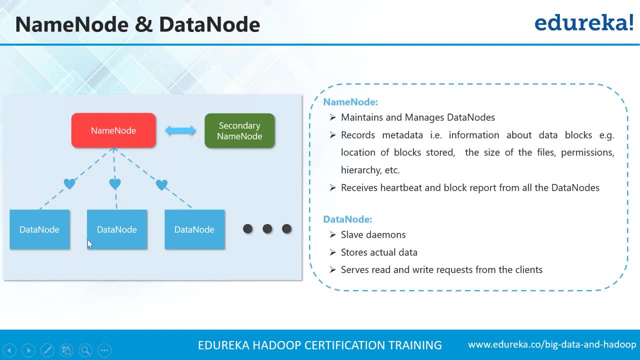 be feeding the data in form of a file and the file will get distributed. that's why we say that it's not a database and on the file you cannot have constraints like primary key, foreign key or things like that. right, okay, so yeah, hdfs. so, guys, when it comes to the hadoop distributed file system, 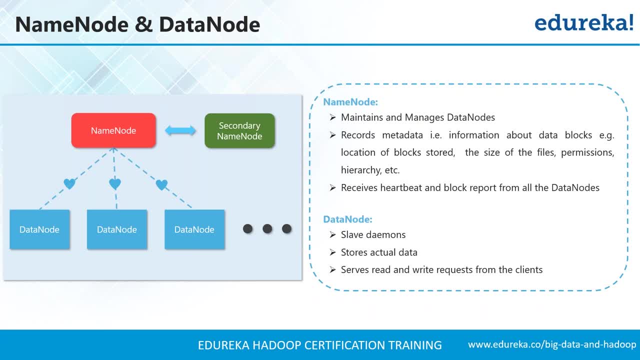 so basically, we do have a master slave architecture. master is nothing but a name node. okay, it's like manager and the slaves are nothing but the data node. so why are we calling it as a master? because it will, or why are we calling it as a manager? because it will just have the metadata and 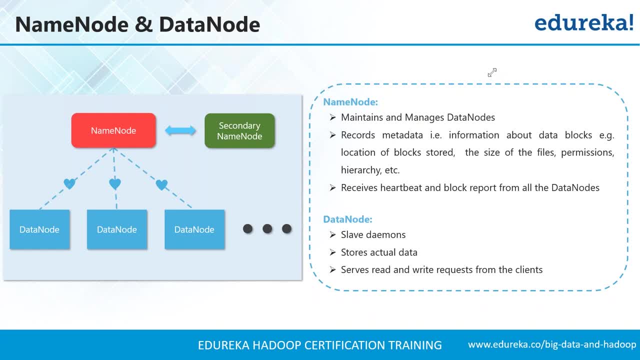 data nodes will have the actual data, so like we will always be sending the status email to our manager saying that this is the status, right? so manager is just having the metadata, but the detailed information like what we are working in our project or on what uses, like what work we are doing, right? so that is, that is the information. 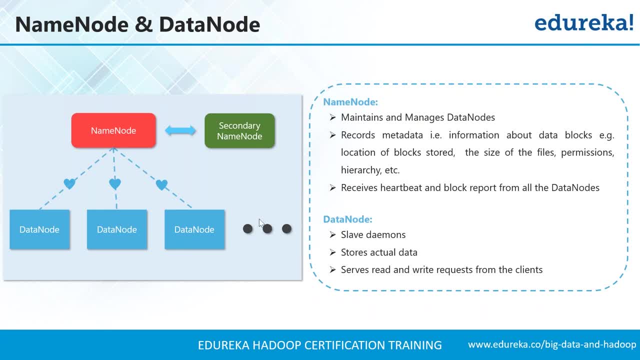 which we have right, right. so, yeah, this is the concept, this, this heart, this hearts. you see, right, so, these are nothing but the heartbeat. heartbeat doesn't sending the status email to them, manager, saying that, hey, i'm there in office and i'm working from home, and this, this, this is the. 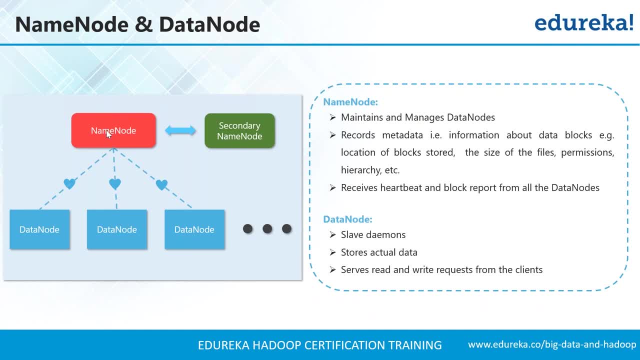 work which i'll be doing today, or this is the work which i have done in the day, or things like that. right, it's like sending the status to the manager. so the point is the day when you do not send a status email to your manager, the day when you do not send a status email to your manager. 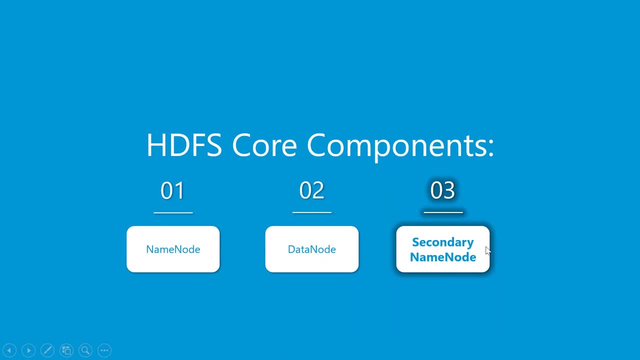 manager will say that, okay, hey, this guy is not working or something is wrong, right, and then manager will be taking the action accordingly. then manager will be taking the action accordingly, fine, okay. so, when it comes to okay, so this candy node is something which is optional, but, guys, one thing: 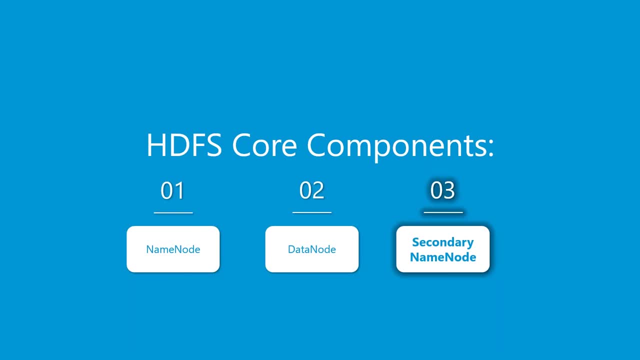 okay, uh, by looking at the name, just don't think that it is a backup. it's not a backup, it's just assisting the manager. it's just a helper to the name node, it's not the backup. so, when it comes to the backup of the name node, we will have high availability implemented. 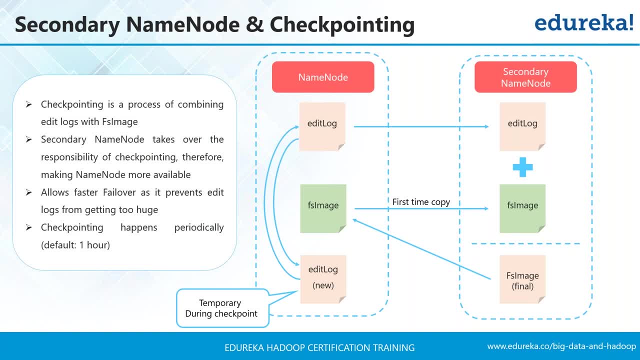 so, when it comes to the backup, what we will have, we will have high availability implemented, where we will say that, uh, we will have two name nodes in the active- passive configuration: one will be active and another will be passive. okay, this is what we will have, okay. 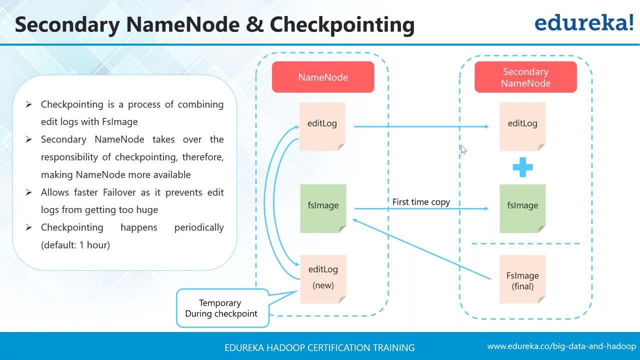 okay. so, guys, it's like i don't think so. there is a need to discuss secondary name node and checkpointing. uh, i think we have other important topics to discuss as well. so the only thing which you need to understand here from secondary name node perspective is: 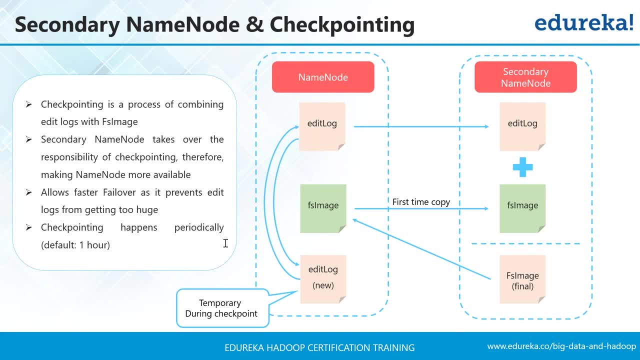 it is optional in hadoop, too, it is not being used, right. that's why i'm saying that we do have other important topics to discuss, but if someone is all, someone is asking about secondary name node, right? so it's like it's just a helper to the name, or it's not? 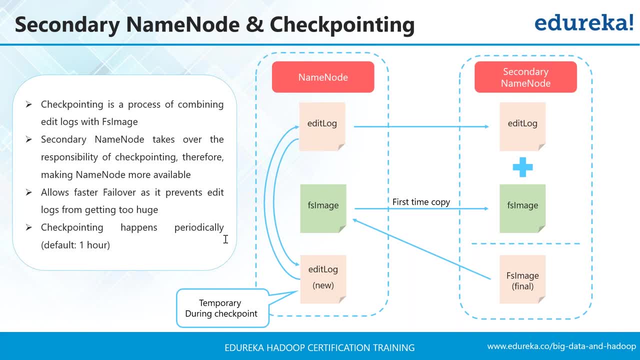 the backup. that is something which you need to keep in your mind always. okay, then we have will secondary name node configured in high availability mode. yes, so it's like when it comes to hadoop 2, right secondary name node is optional, so that is something which you will not be using in hadoop 2, but yes, if you talk from hadoop one perspective. 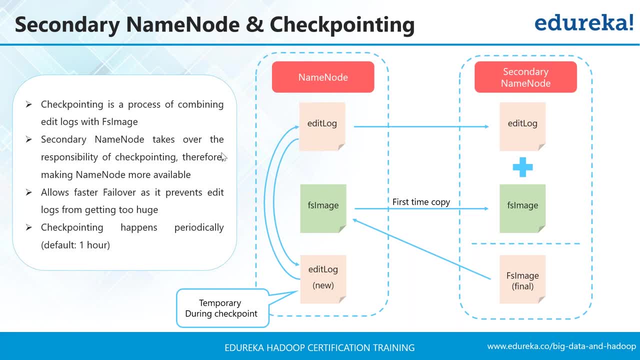 secondary name node is. if you talk from hadoop, one perspective secondary name node is being used, then yes, again, it will be. you know, we'll have a backup for this as well. before that, i have a question. um, sorry, every time the data is changed due to processing, it will. 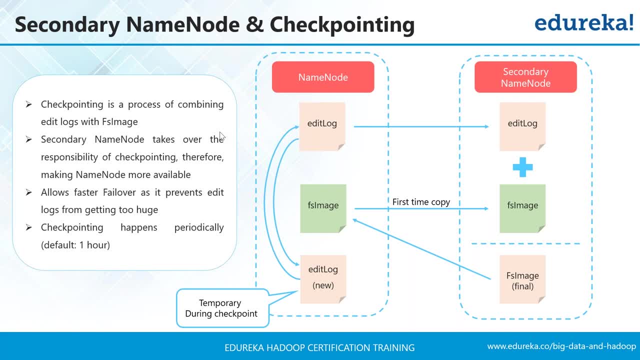 be have to copy twice, so won't this be very slow overall? no, no, it's like the point is. here we are dealing with big data, so if you look at the end result right, it is 100 times faster than the traditional systems. okay, so here it's like what we say. we say that hadoop is 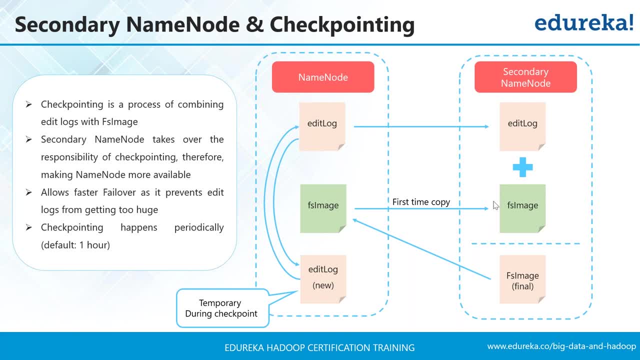 designed specifically for big data. we do not say that it is for small data. if you are processing small set of data using hadoop, it will be taking much more time than the traditional system. but because it is designed for big data, and if you are processing big data using hadoop, 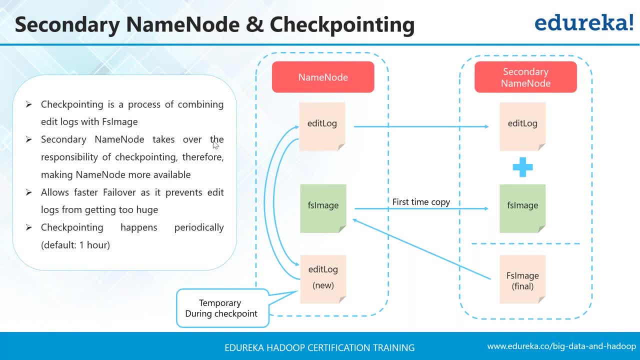 it is 100 times faster than traditional system. i had a question here regarding csv. i saw that question and i think i missed that. so one of you had asked the question regarding csv. oh yeah, it was srikumar. so he says: say you load a csv, it gets split into different. 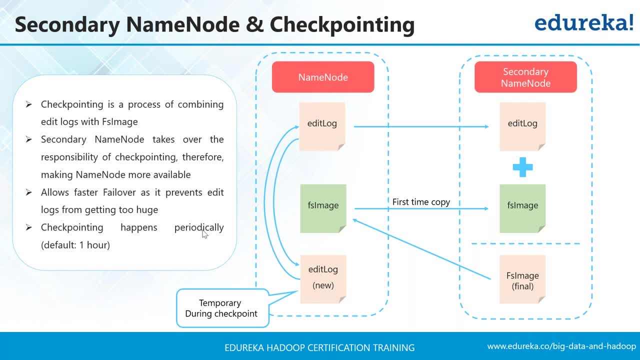 csv and stored in the different node. yes, srikumar, yes, that that's how it works, okay. yeah, okay. so if one one server goes down, what happens to the master file? so it's like everything is being handled by hadoop framework internally. you, as a developer, don't need to worry about it. you won't even get the idea that something. 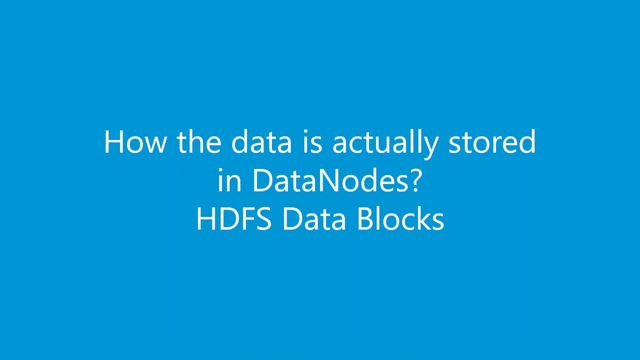 has happened internally. that's why i'm saying that you need to get the understanding of this framework, like how things are working internally. okay, well, that's what i said. secondary name node and name node are not the backup of each other. so canry, nameNode and nameNode are not the backup. 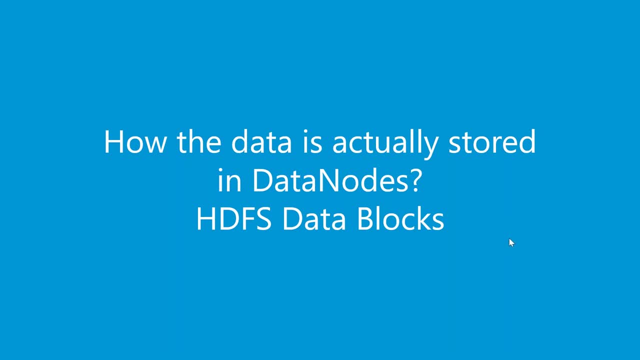 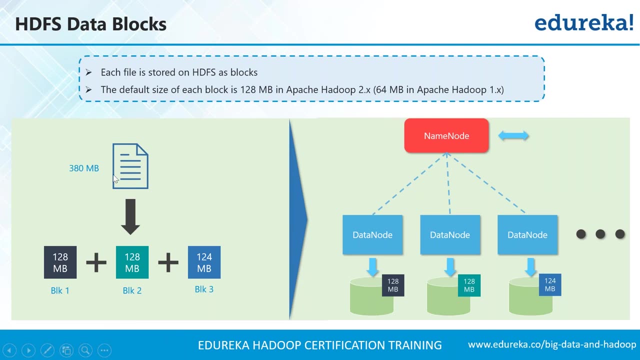 okay, well, that's what i said. secondary name node and nameNode are not the backup of each other. so candy name node is just the helper. so do you think that housekeeper can become the master or the owner? no right. so same thing, it's just the helper for a name node. we will have a complete. 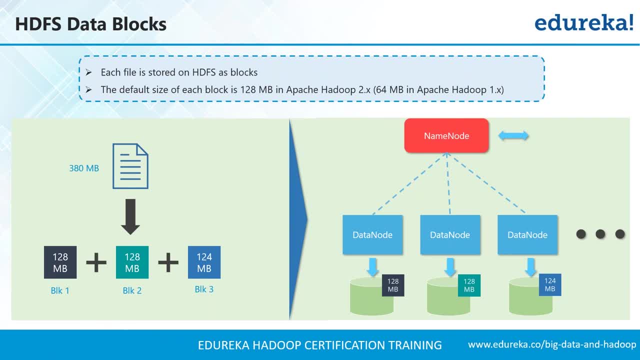 backup or a mirror copy and we will say that these are in the active passive configuration. okay, so, yeah, let's move on to how the data gets stored. so, guys, here is your file. okay, so let's say that you do have a csv file. doesn't matter if you have a csv file or if you. 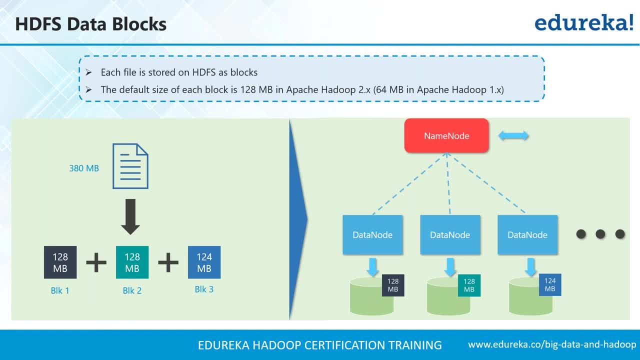 do have an audio file or a video file or you have an image. doesn't matter what you have or what you are storing in hadoop. so that's why we say that hadoop is meant for storing varieties of data. that's why we are saying that hadoop is meant for storing varieties of data. 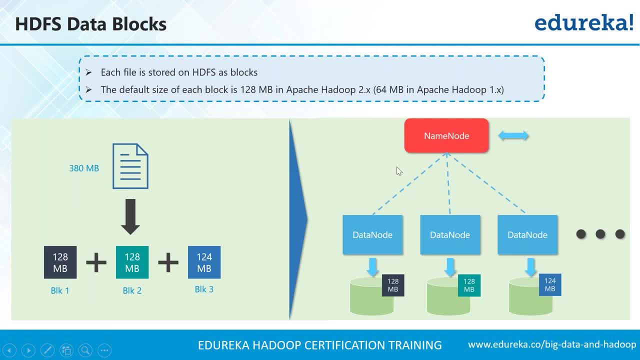 okay. so yeah, here, what do you see you have? let's say that you have this file, which is of 380 MB, so parts of this file will get created, so maximum size of each part can be 128 MB. so what is happening here? it's like 380 MB divided by 128 MB. so three parts got created. now you see, 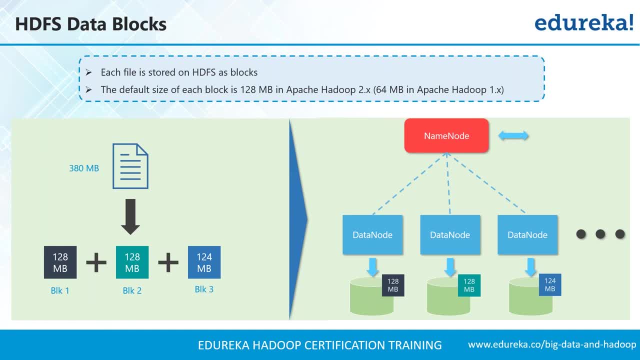 one part is going on one machine, another part is another machine and this is how the distribution is happening. but you as a user have to separate the two parts and if you have a file with a lot of developer will not be doing this. this is not your job. your job is just to give the file to hadoop. 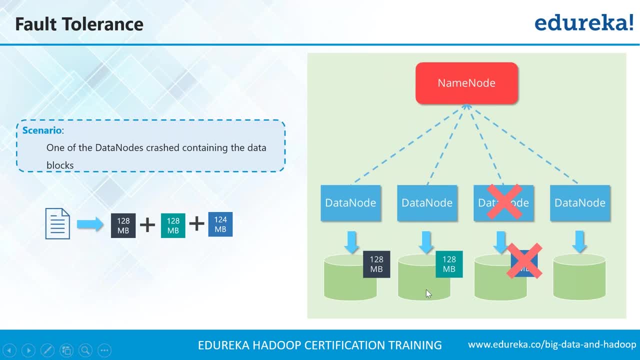 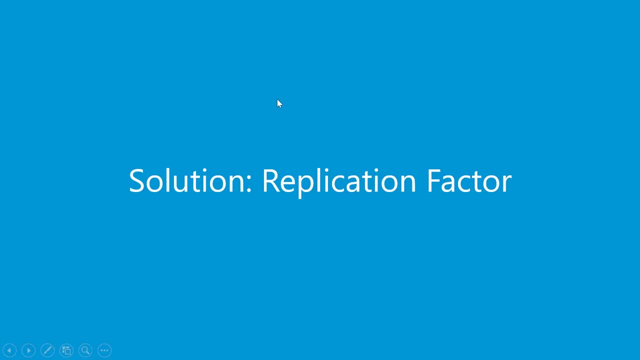 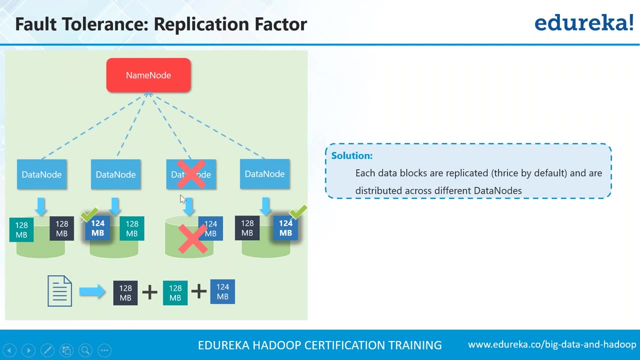 and internally, it will do the splitting as well as the distribution. now you see that it is there on the multiple machines right now, the same question which you are, which many of you had asked: so what if, now that we had distributed the data? so what if it you know, one of the machine? 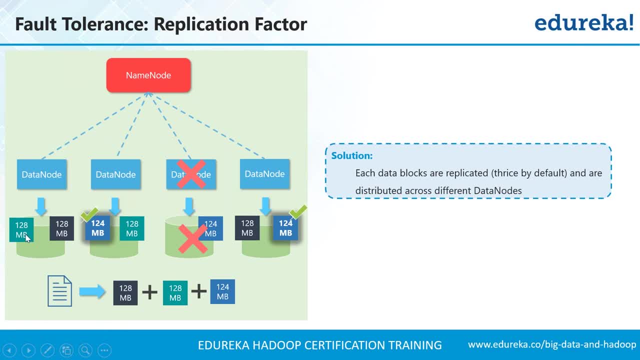 fails, what will happen? the application factor right. so when you were, when hadoop was writing the data or when it was doing the splitting, right what it will do you. you see the application for each block. this for each part. it has that application. this part is present on this machine. 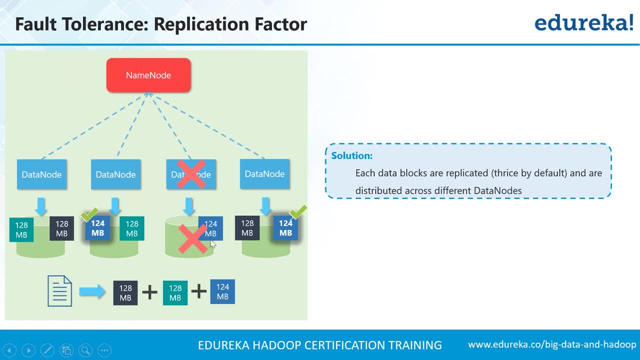 as well. this part is present on this machine as well, right, so now, if this machine goes down, it was having this part. so where is the replica of this part present? it is present on this machine, right? so it it distributes and it replicates the data in in very intelligent manner. okay. 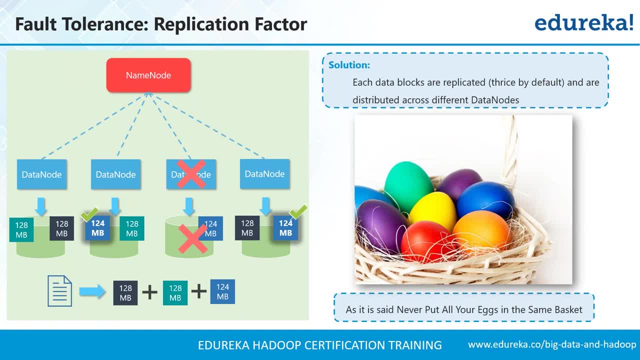 right, so by default, hadoop will be replicating the data three times. it's like if you do have a file of size 100 mb. so basically, if you do have a file of size 100 mb, so what it will be doing it will be creating three replicas, as in 100 into three. so you need 300 mb of play storage. 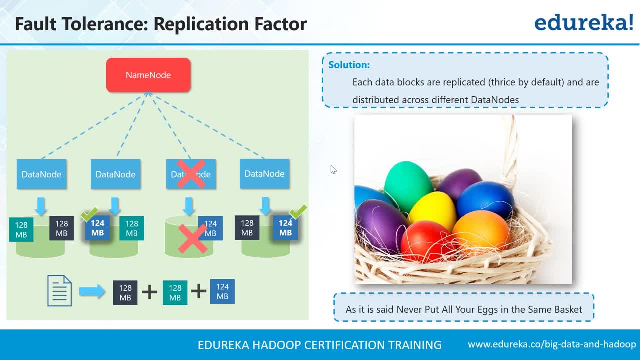 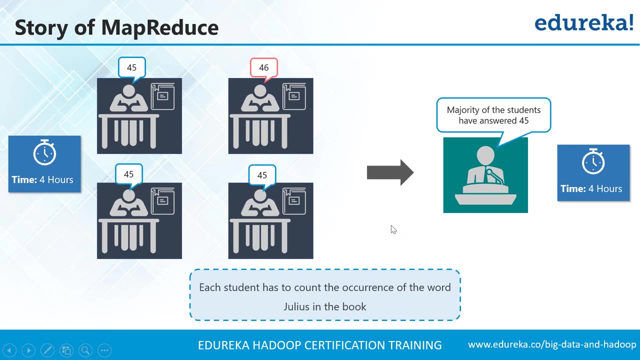 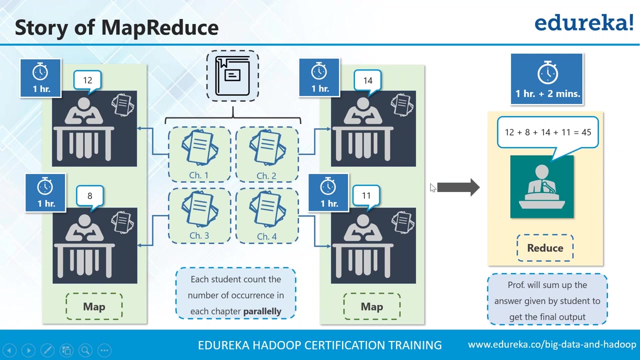 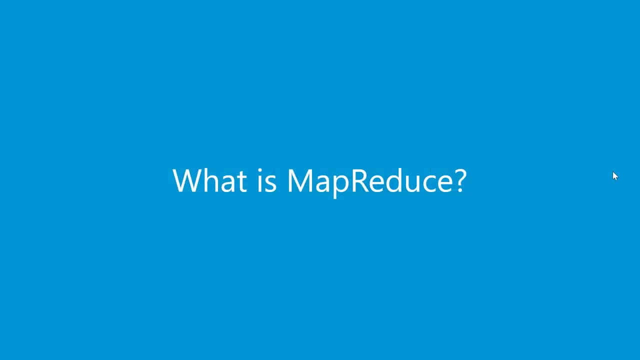 space. what you need? you need 300 mb of storage space. okay, so now it comes to map reduce. it's like parallel processing, right? it's like multiple resources would be running in parallel. so what is map reduce? as in multiple resources would be running in parallel to generate the single output. 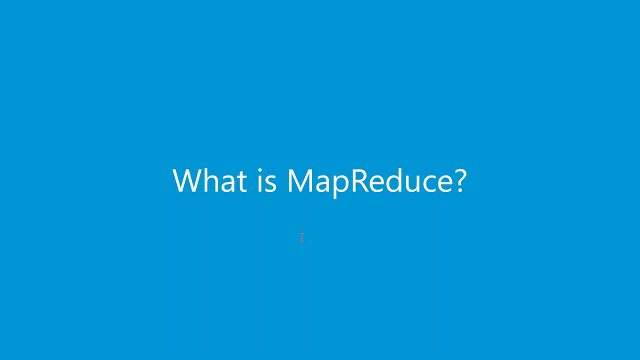 vivek says any specific reason: the size has to be 128 mb. yes, it is the optimized size, but you can change it based on your. usually we don't change it because this is the optimized size, but yes, you can change it. and when you say, how does it keep tracks of replicas? so that's something. 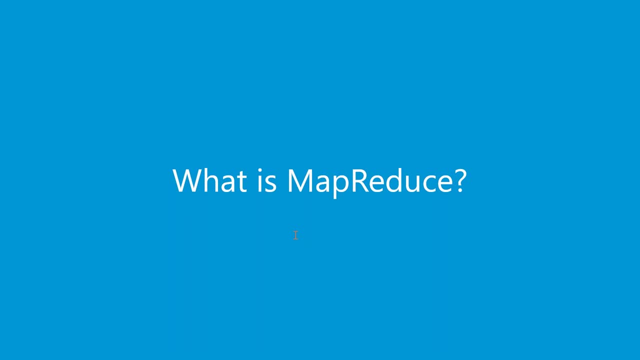 which we cover as part of the architecture and that detailed discussion we are not doing here. so come back. we are underיפne the others website as well and we will be done in theenza terminal in the next fps. so bye, bye, Guys, when it comes to the detailed discussion of HDFS. 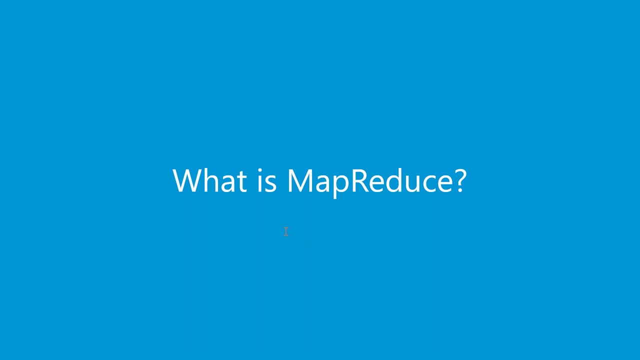 it takes around four to five hours just to discuss how this HDFS works. okay, So that's why I said that we will not be having a detailed discussion, because it's not possible to do that in one and a half hour. Objective of this session is to you know. 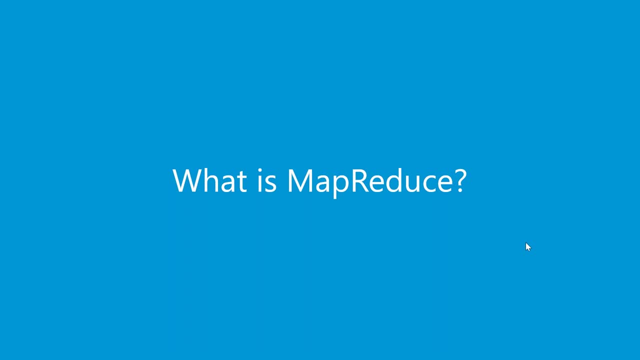 it's basically just a trigger. Now many of you are having a number of questions, So if all the questions are not being answered in this session, I'm pretty sure that you'll use Google or you will have that urge to find the answer right. 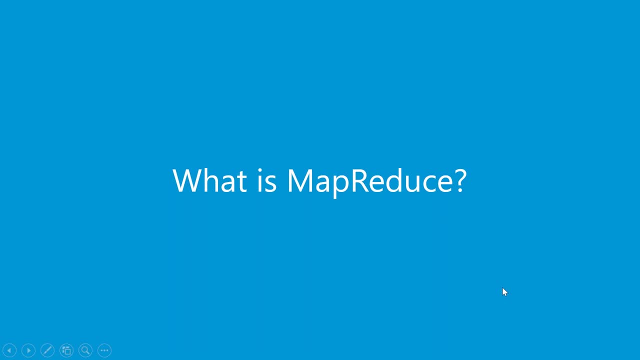 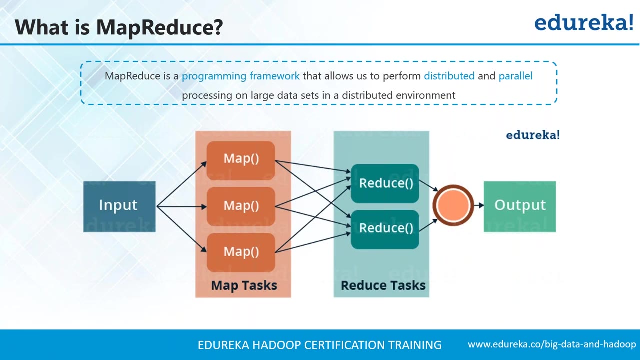 So that's why we say that it's nothing, but it's a trigger, okay, So what is MapReduce, guys? So MapReduce is nothing, but it's a programming framework which allows to perform distributed and parallel processing on large data set and distributed environment, as in. this is our input. 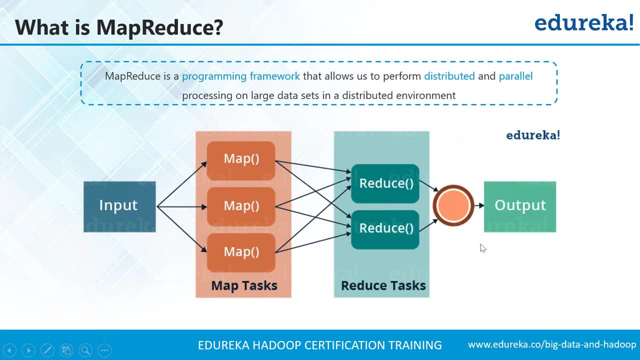 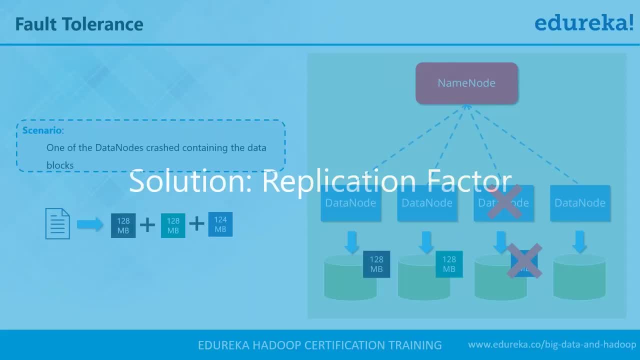 So what do you see here? Internally, this is a machine, right? So what do we discuss? We discuss that your data got distributed to multiple machines, right? So now, when it comes to the processing, this machine has this part. 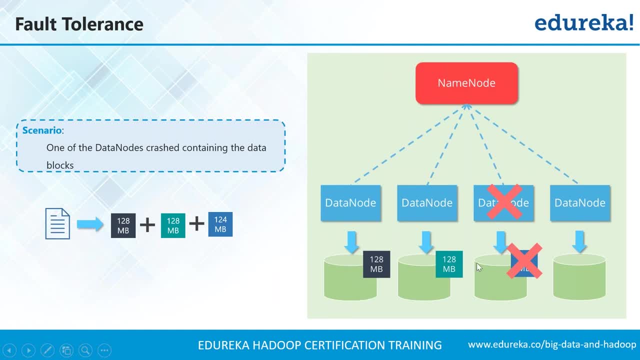 So this machine will be implementing the business logic. Again, this machine will be implementing the business logic, and this machine will be implementing the business logic. So what is this? This is nothing but the concept of parallel processing. This is nothing but the concept of parallel processing. 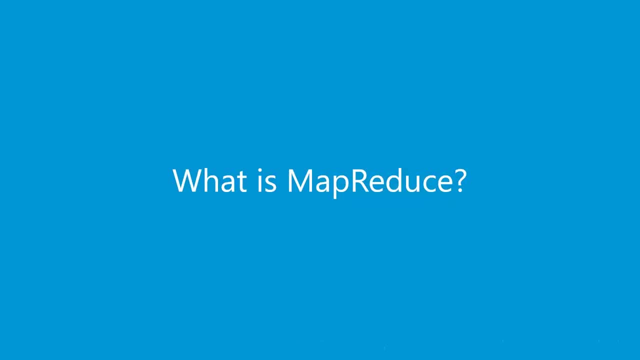 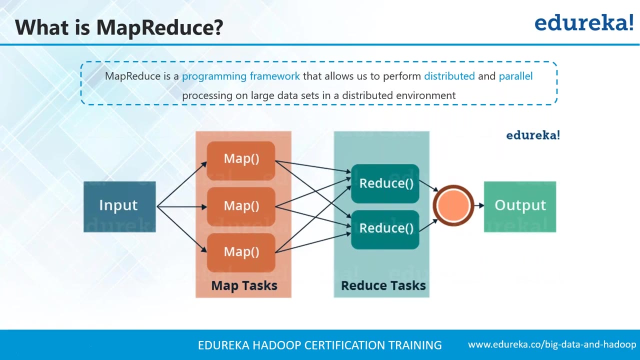 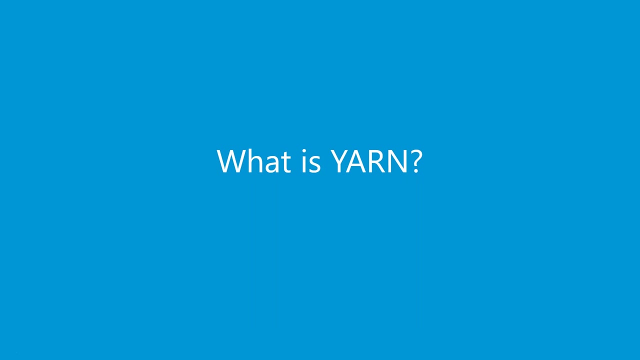 Okay, So yeah, when it comes to reduce, it's like you know, doing the aggregation and serving the end product to the customer. okay, So yeah, what is YARN? So, guys, it's like now because we do have N number of machines running. 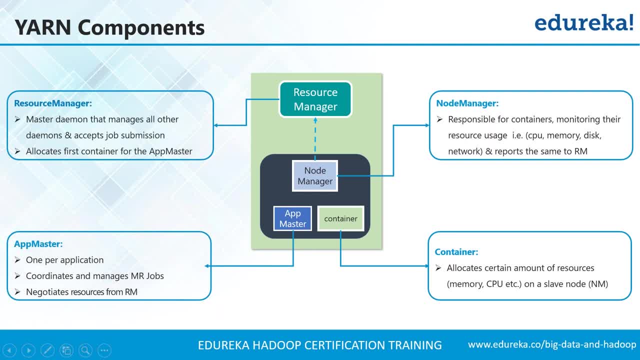 in case of Hadoop, right? So those N number of machines are nothing, but it's a cluster. So what do we have? We do have N number of machines running and that's nothing, but it's a cluster. Okay, So it's like there has to be someone. 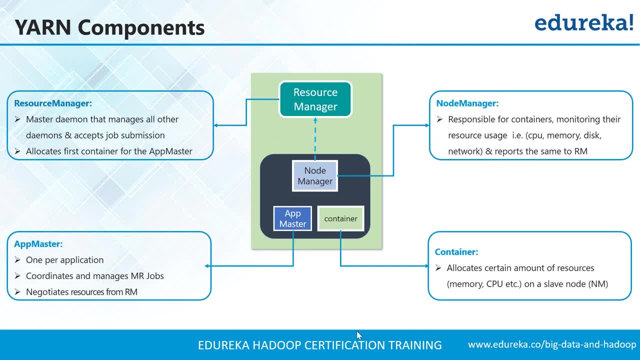 who will be taking care of all the jobs running in that cluster. So what do we have here? We do have YARN. So what is YARN? YARN is nothing but yet another resource negotiator, As in. this is the framework. 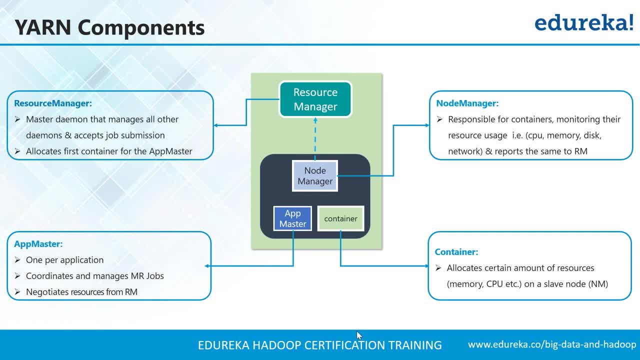 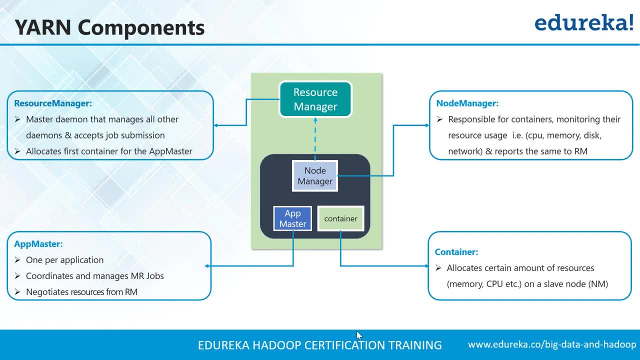 you know, for your job, N number of tasks are running in parallel and for my job again, 100 tasks are running in parallel. So this framework will take care of all the processes running if something fails, or from where to restart, or things like that. 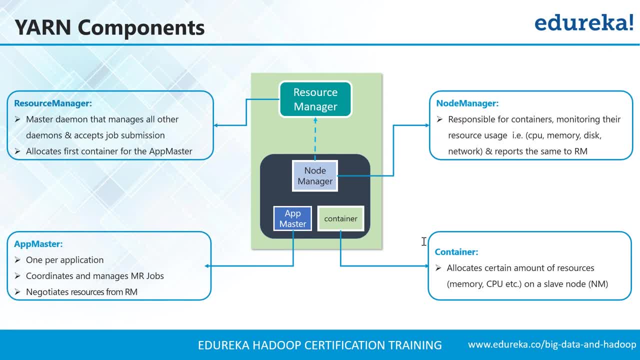 Okay. So what do we have here? We do have yet another resource negotiator which takes care of all the processes running in the cluster. I have a question from Sudesh. Sudesh says how many concurrent jobs I can run and what are the factors as 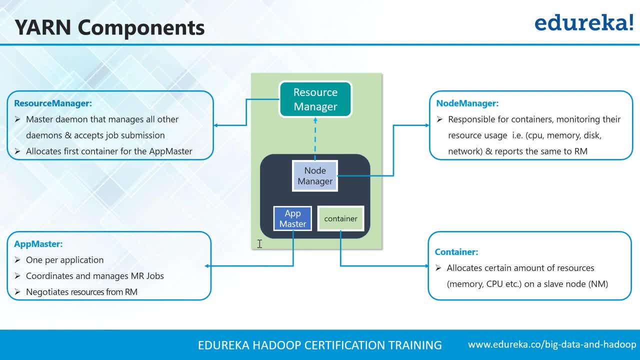 Sudesh, let's understand practically. You do have a limitation for your laptop, right? Let's say that your laptop has got 8 GB of RAM. So what if you use that? you use some kind of application which is consuming more than 8 GB of RAM. 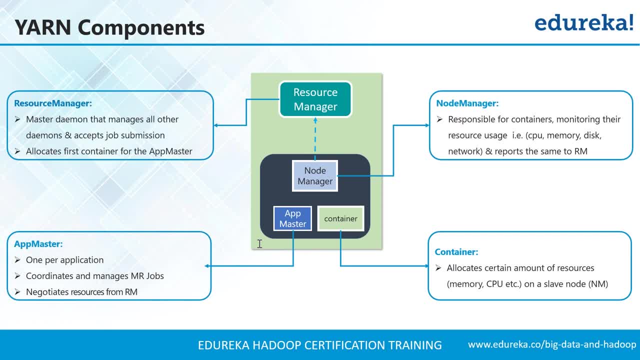 Your laptop will crash. right, Something will happen. So same in the case When you say how many concurrent jobs? that will always depend on your cluster configuration. That will always depend on your hardware specification. Okay, So it will happen. So, guys, once you start working on the Hadoop project. 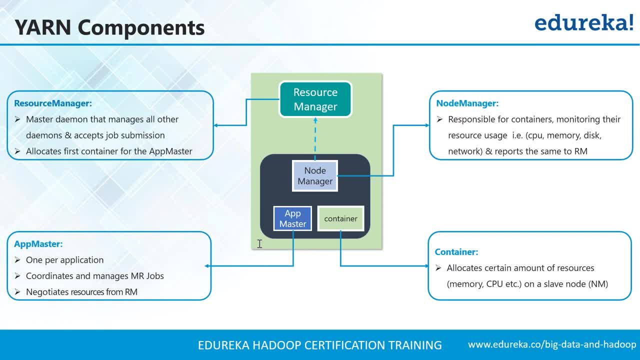 you will get this idea that sometimes, when you say that you know you want to run, sometimes when you say that you want to run more jobs in parallel, then we will say that okay, it's not possible. So what we will have to do is: 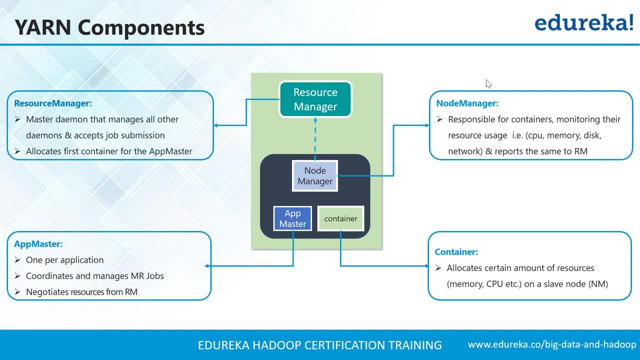 we'll have to increase the cluster configuration. What is the recommended size? Again, Sudesh, this is not fixed. Again, it will depend on the data- Facebook. if Facebook has got more data than my organization, the cluster size for Facebook. 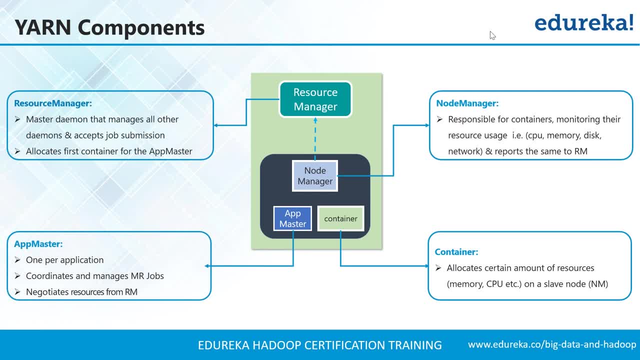 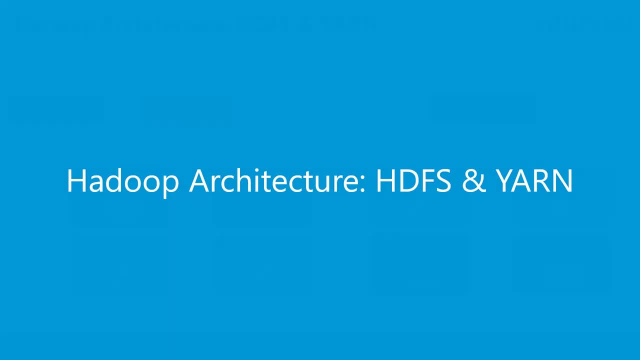 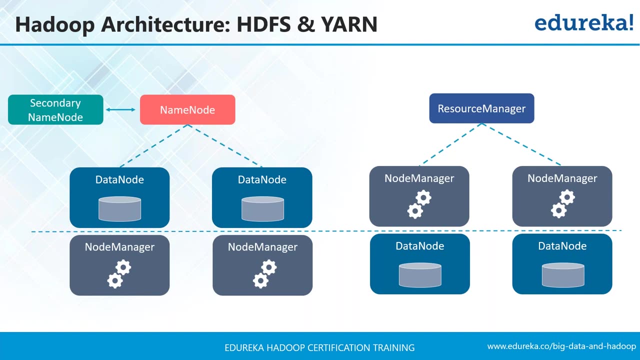 will differ from my organization. Okay, So there is no, some rule as such. It will always depend on your need and the amount of the data or what is your requirement. Okay, So yeah, HDFS and YARN, So it's like YARN is a framework. 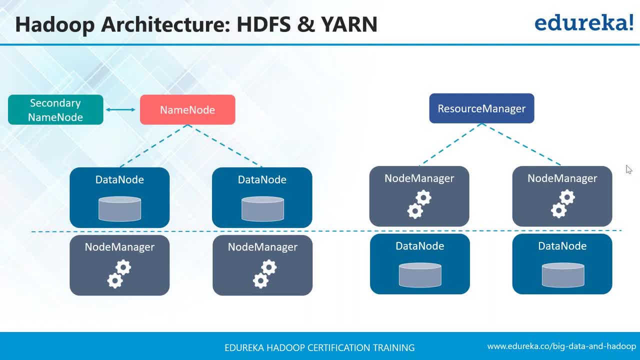 So YARN again will have some background jobs or some daemons running on each of the data node. Does it work in vertical scaling? Horizontal scaling? Sudesh, It doesn't work in vertical scaling mode. So it's like when you have exhausted. 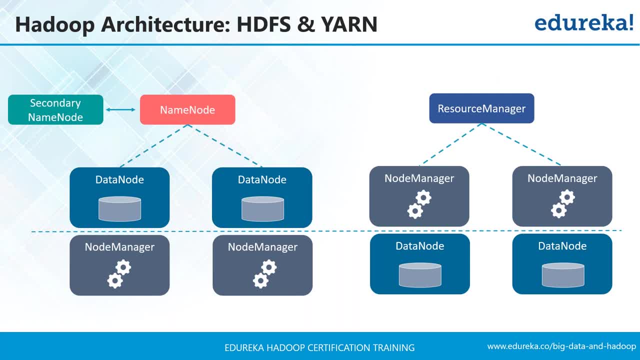 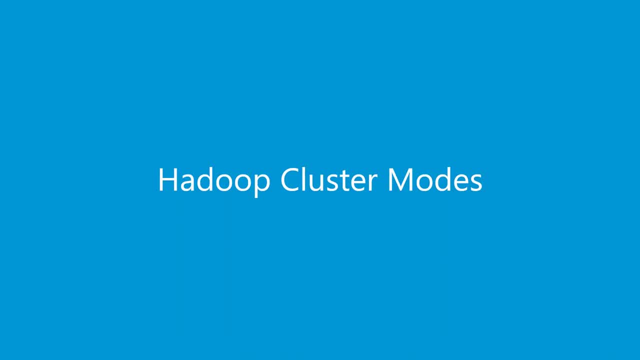 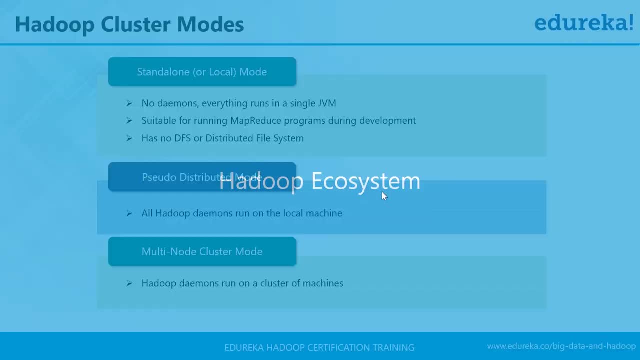 like when you have used all the ports of a particular machine, the only option which you will have there is, like you will have to go for the horizontal scaling mode. Right, Okay, So yeah, Hadoop cluster mode. So, guys, it's like when it comes to the Hadoop cluster modes, 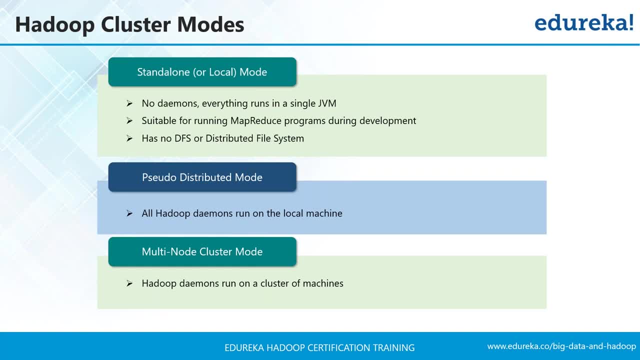 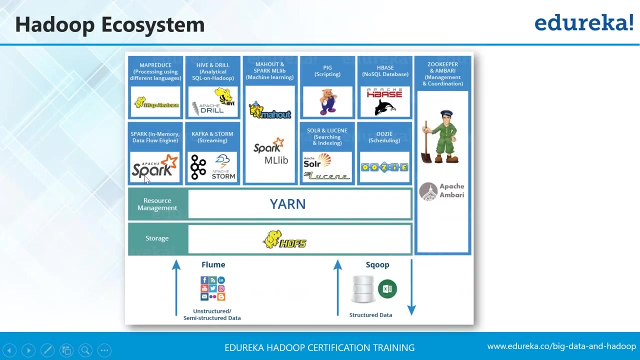 it can run in different, different modes. Okay, So it's like, when it comes to the production environment, it would be. it would be running in the multi-node cluster mode. Like it would be running in the multi-node cluster mode. Okay. 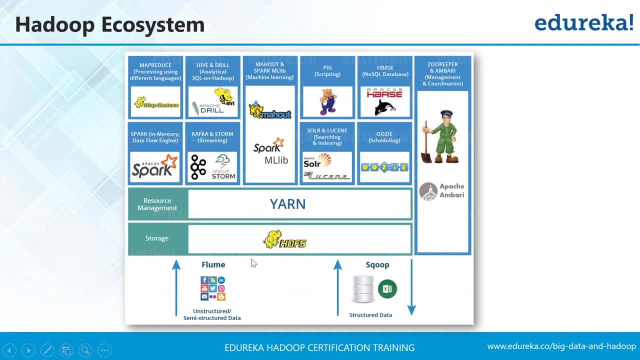 Okay. So, guys, when it comes to the Hadoop ecosystem, you know that HDFS is the base, So it's a storage. Whatever data you have, first of all it has to go here. So now you see, we do have unstructured data. 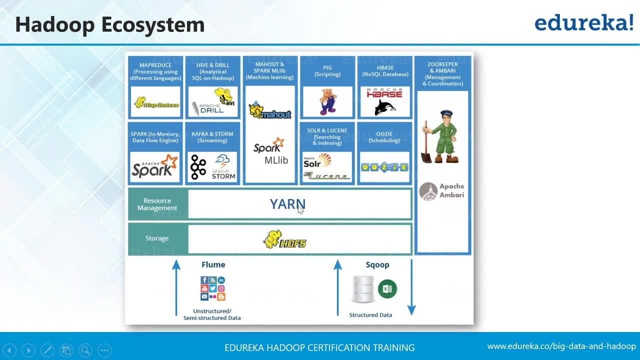 We do have structured data. It has to go here. Then we do have YARN, which is a framework which will be taking care of all the jobs running in the cluster. So these two are the mandatory, you know, or the core components. 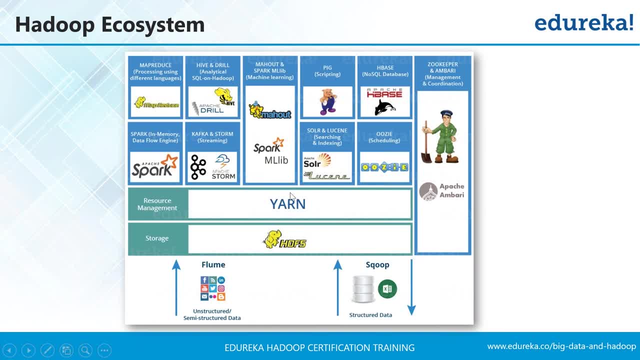 So now for processing. we do have MapReduce. So when it comes to the MapReduce, you need to implement the business. When it comes to the MapReduce, you need to implement the business logic using Java or Python. You can do that. 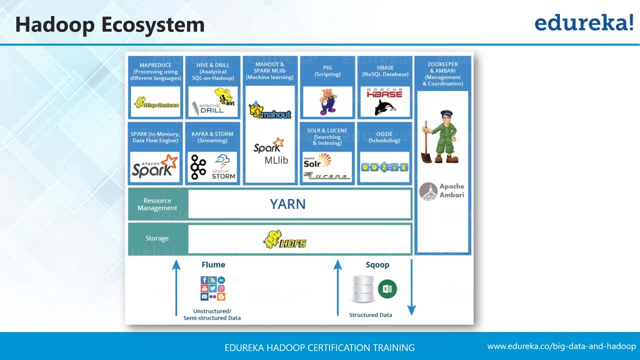 But let's say that you do not come from a programming background And you are saying that, OK, hey, I come from a database background, or I know how to write the optimized SQL query. So tell me, what do I use? right? 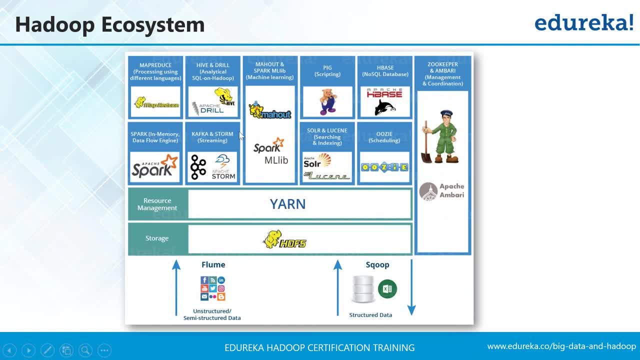 Then we'll say that, hey, you go with Hive, But this Hive internally, it will be talking to the core components and it will be converting your SQL query so that it can be submitted to the processing engine. OK, So this is what it does. 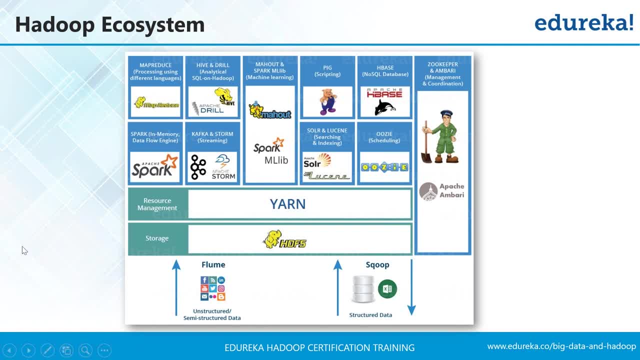 So, when it comes to the ecosystem component, guys, we do have a component using which we'll be doing the migration of the data, using which we can run the SQL queries, or we can run the you know pick scripts we can write, or we do have a NoSQL database. 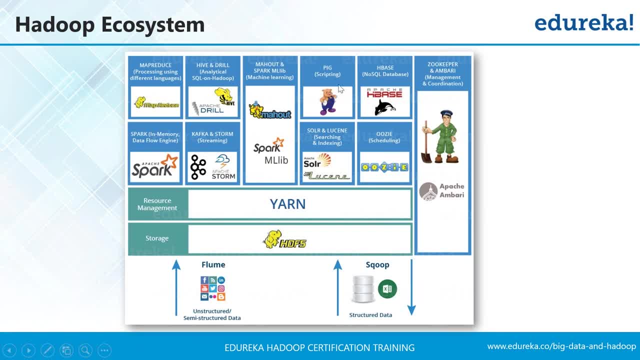 which is edge-based. Then we do have a scheduler which is Uzi, using which we can schedule the jobs, And then we do have Spark and Kafka as well. OK, So, guys, I'm being honest here. Once you enter into this big data domain, 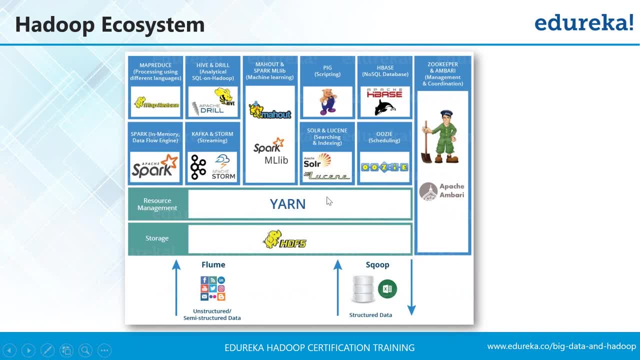 it's like you need to learn n number of things. And one of my project- I worked on Hadoop. Then I move into the Spark project. Then I change the organization Again. I started working on Hadoop because there weren't any need. 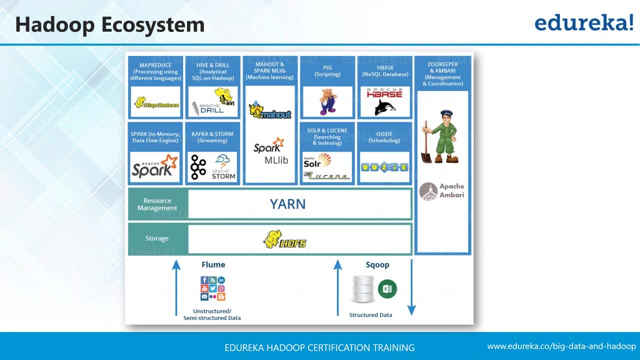 to do the processing on the real-time data. Then again I changed the project. I started working on Azure, where we were writing the Spark or the Hadoop code on Azure right. So it's like once you enter into this big data domain. 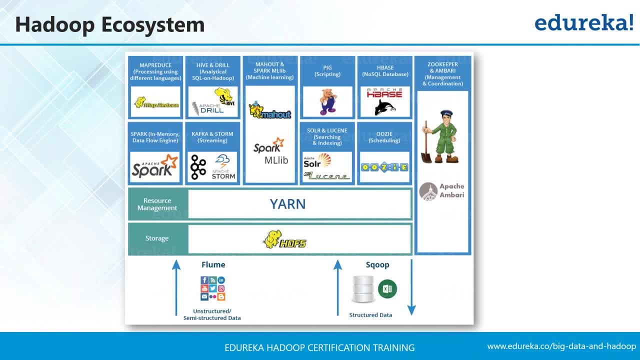 there are n number of things. The other thing is it's like you need to be flexible. So it's like you need to be flexible and you need to have quick learning skills so that you can work on all the components, And always it'll depend on the project need. 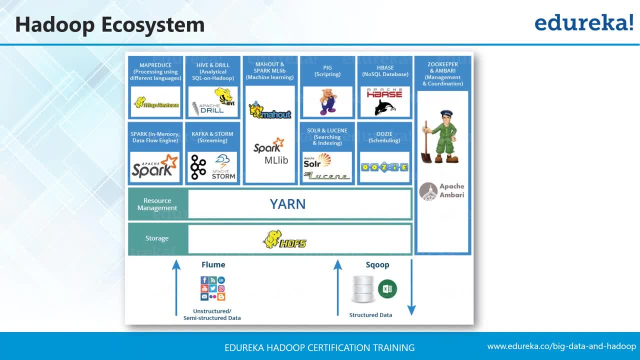 So if you're saying that in your current project you had used Spark or Hadoop, in the next project also, for sure you'll be using that. No, in the next project or in some other organization you can work on HBase, right. 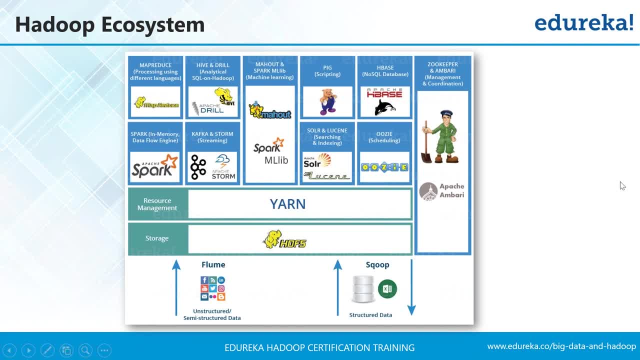 All right, OK, Our question: why HBase, no SQL? Because Hadoop is not a database, Srikumar, because it's a file system and you cannot perform updates on a file system. So if you say that you have a need to perform OLTP, 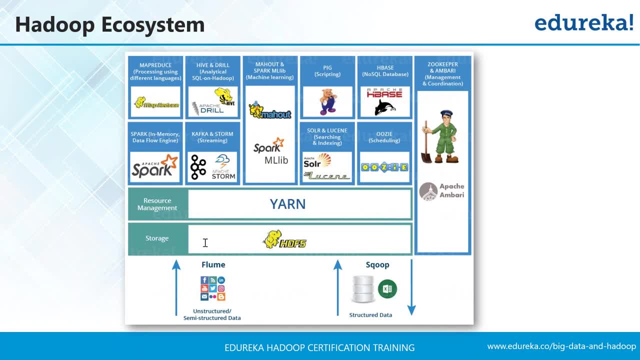 then you need a database. Then, when it comes to Hadoop, what do we have? We do have HBase. Our question from Arti: Guys- I hope I'm audible, Guys, can you hear me? OK, perfect, Sudesh says OK, thank you guys. 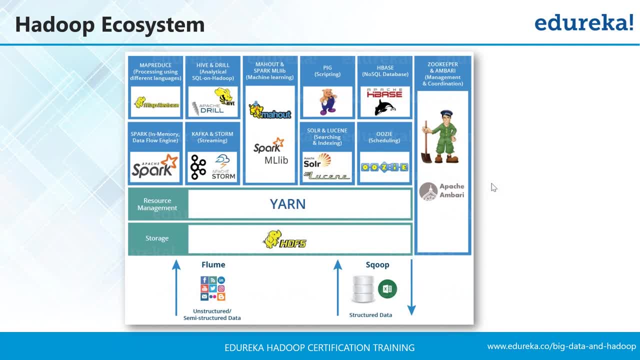 Sudesh was saying that I'm not audible. OK, I have a question from Arti. Arti says: just a quick question: Is it mandatory to have Hanchon on Core Java? No, basic Java is enough, Arti. 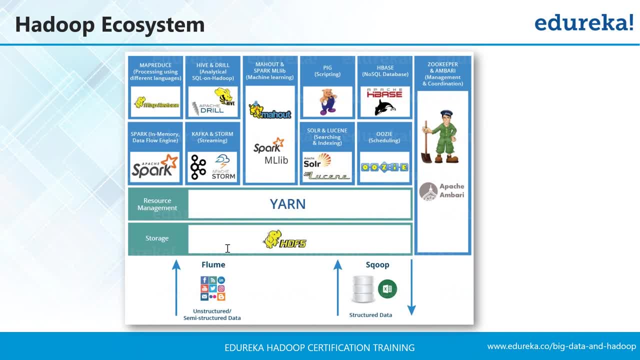 if you want to work on Hadoop and Spark, Basic Java is enough. Kewal says are new projects? still goes with MapReduce or mostly new ones. use the new tools. No, Kewal, it's like if you have a use case. 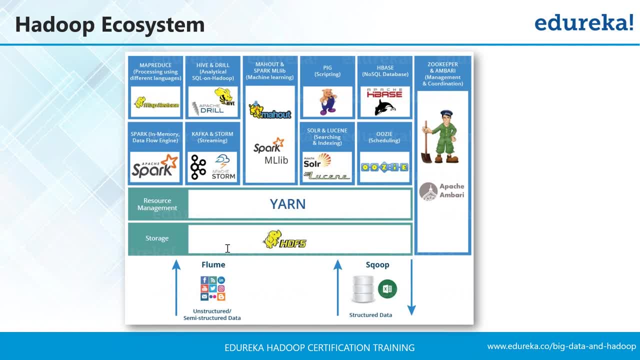 I'll tell you one example. OK, So when you open the Facebook, right. So what do you think? What is the priority for Facebook to you know, to load the profile or to show the friend suggestions? Obviously, it's to load the profile, right. 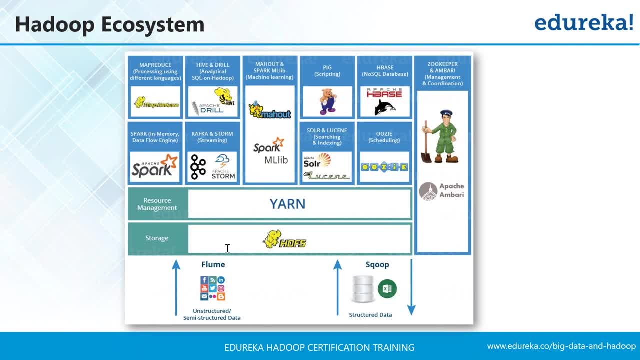 For loading the profile. they need some new tool which is very much fast, right, And to show the friend suggestion. Facebook is saying that, OK, hey, we can show the friend suggestion after five or 10 minutes as well, So they don't need a, you know, high processing system. 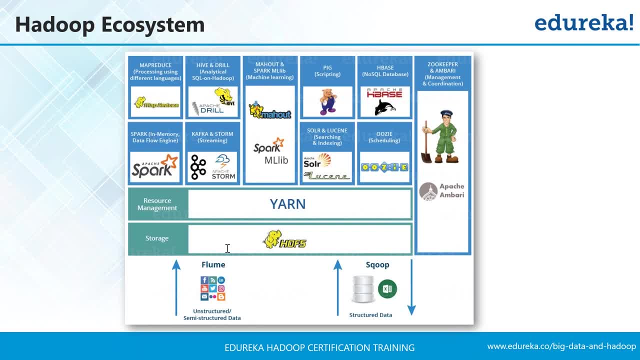 because if we are saying that our objective is to get, or if we are saying that you know, we want to process the jobs at a very high speed, then we will have to invest in similar kind of tool as well. Right, So it will always depend what is their use case. 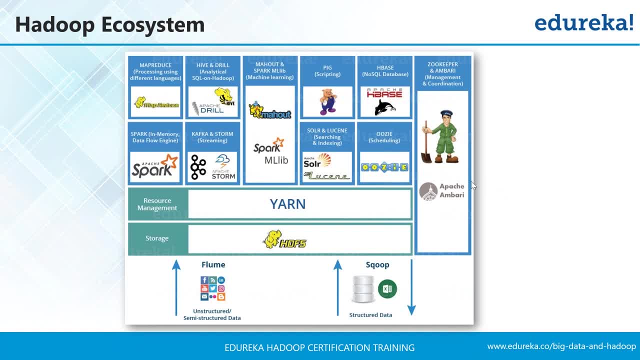 and accordingly they will be going with Hadoop or the new tool. Hive is a database. No, it's not a database. It's not a database but because it is running on top of a file system. That's why we are saying that it's not a database. 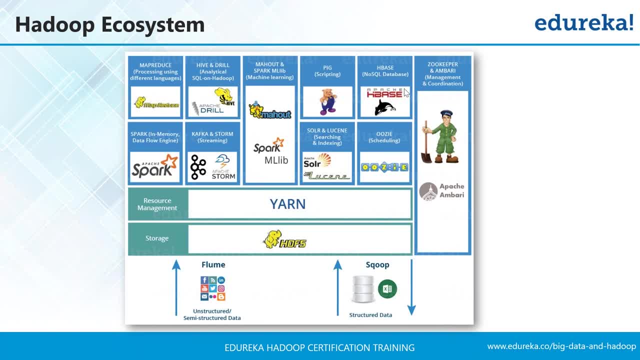 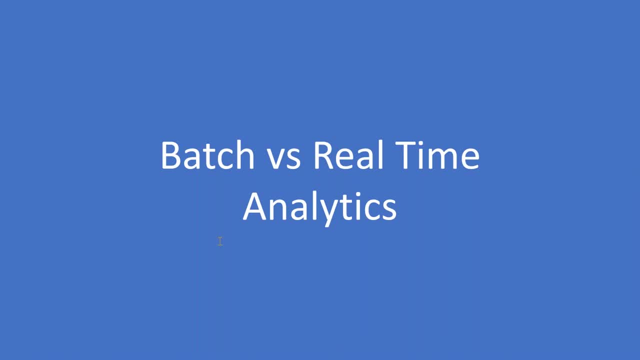 Okay, Okay. so, guys, now let's talk about spark as well. This is what. okay, So, guys, let's understand quickly. So I'm saying that we can run DDL, DML there, Yes, the one we can do, that we can run DML as well. 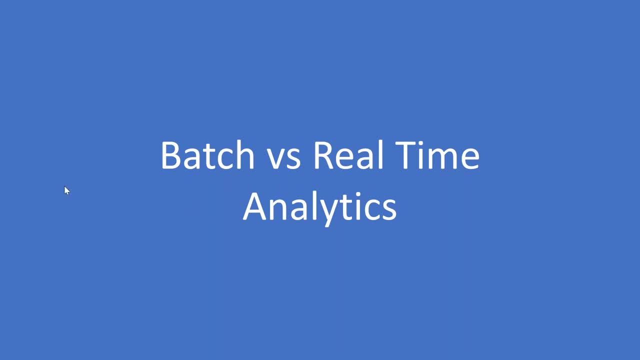 But I think once you start working on it you will understand that in Hive by default will not have updates enabled. So you need to set that injection manager to true and then only will be able to perform the updates. So that's why I'm saying that you know. 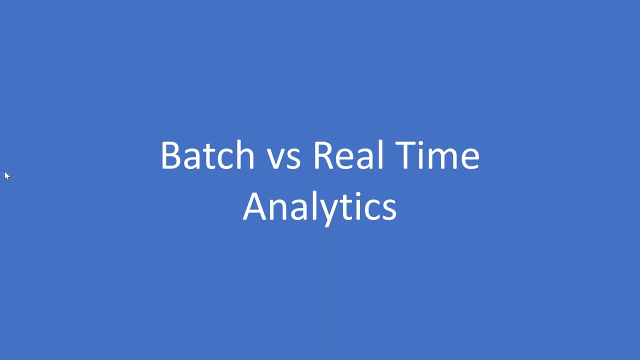 you just need to understand the architecture first, that if it is a file system, then how high was the database? Okay, so, let's go on. Okay, guys, Now we will talk about batch versus real-time analytics. Okay, So, what is this batch data, guys? 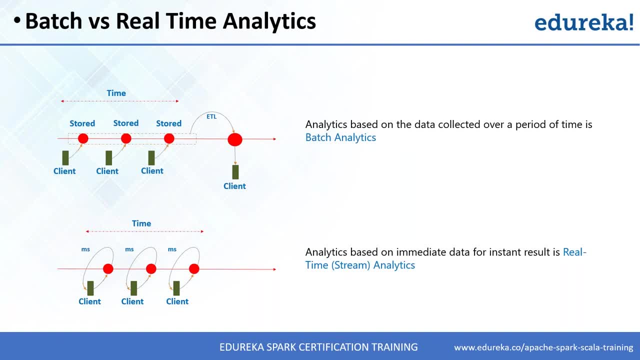 So, basically, it is the data which is coming at regular intervals. Okay, It is the data which is coming at regular intervals as an. I'm saying that, hey. I'm saying that, hey, that every half an hour I'll give you one file. 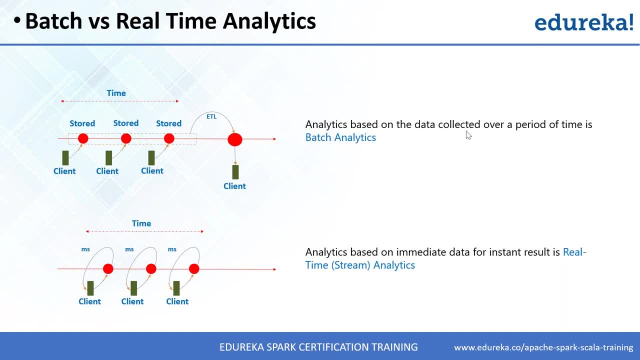 So what you are doing, you are storing the data. Okay, So what you are doing here is it's like you are storing the data. You are getting a file at this time, at this time, So you are storing the data and at the end of the 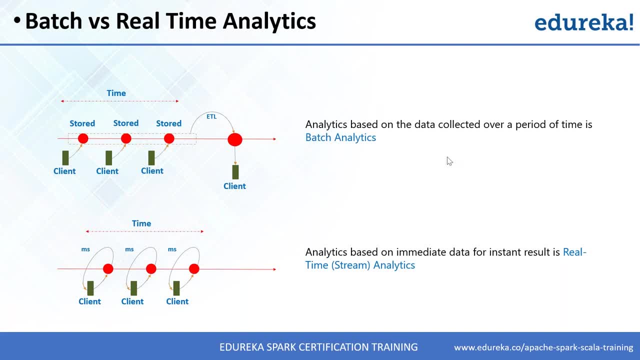 Day you are processing it. Okay, This is what batch analytics is: real-time analytics The moment you get the file, that is a need to process it. So example of real-time analysis: whenever you swipe your card on the pause machine. right, It's like you know these payment gateways, they do have a payment. 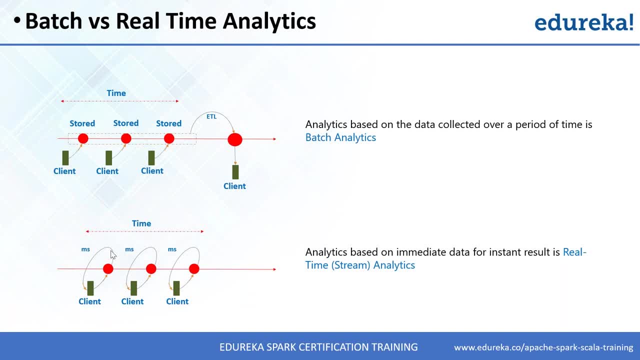 gateways, They do have a SLA of seven seconds. Okay, So within seven seconds you should get the acknowledgement, or you should get the response if the transaction is approved Or if it is rejected. So now, if you think from the payment against Gateway perspective, 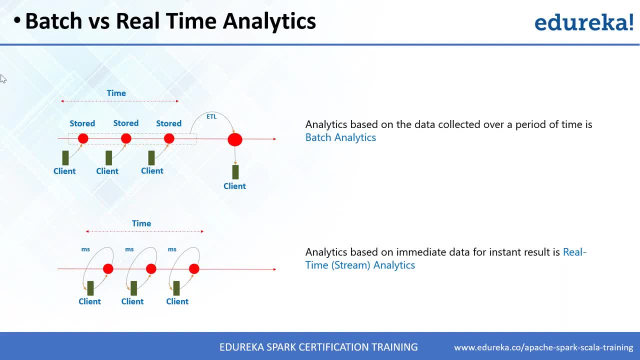 if you think from Visa perspective or from MasterCard perspective, right? So they do have a number of transactions flowing every second or every millisecond, So what they need to do is they need to process it quickly, right? They cannot tolerate this delay, right? 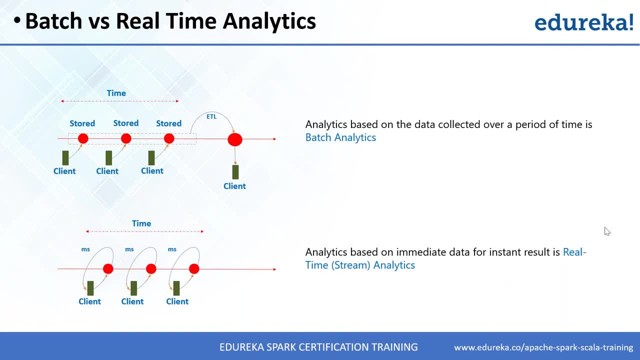 Even right and also it's like they need to run this, they need to run this fraud detection algorithm as well. They need to run this fraud detection algorithm As well, where they say that you know, yes, within seven seconds, we need to process it and we need to run the fraud detection algorithm. 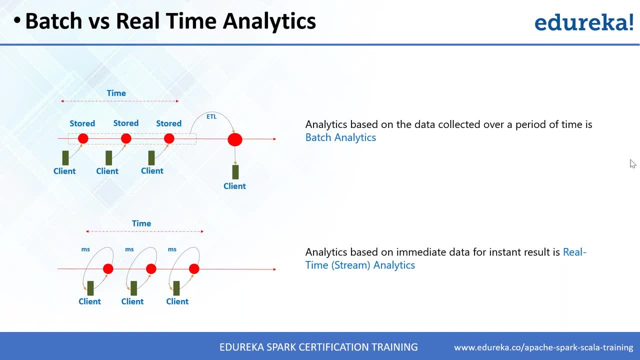 And also it's like, even if there is a delay of millisecond right And if your transaction has entered the payment Gateway, no one can stop it. Okay, Okay. Vani says: is my chart visible? Yes, money, I can see this. 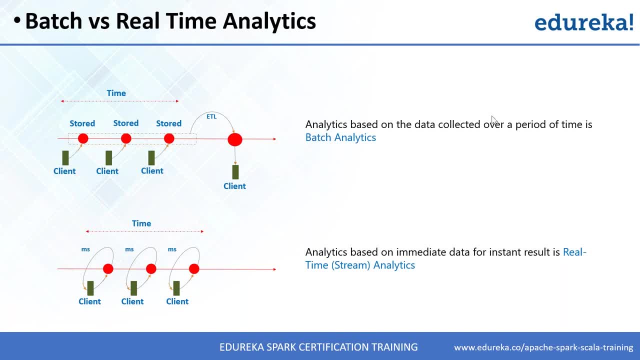 Why did you have any other Questions? Can you give example for employee data And how would MapReduce is done with Hive? I mean the flow. So, Vani, that is not something. So, Vani, it's like we do have more webinar schedules for the detailed. 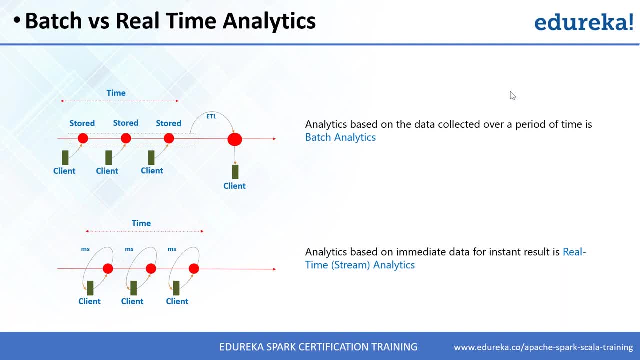 discussion on Hive and PEG. Okay, so it's like schedule is already published, So you look for the webinar which is specifically for Hive and PEG. So there we will be discussing the scenario in detail. Okay, As part of this session. 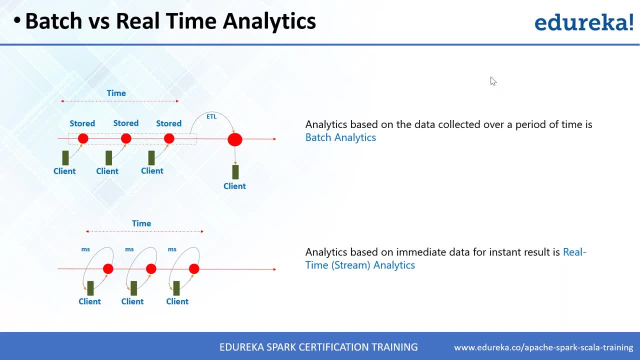 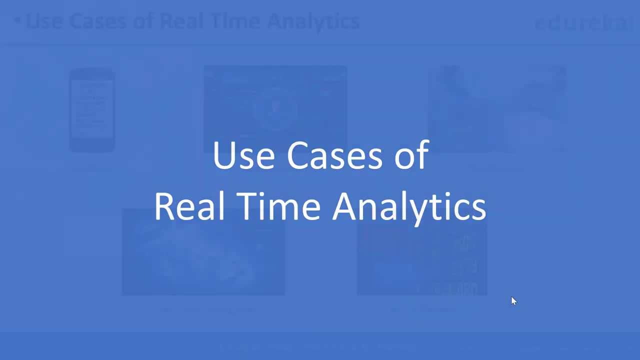 We are not going to do that. So yeah, guys, so this is what the, this is what the difference is between batch and streaming data. So yeah, I've given you the example of real-time analytics already: stock market, banking, telecommunications, healthcare right. 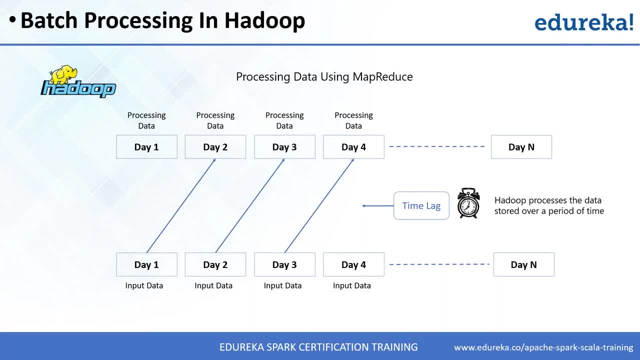 So why is Spark when Hadoop is already there, right? So the point is, guys, when it comes to Hadoop, right, It is designed for doing the analysis on the batch data. Sorry, guys. So when we talk about Hadoop, right. 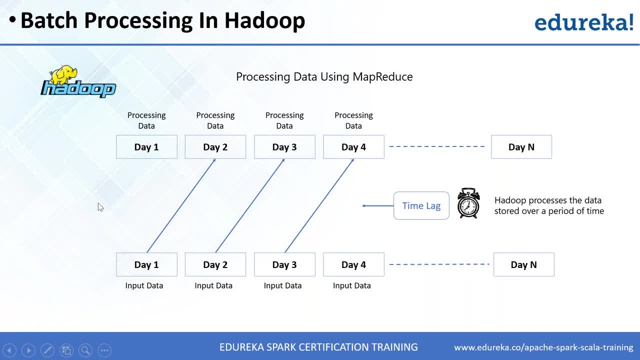 It is designed for doing the analysis on batch data, which is coming at regular intervals, and also it was designed for OLAP: OLAP as an online analytical processing. OLAP as an online analytical processing where you are doing the analysis on the historical data. You are interested in generating some reports. 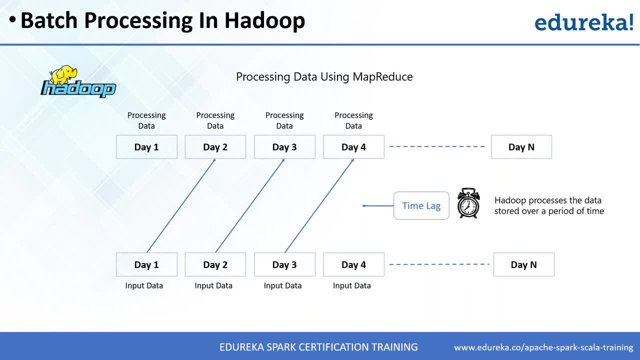 On top of this data. Right, That's, that's what we are saying. So now, when it comes to the spark, right, So it's like we there, there shouldn't be any lag like the moment We are, moment We we get the data. 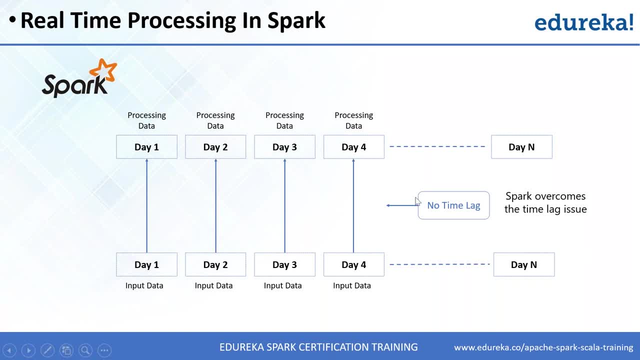 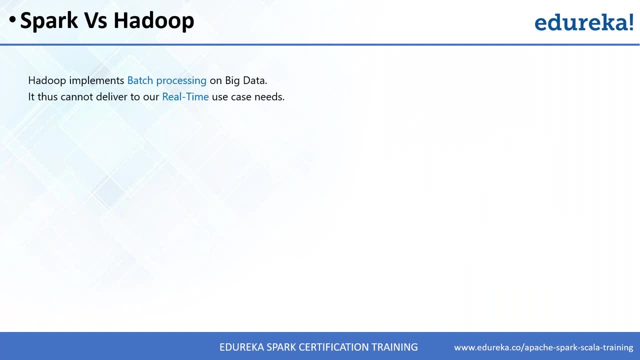 We should be able to process it Right. So spark is designed for real time. So the point is: what is the difference? or how spark is able to process the, the real-time data? So the point is, guys, Look at this, Okay. 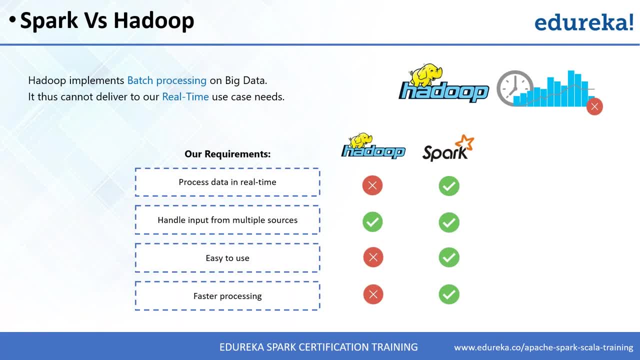 So point is, when it comes to Hadoop's MapReduce, right? So MapReduce is always working on the disk as a reading and writing will happen to and from the disk, and when it comes to, when it comes to, spark water does what it does. 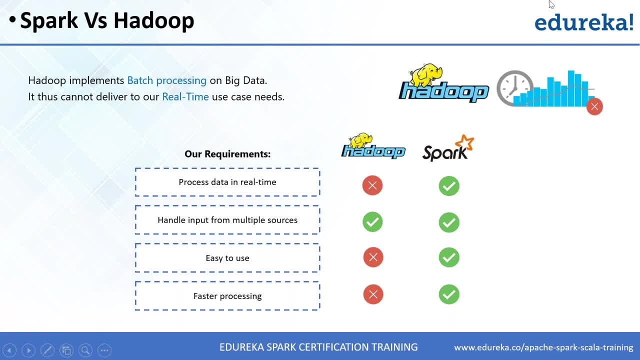 It does the reading and the writing in the memory. what it does? It does the reading and the writing in the memory. Okay, this is, this is what it does. So now, if you want to process the data In real time, you should be using spark. 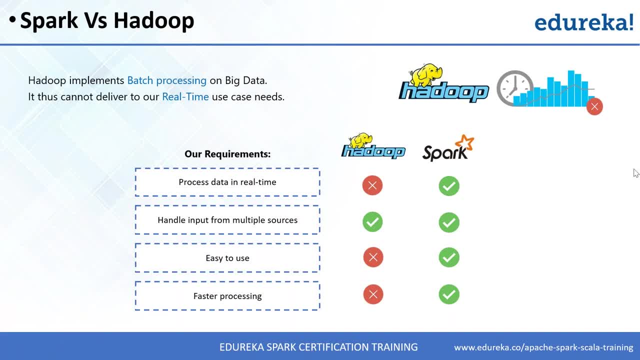 If you want to handle the input data from multiple sources, you can go with Hadoop as well as from, as well as spark. What is more easier to use spark? So point is, when it comes to Hadoop, MapReduce, right, You need to write a complex MapReduce program. 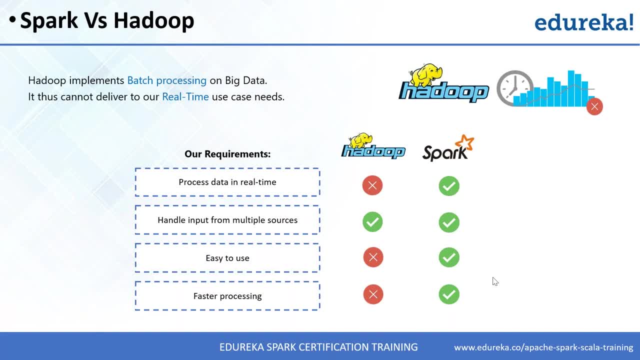 Okay, and if you look from implementation perspective, in spark we can use Scala as well instead of Java, and Scala is a higher level programming language. So basically, if in Java you are writing 100 lines of code, if you are writing 100 lines of code, you in spark. 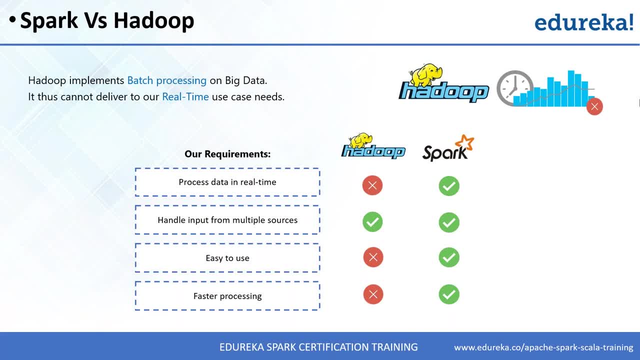 you will hardly be writing 10 or 15 lines of code. Okay, and spark is for faster processing. I have a question here: Apache Kafka comes under Hadoop or spark. It comes under spark Kumar. So spark is also a framework. Yes, Vani, spark is also a framework. 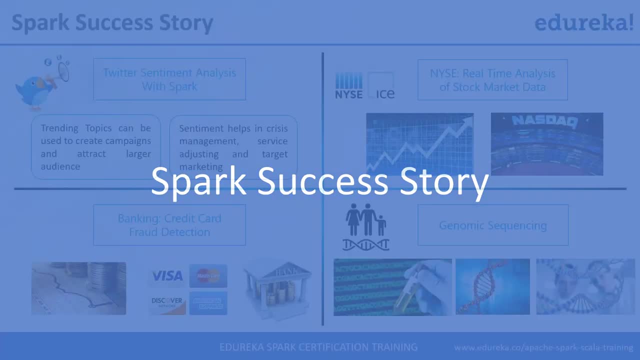 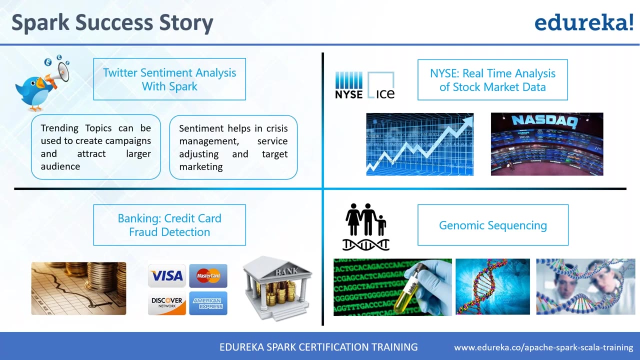 Okay, spark success story. It's like you know, wherever you see the real-time Analytics, most of the time It is it is happening using spark. Okay, most of the time it is happening using spark. Can we use both at a time? 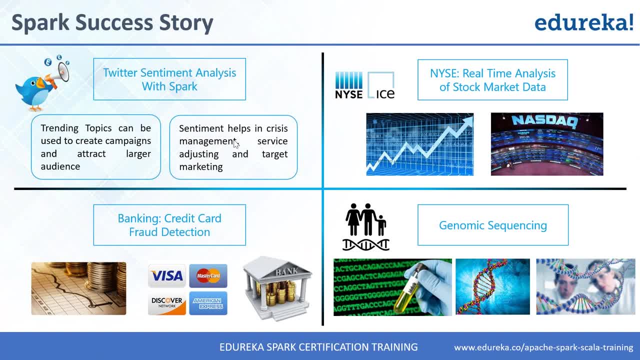 Vani, I took the example of Facebook right, where I said that you know, priority for Facebook is to load the profile, then to show the friend suggestions. now for one feature: for showing the friend suggestion, Facebook is using MapReduce because it is less expensive, but to load the profile, Facebook is using spark. 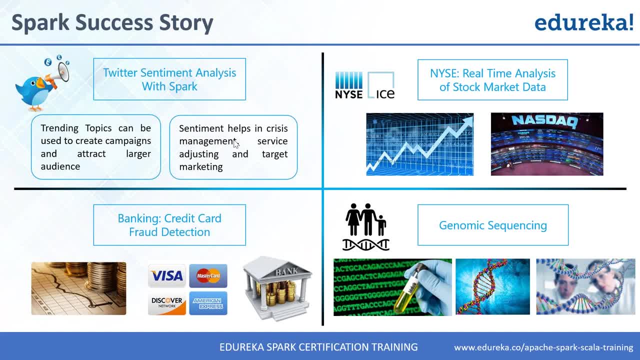 So for each and every feature, right. So we'll be say we'll be saying that, okay, for this feature, data should go here So we can do that Are? this is what exactly is Kafka. Kafka is nothing, but it's a messaging queue which we use, which we use to collect real-time. 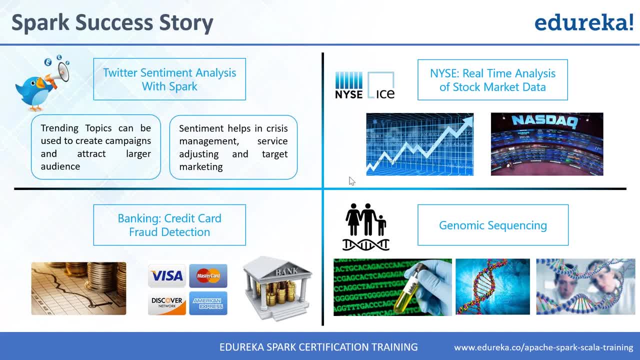 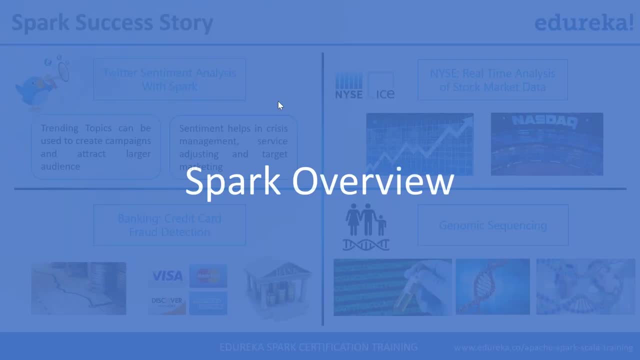 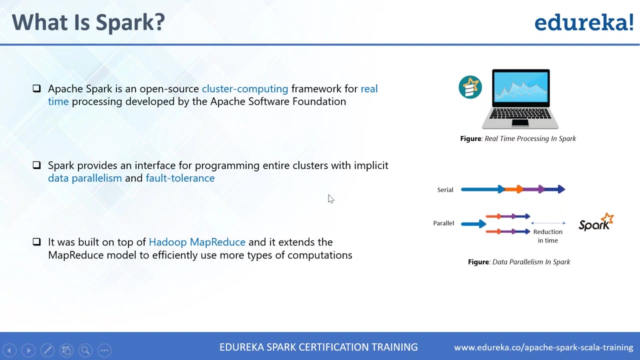 data, So we'll talk about that as well, actually, Okay, Okay. so let's move on. Okay. so spark, wherever you see the real-time analytics that's happening using spark. So spark overview, guys. Okay. So it's like: again, it is a framework. 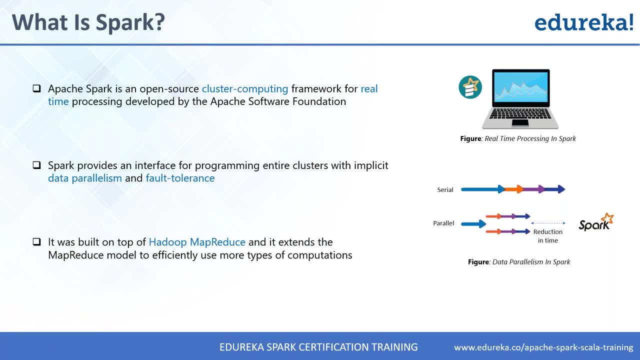 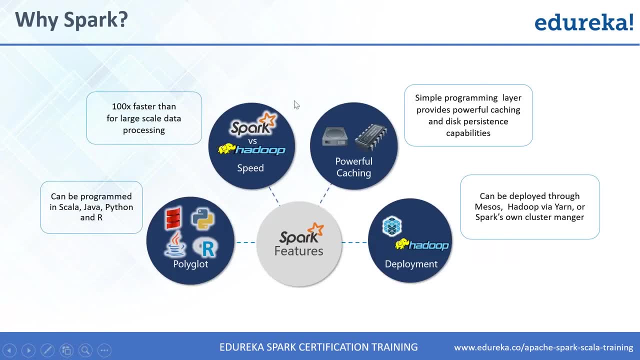 Okay, and it has got the capacity to process real-time data and it is hundred times faster than Hadoop. Okay, 10. Times faster, simple programming, and when it comes to the implementation of business logic, you can do that using Scala, Java, Python and R. 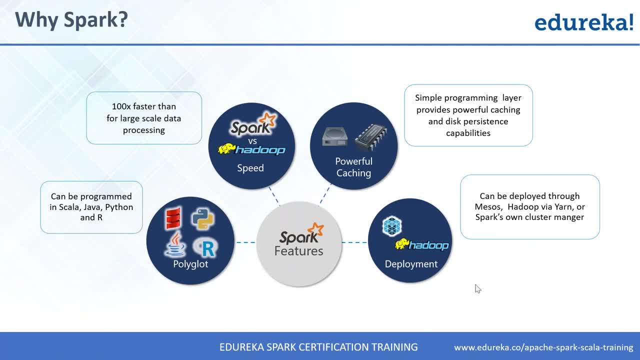 Okay, Scala, Java, Python and R, and then you know it's like. when it comes to the deployment, it can be done using Hadoop as well. Okay, I have a question here. question is: most of the folks using Scala spark, What is the scope in python? 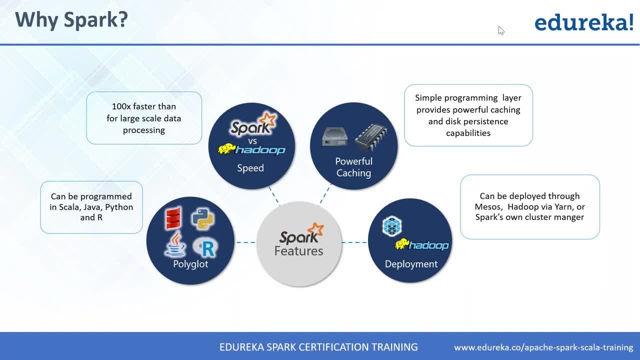 No, no, Ajay Ghosh, It's not that. so, basically, when it comes to, when it comes to spark with python, it's it's called a spy spark. So, guys, the point is, whenever it comes to the statistical analysis, right. so it's like until unless you are completely involved into 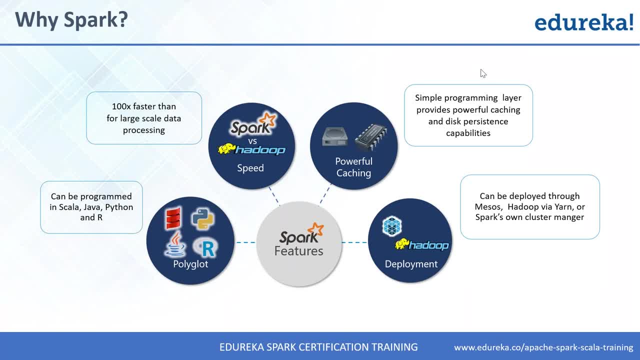 statistical analysis. you will not be using pi spark. Okay, when it comes to machine learning or when it comes to statistical analysis, then we will be going with the python, with spark, Okay. So yeah, yes, using Hadoop through spark. So spark plus HDFS guys. 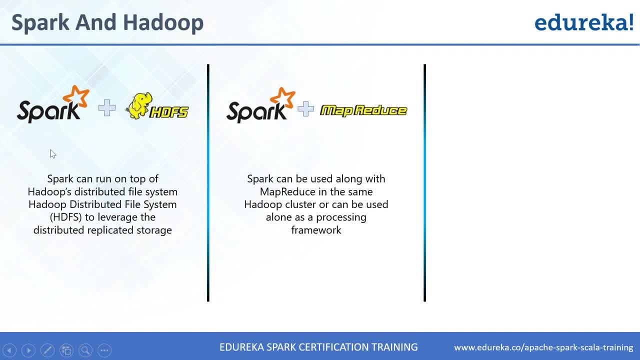 What is HDFS? HDFS is nothing, but it's a storage, So spark can run on top of HDFS. It's like your data data will get distributed by HDFS and for processing, instead of using MapReduce, you can use spark right. 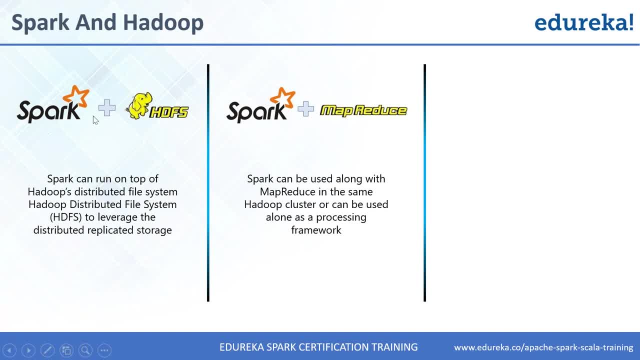 And this question was asked by Vani, like: can we use both at the same time? So the answer is yes, All right, so spark can be used along with MapReduce in the same Hadoop cluster can be used alone as a processing framework, right? 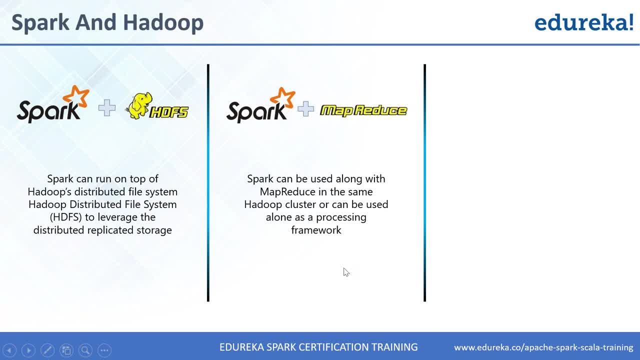 So cluster can be same. There is. there is no need to deploy a different cluster. Okay, Okay, let's move on. Okay, spark and Hadoop. spark is not okay. So, guys, I get this question most of the time, but I think I've already. 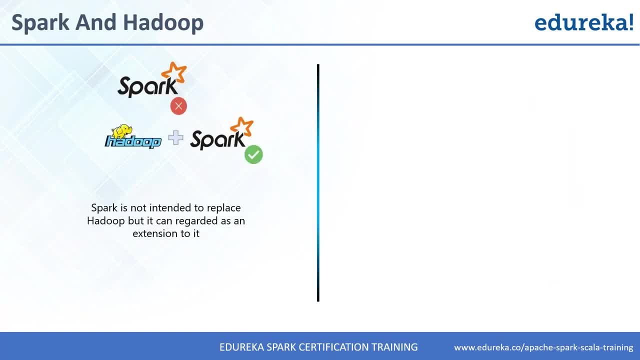 answered this question. the question most of the time from the participants will be: is spark a replacement to Hadoop? No, it's not a replacement, guys. again the same example which I took off Facebook. So, guys, if there is something which can be done by spending less, 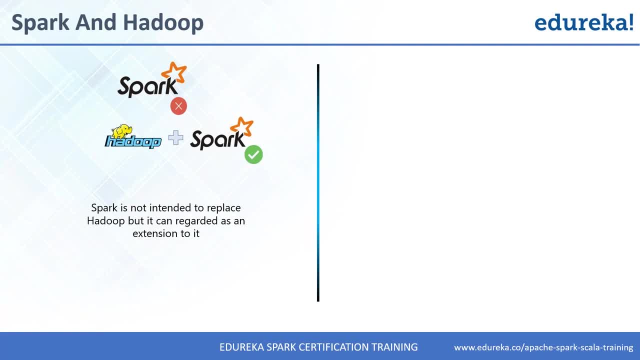 would you be spending more on that? No right, Same thing. Hadoop is less expensive than spark. Why? because Hadoop is doing the you know. basically Hadoop is doing the reading and writing to and from the disk, And when it comes to spark, spark is doing the in-memory processing. 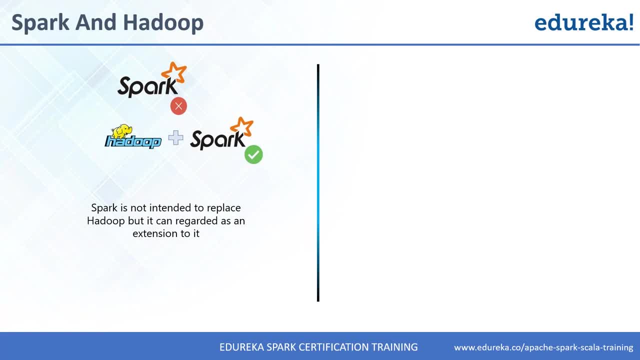 in-memory processing as an. it is expensive, So based on your use case, you will always be choosing. I told you right. when I change the, when I change the organization. I was interviewed on Hadoop and spark both and before joining the new organization. 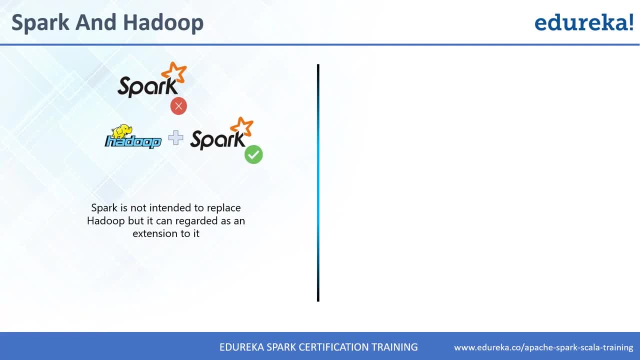 I was working on a spark project when I joined the organization. I was told that I'll be working on Hadoop right, and I was. I was curious to know the use case. And then they explain the use case and I was convinced that, yes, there. 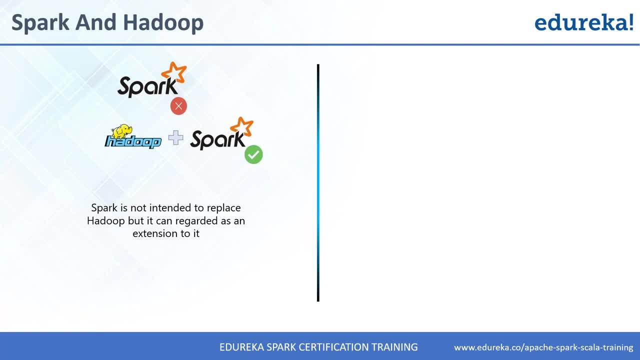 is no need to use spark, right? It's not that that spark is a replacement of Hadoop. No, it will always depend on your use case and on the need. Okay, Okay, Okay. so yeah, let's move on. 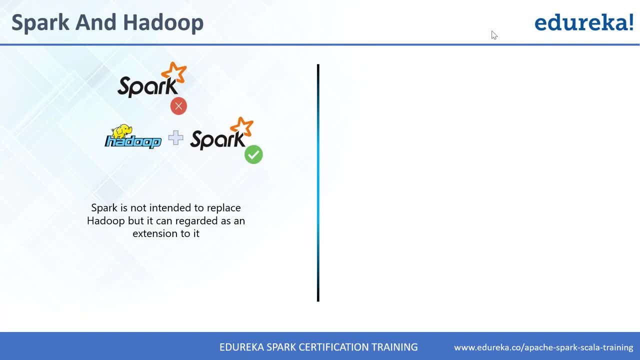 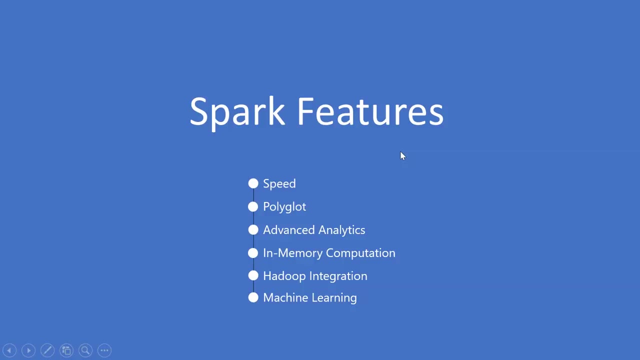 Okay, so MapReduce and spark are used together, where MapReduce is used for batch processing and spark is used for real-time processing. Okay, so what are the sparks feature guys? So it's speed. It is hundred times faster than Hadoop, and when it comes to the 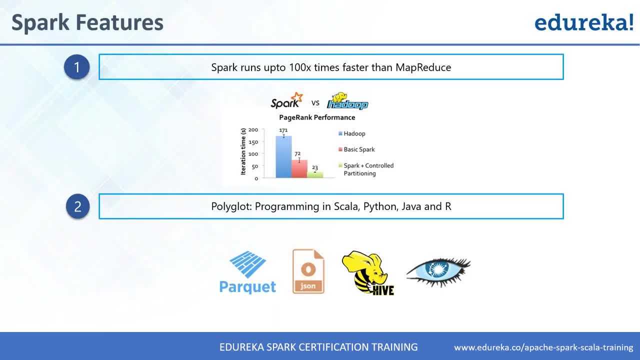 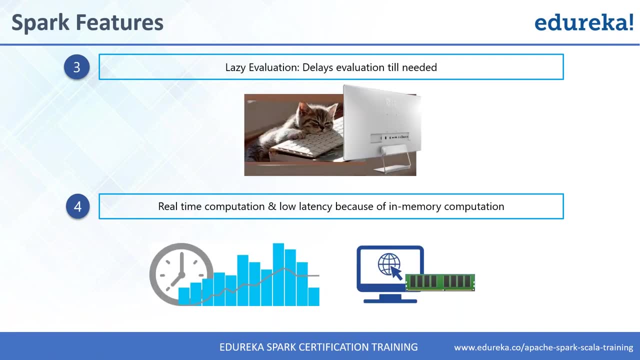 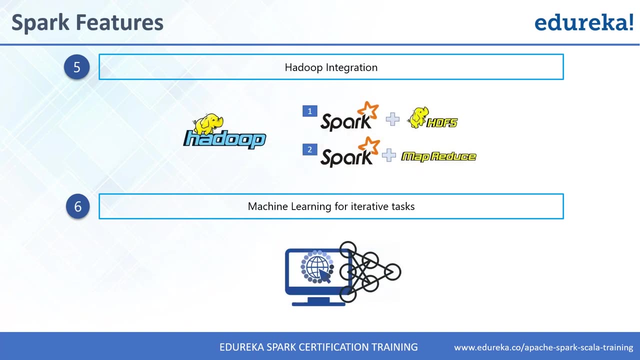 implementation of business logic. it can be done using Scala, Python, Java and R and it can have different different file formats. Okay, it does the lazy evolution, real-time computation Okay, and integration of Hadoop is possible, and also it has got modules. 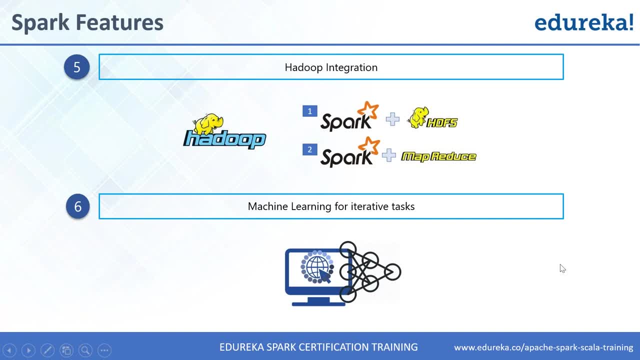 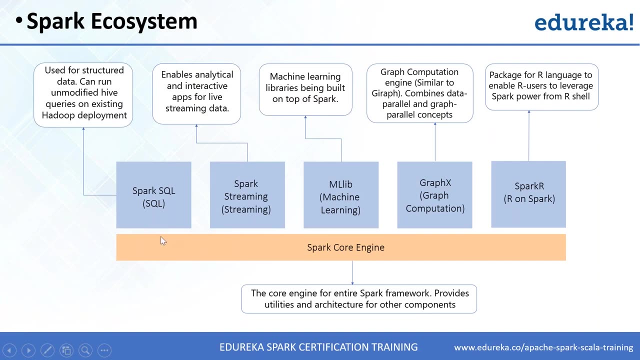 using which you can implement the machine learning algorithms, as in, you can have the iterative tasks. Okay, so, when it comes to the spark ecosystem, guys, so what do we have? We do have a core engine and then we do have spark sequel. So, using this module, you can write the sequel like queries and 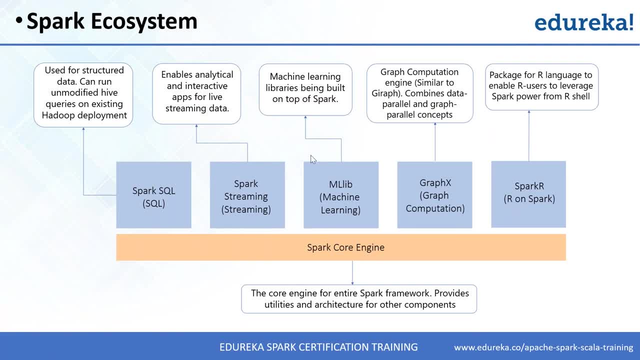 then you can also do some other things using this module. Okay, so how do you need to do that? I have a question from Shrikumar. Shrikumar says when you say Hadoop, it refers to MapReduce. No, when you say Hadoop, it refers to HDFS plus MapReduce. 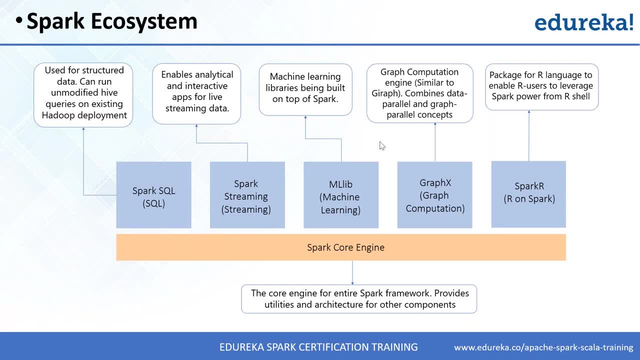 Okay, Okay then. so, guys, when we talk about spark ecosystem, right. so when, When it comes to the spark ecosystem, we can use Spark ecosystem to the code, spark, right, you can implement the business logic using python scalar art, but if you don't come from programming background, if you do not come from a programming background, 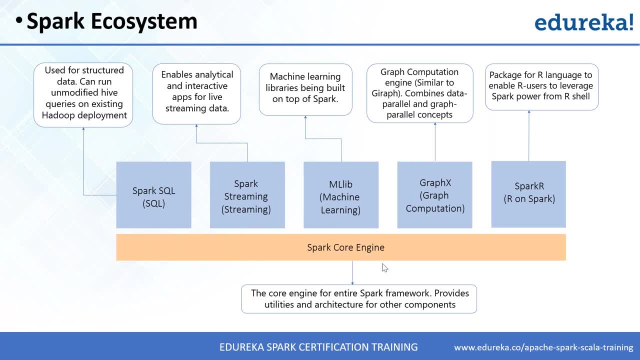 and you say that, and you say that: hey, you are interested in writing sql queries. right then, we do have a module using which you can write the sql queries. then we do have spark streaming, using which you'll be processing real-time data. then we have for machine learning, using which 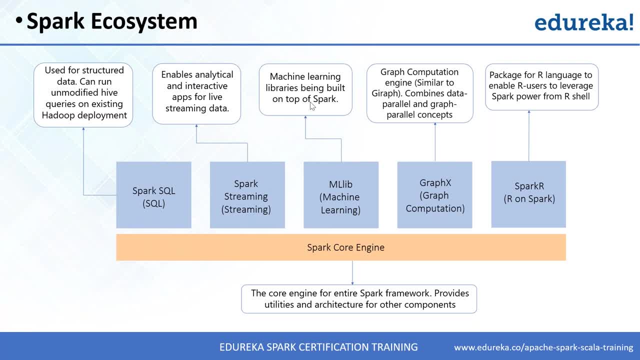 you can implement the machine learning algorithm. if you have the need to do the analysis on graph data, you can do that. right, so these are the things which you can do, okay, so, guys, so the point is, uh, right, so the point is, it's like: now, you see, one installation of spark can serve. 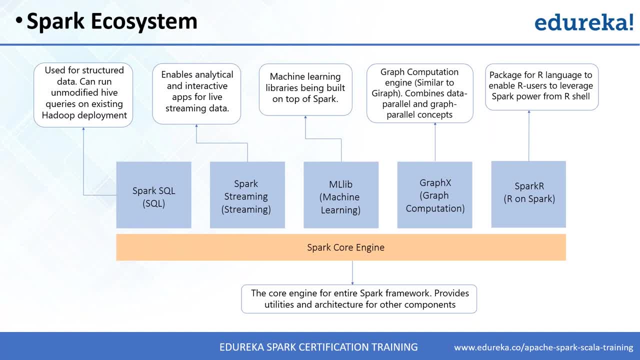 these five purposes right. so if you do not use spark, then for doing for sparks seek for for are implementing the sql queries, you might have to download different tool or a component. then for real-time analytics you might use tom, for machine learning you might use mahat, then for graphics you might use neo4j. so the point is because 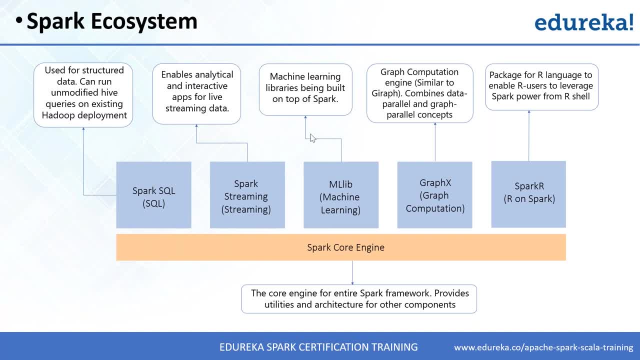 spark is providing n number of features, right, so that's why you know we say that it is being used widely. but again, the use case can be different. so whenever someone says that they are working on spark, be confident on on raising this question where you say that, okay, hey, which? 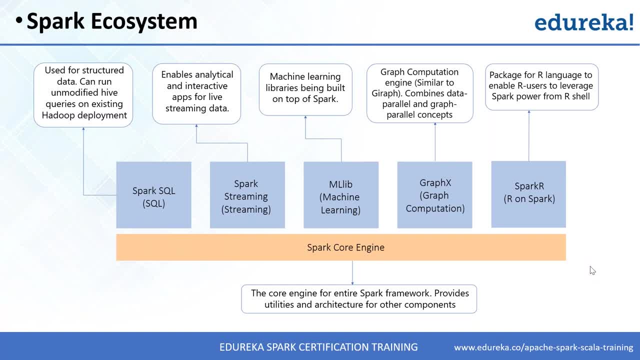 module of spark you're using. are you working on mlib or you are working on spark streaming? so yeah, okay. so yeah, spark core. so, basically, as part of what, what course we have for spark and spark code? you will understand how it does the distribution in memory. okay, what? 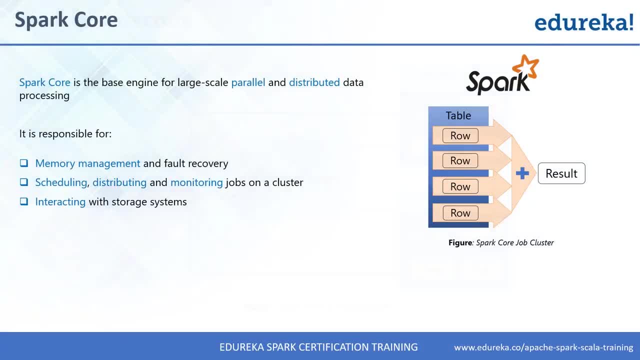 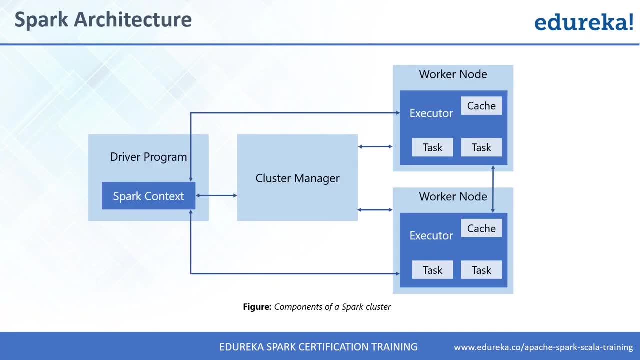 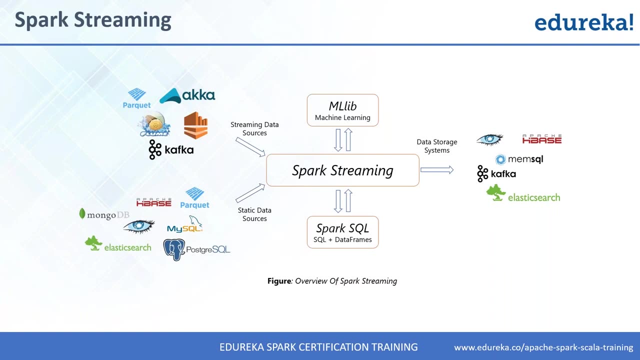 if something goes wrong, how? how it recovers the data in the memory, right. and then it comes to the spark streaming. you will understand that how it deals with the real-time data and when we talk about spark streaming, we talk about kafka. so basically, spark says that, hey, my job is to process the real-time data, my job is not to go and collect. 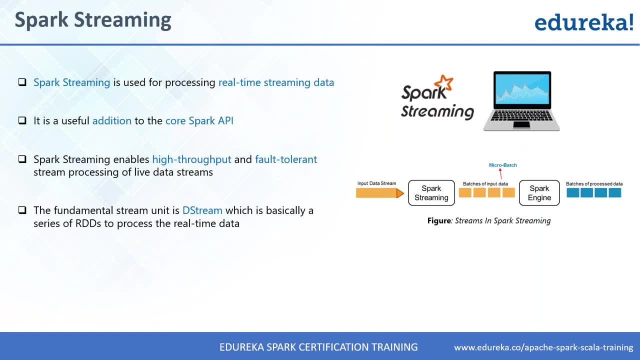 the data from somewhere. so now we need someone who will go and collect the data for us. so what do we have? we do have kafka. so kafka is nothing, but it is a messaging queue which we use to collect the data. so, on one hand, we will be connecting kafka. on one hand, we will be connecting. 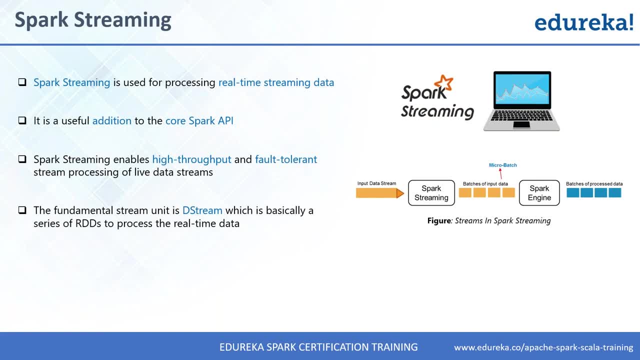 kafka to a streaming source, let's say twitter to a fitbit, and then, on the other hand, we will be connecting it to spark, right? so basically, kafka, as a messaging queue, will collect the real-time data and it will feed it to spark. okay, so, yeah, this is what spark streaming is. right, then spark sql. so 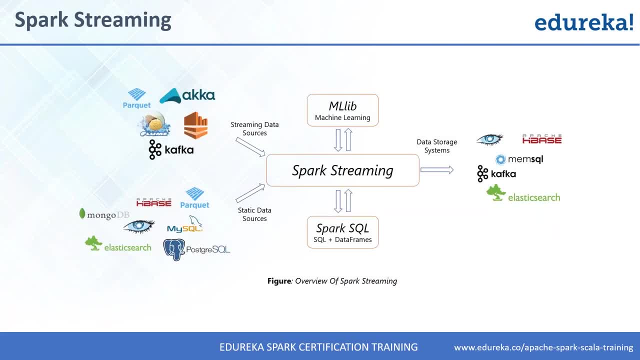 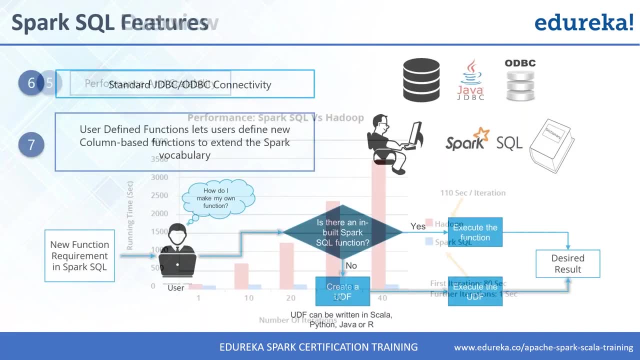 it's like you can write the sql like queries for implementation of the business logic. you can always do that. so let's move on. ravi says how many kafka sources can be connected to one spark stream. so kafka itself is a distributed system. ravi, kafka itself is a distributed system. 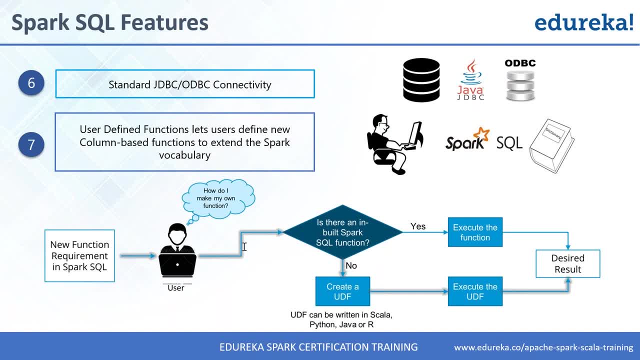 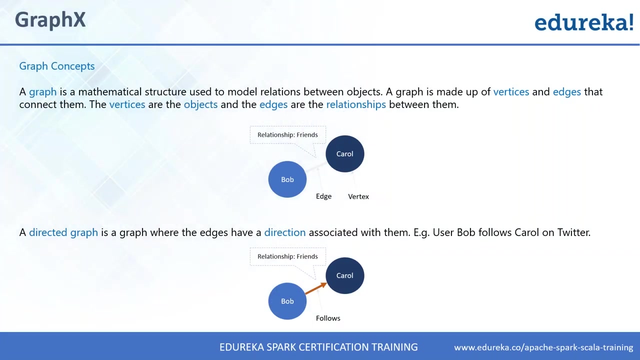 okay, okay, so let's move on, okay. so, yeah, then we do have a component using which you can implement the machine learning algorithms. then graphics: it's like you, on facebook we have friends, friends of friends, and if you are interested in doing the analysis on that kind of data, then we will be using graphics, okay. 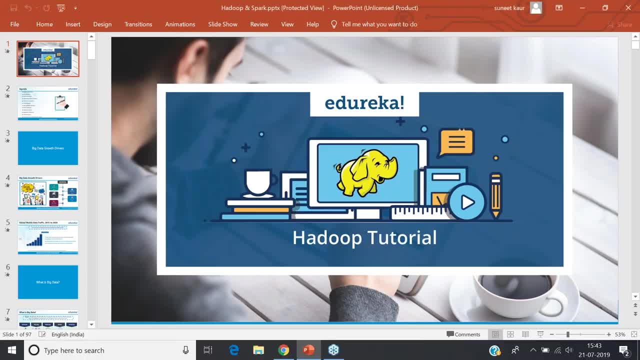 so, yeah, guys, um, what is spark streaming? spark streaming is nothing but uh, it's a module using which we will be doing the analysis on live streaming. so we will be doing the analysis on live data. so it's printed on live data. so what is this module? so, basically, this module has got n number of- uh, you know, functions. 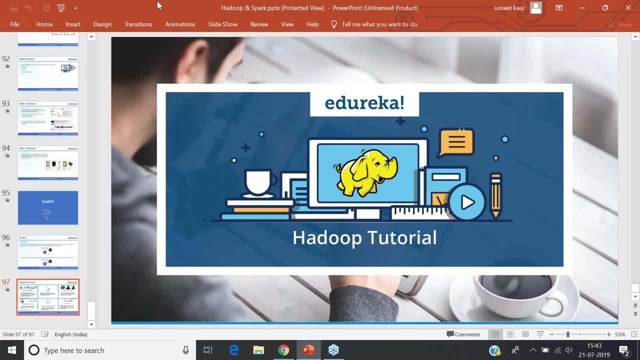 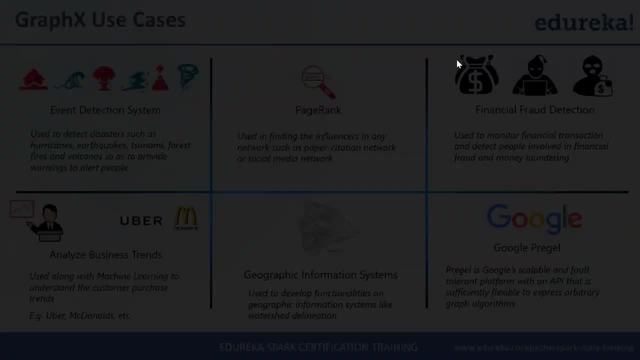 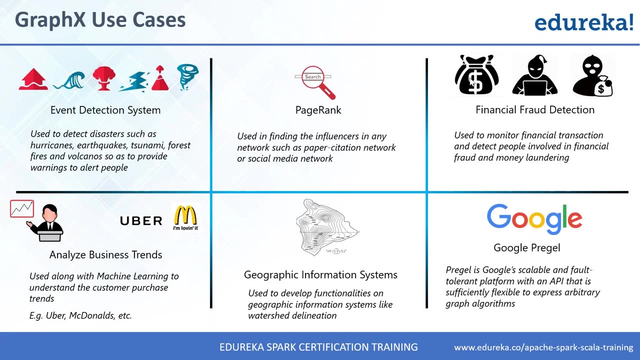 this module has got n number of functions and those functions will help you in doing the analysis or real-time beta, so you don't need to write uh code for processing real-time of data. okay, stream values are different. extreme values yeah. multiple uh kafka sources can be connected to sprint streams. they're actually taste good stresses. 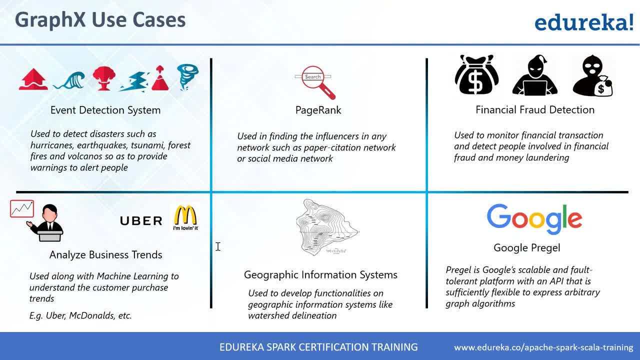 connected to spark, in that case ravi, okay. so yeah, guys, uh, this was all about the overview of hadoop and spark. so quickly to summarize, when it comes to spark, we do have spark core, in which we will be implementing the business logic using scala, python or r. we can use java as well, and 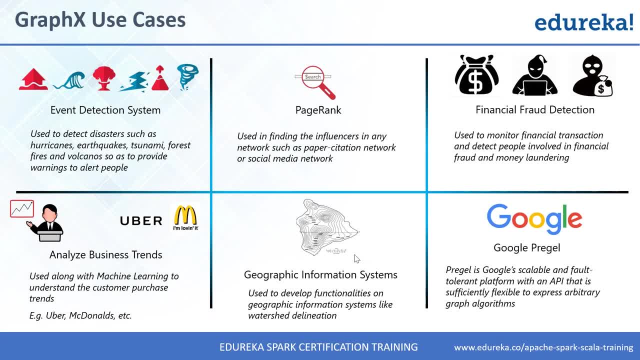 then it has got modules like: there is one module which we using, which we can implement the sql like queries. then there is this module module, as in, it has specific functions like, like, related to sql. then we say when, when we say spark mlb, as in, it has functions using which you will be implement. 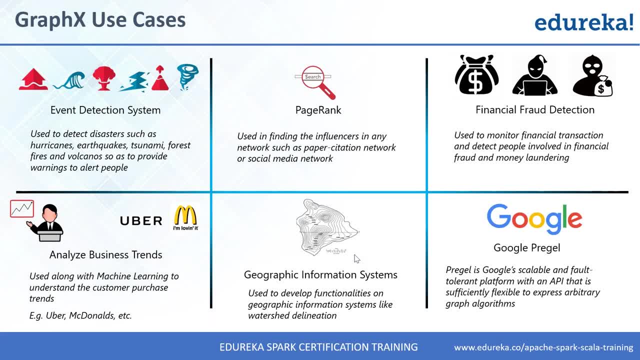 you will be able to implement machine learning algorithms easily. okay, then we say that. okay, we have, you know, uh, spark streaming, using which we'll be able to do the analysis or real-time data easily. what are popular ids? uh, we are using eclipse and uh, intellij. yes,